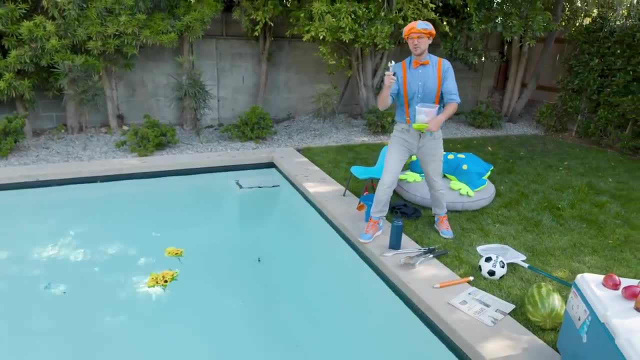 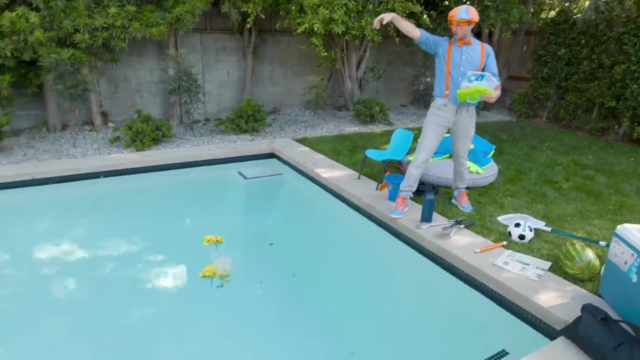 It floats. Oh, I bet you know what these are gonna do. Yeah, the tools, The tools, The tools, The screwdriver and the pliers. Yep, They went all the way down to the bottom. That means they sink. 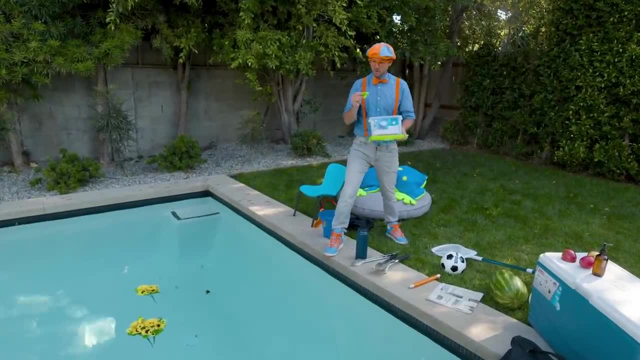 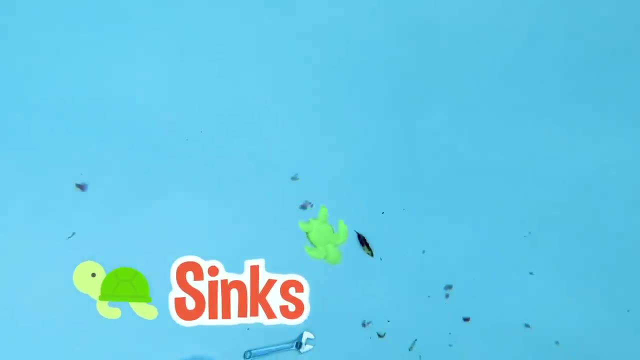 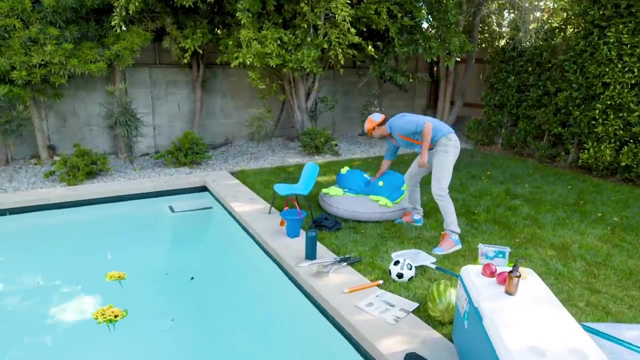 Oh, let's see, Let's take some of these toys. Oh, a little turtle, Whee. Oh, That one sinks as well. Buh-bye Whoa, Look at all these other things. Alright, Let's put this pool toy in here. 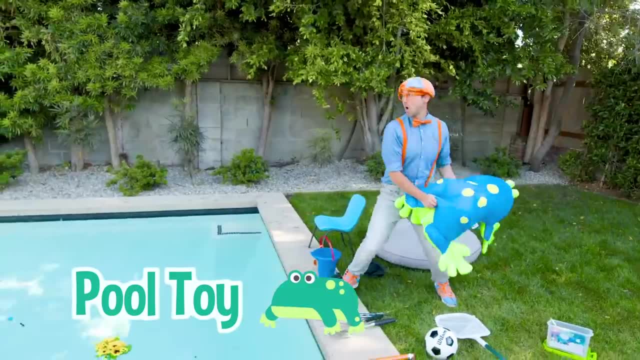 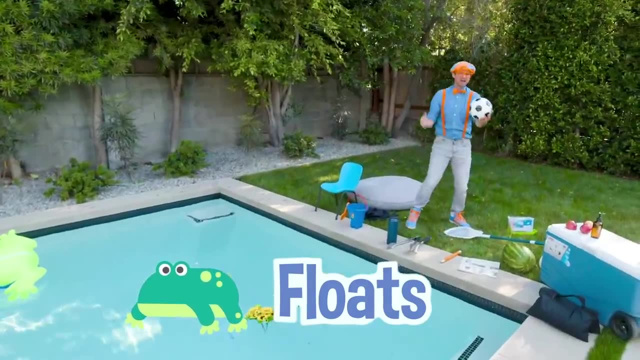 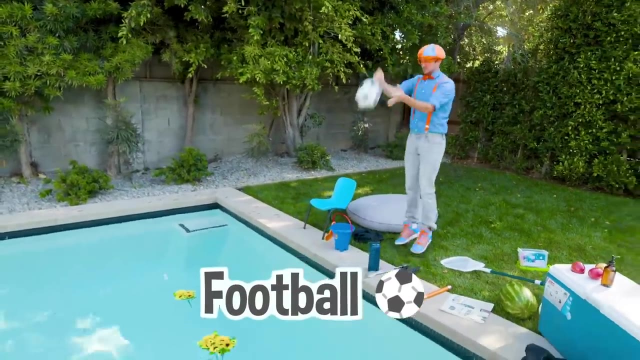 Let's put this pool toy in here. Let's put this pool toy in there. Woohoo, Yeah, It floats. Whoa, Check it out. A soccer ball. Some countries call this a football Ready. Whoa, It floats as well. 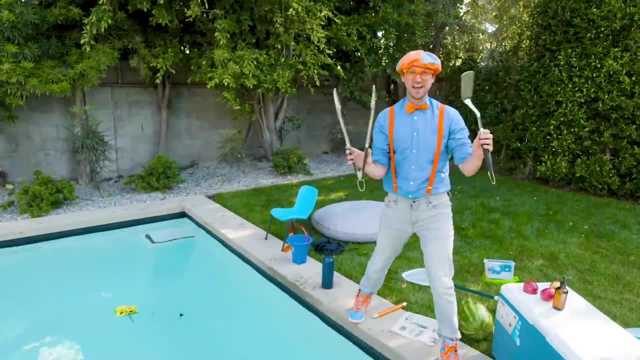 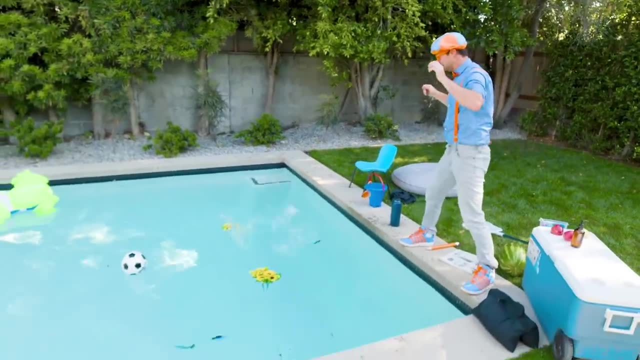 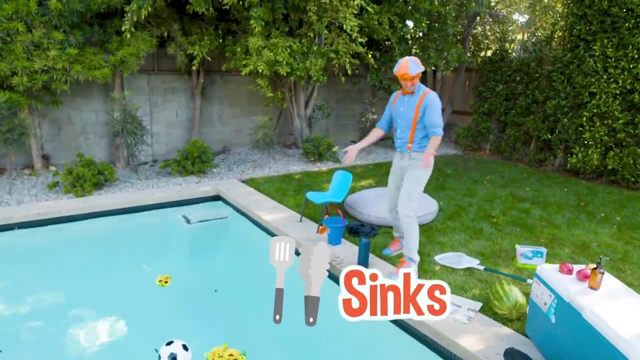 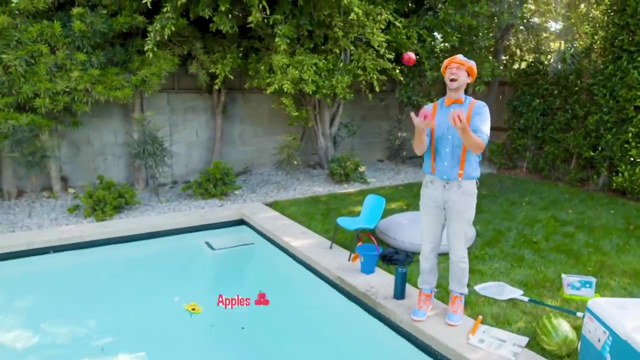 Whoa Yep, Barbecue tools, BBQ, Here we go. Where'd they go? Oh, they went all the way down to the bottom. That means they sink. Hey, Look Some apples. Check this out, Whee. 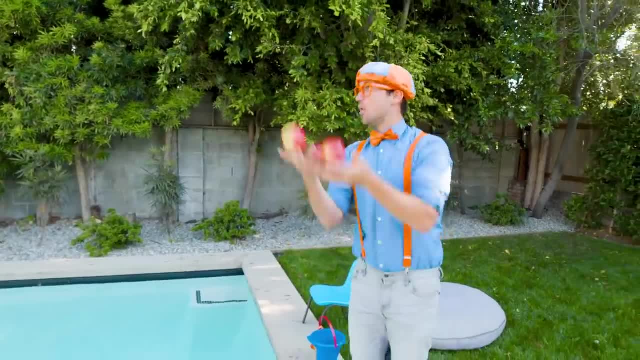 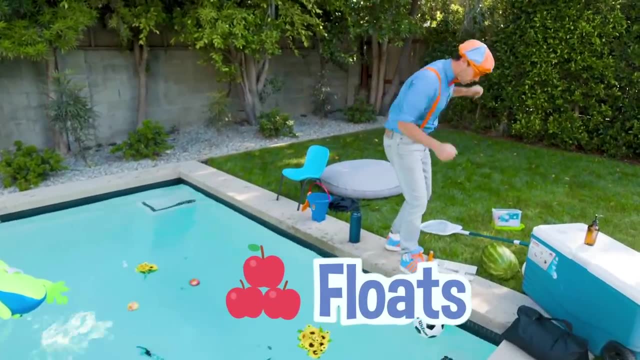 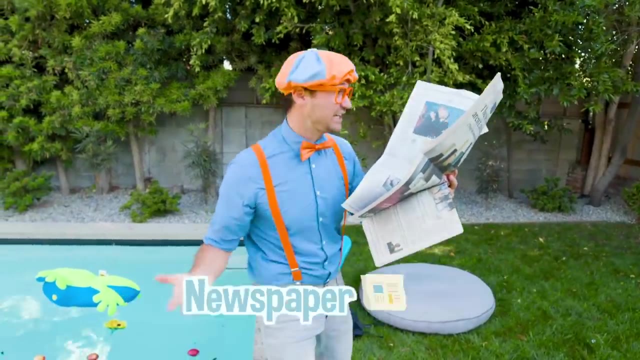 Whoa. I wonder if these apples will sink or float. Woohoo, Hey, All three of them float. Whoa, I love reading, Especially newspapers. They're so exciting. That's what my grandparents would say. That's what my grandparents would say. 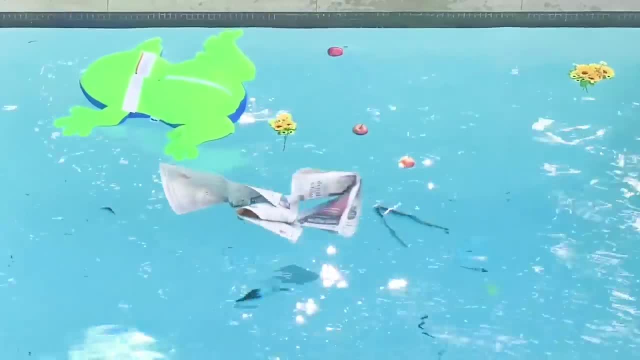 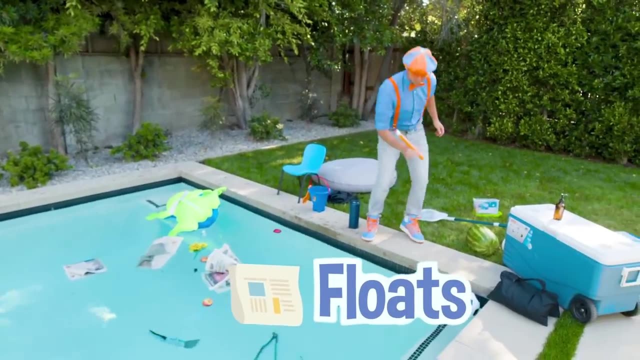 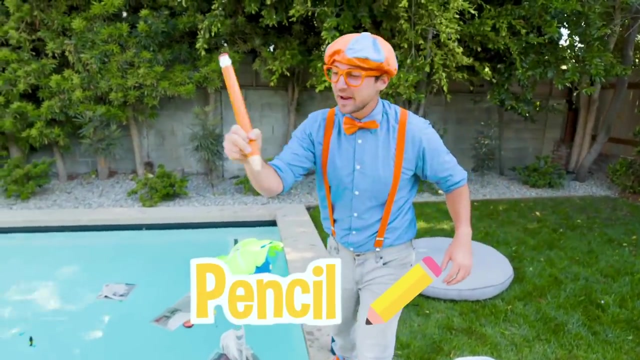 Alright, here we go. Alright, here we go. Hey, Look Those newspapers float. Look Those newspapers float. Hey, Someone had to write all those words on the newspaper. Someone had to write all those words on the newspaper, And they might have started with a pencil on paper. 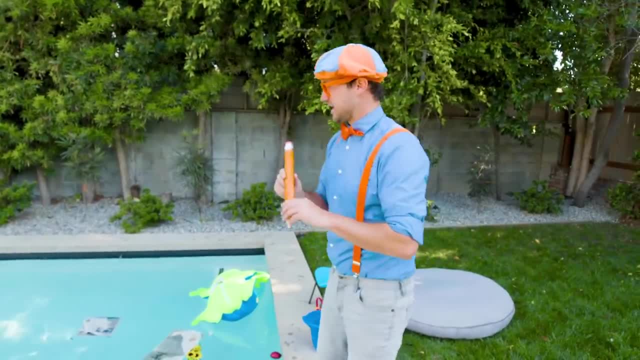 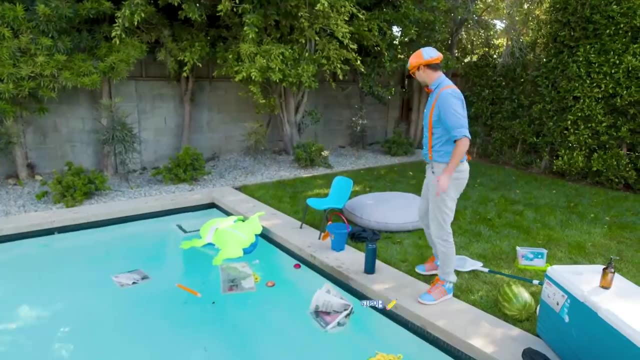 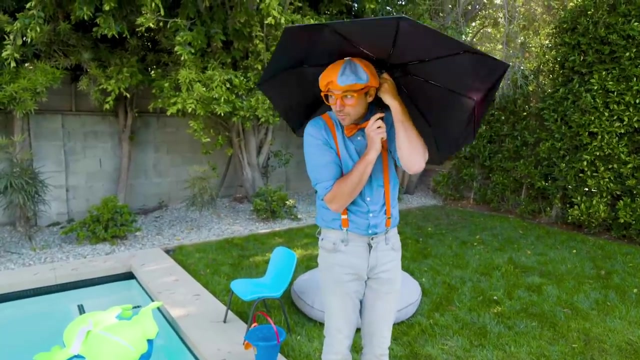 Yeah, It's a pencil. Here we go. Hey, It floats, That giant pencil floats. Do you know what this is? Do you know what this is? It shields me from the rain, Keeps me nice and dry. It's an umbrella. 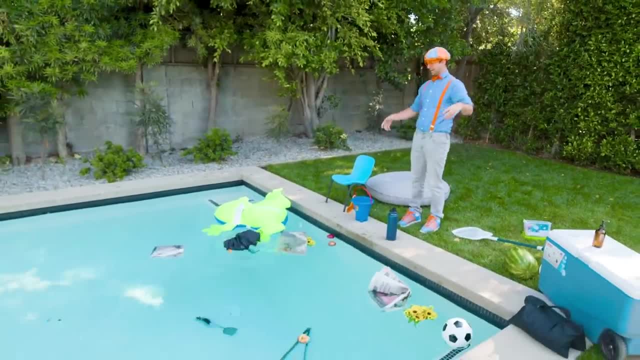 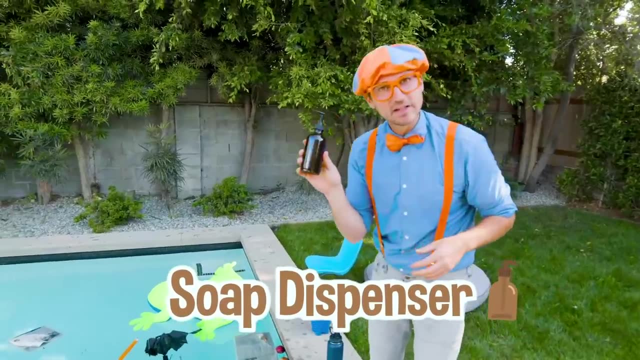 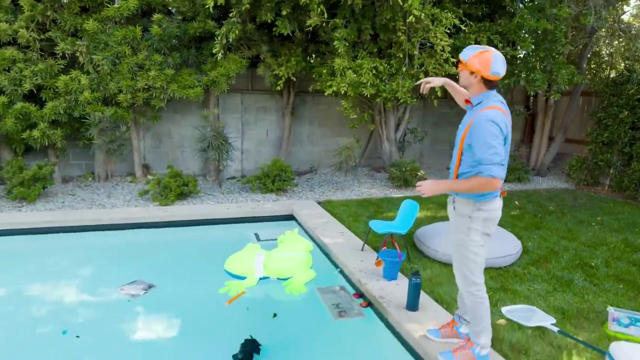 Here we go. Hey, That floats too. Whoa, Yeah, A soap dispenser. I love washing my hands, Do you? Alright, here we go. Alright, here we go. Whoa, Where'd it go? It went down to the bottom. 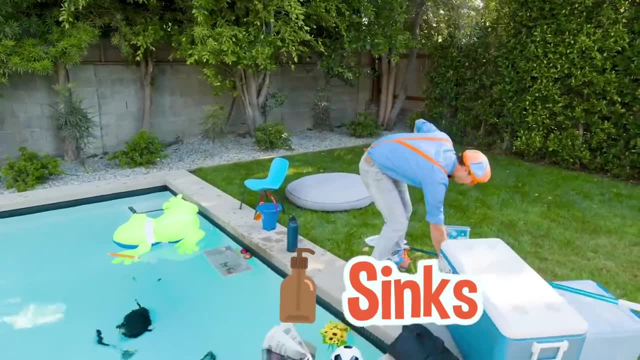 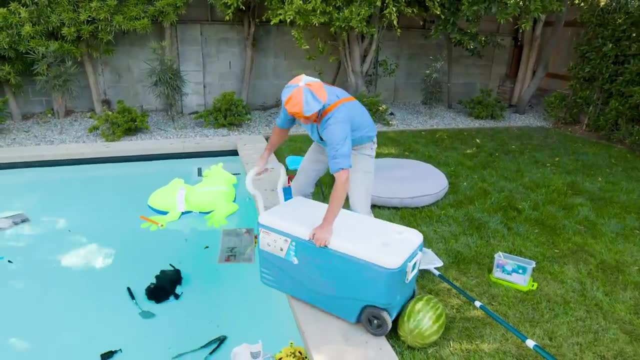 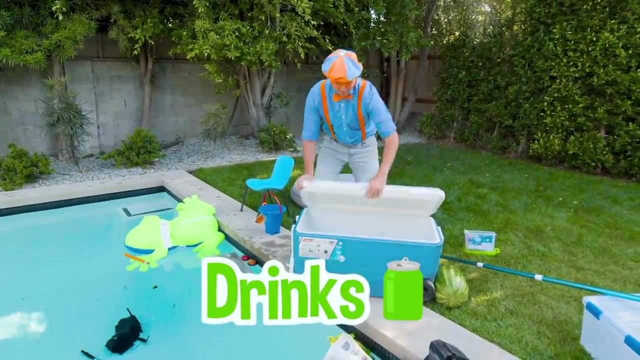 That must mean it sinks. Whoa, Have you ever used one of these things before? Have you ever used one of these things before? This is a. This is a A cooler. You typically put a lot of ice and drinks in here. 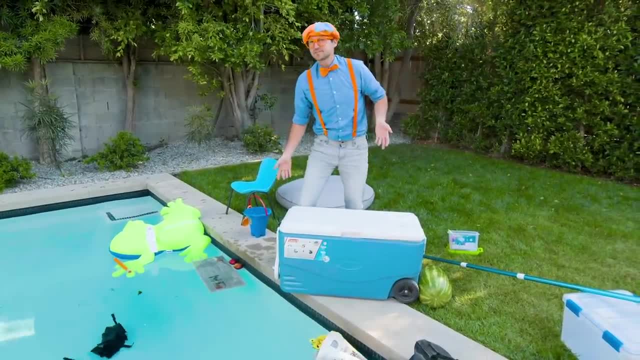 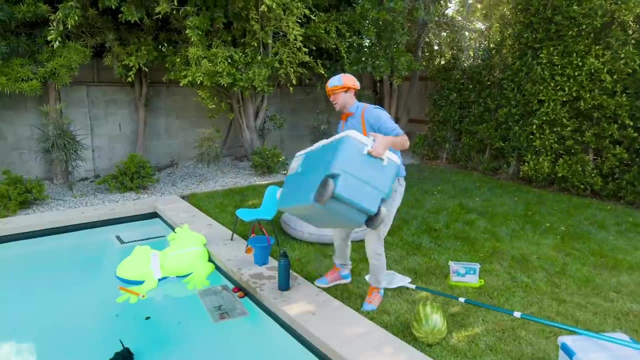 But for now it's really empty. But for now it's really empty, So that must mean it's probably really buoyant and not very dense. So I bet you you know if this will sink or float. Argh, Whoa, Look at it. 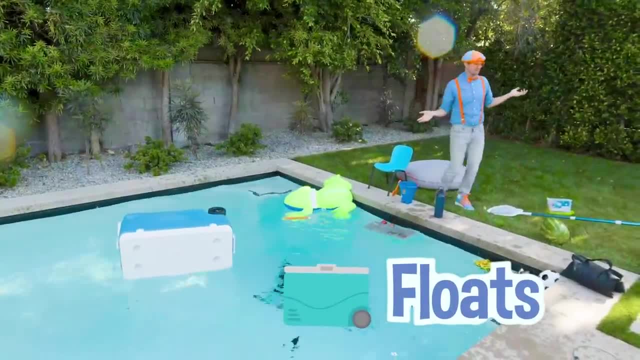 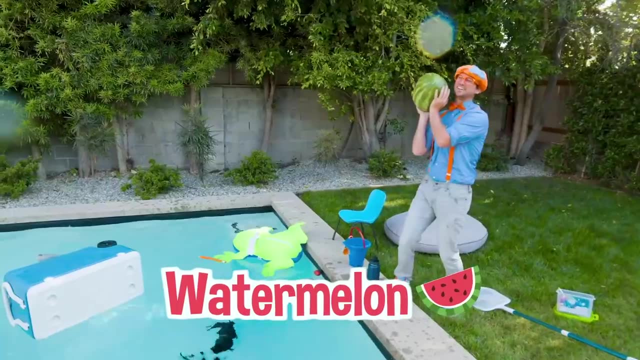 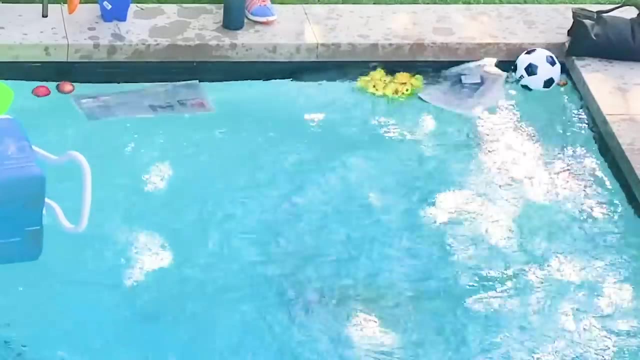 It floats, Yeah, So that means it's less buoyant than water. Alright, Here we go, Here goes the water. Here we go, Here goes the water. Three, Two, One, Whoa, Oh, Oh, It broke apart. 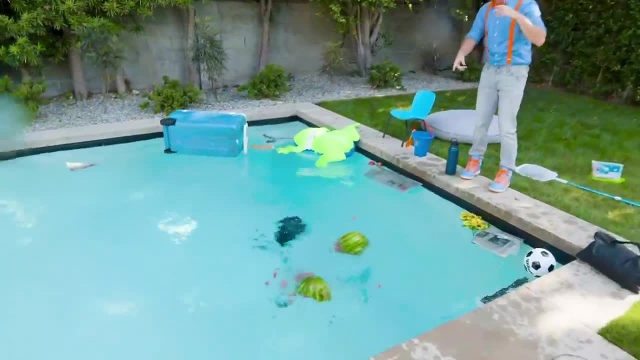 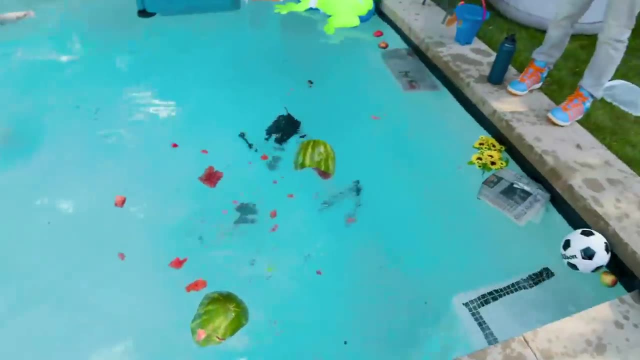 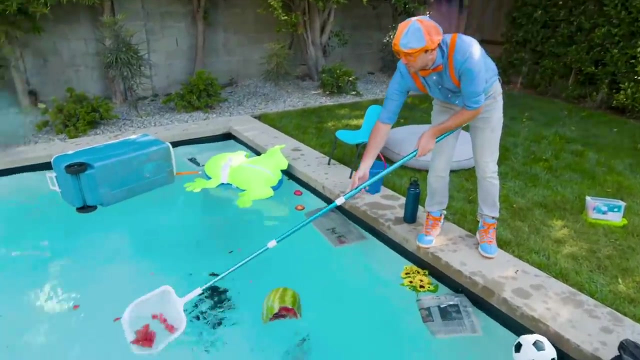 Oh, no, Oh, But it floats. Oh, that's so silly. Oh, I'm gonna have to clean that up. I'm gonna have to clean that up. Okay, let's take this and scoop some of that out. Yeah, Look at that. 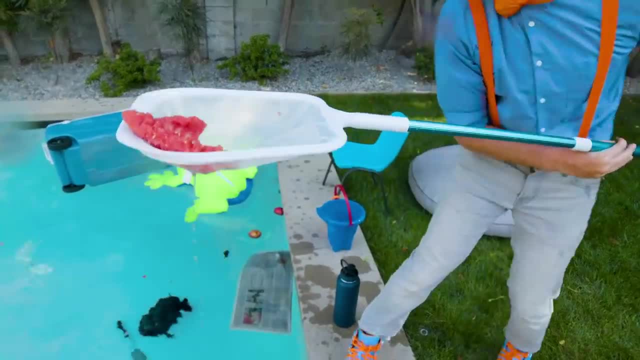 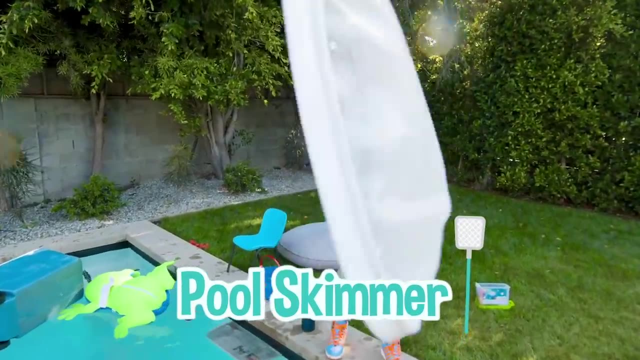 Some watermelon chunks. That looks yummy. Okay, let's put it right over here. Hey, wait a second. Did you see me use this pool skimmer? Yeah, This is what you use to scoop things out of the water. Yeah, like these apples over here. 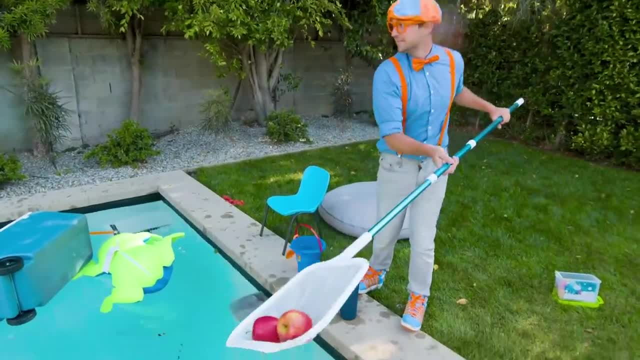 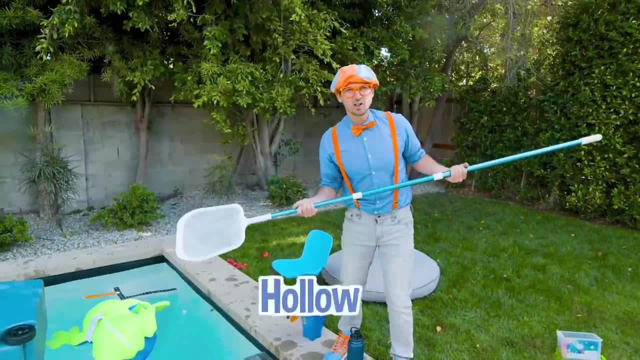 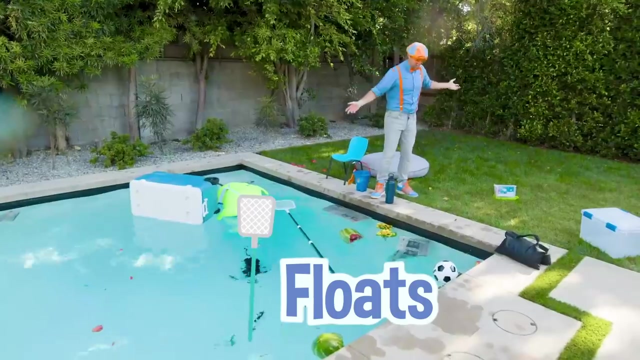 Yeah, remember those from earlier. Let's put those aside. Hey, I wonder if this floats or sinks. It's pretty light. I think it's hollow inside. Let's see. Yep, It definitely floats. There's a lot of other cool things around here. 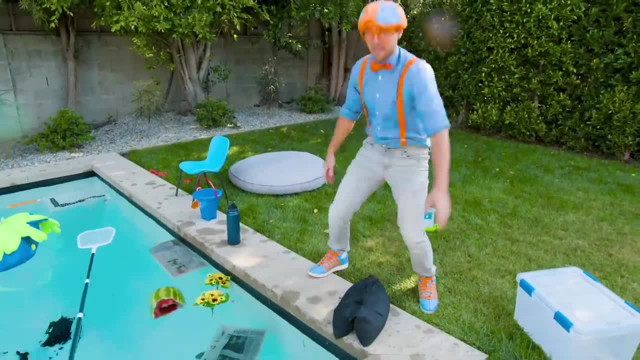 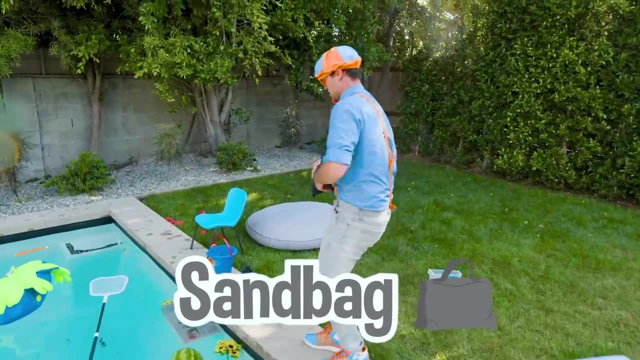 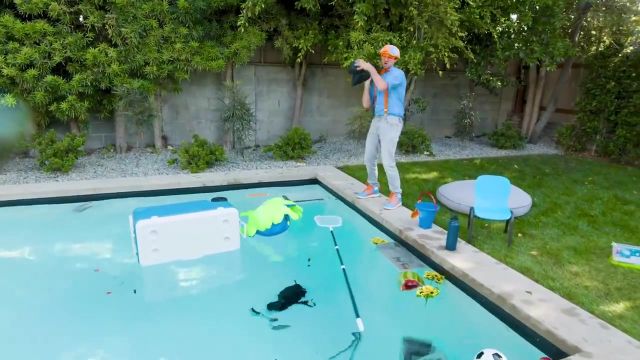 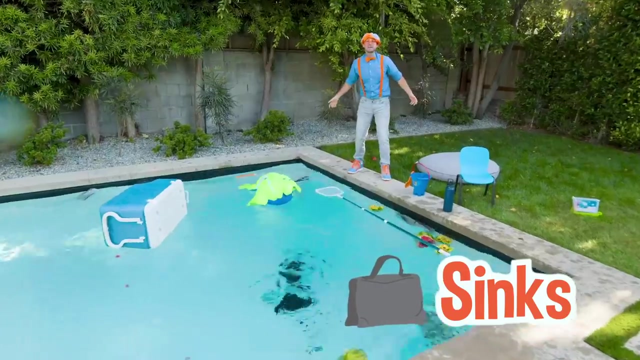 So let's use Whoa. That is heavy. This is a bag full of sand. Okay, I'm gonna go over here. Here we go. I bet this is gonna sink. Whoa, That made a big splash, Wow. 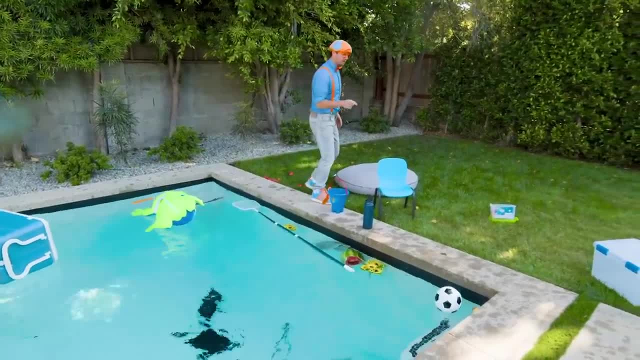 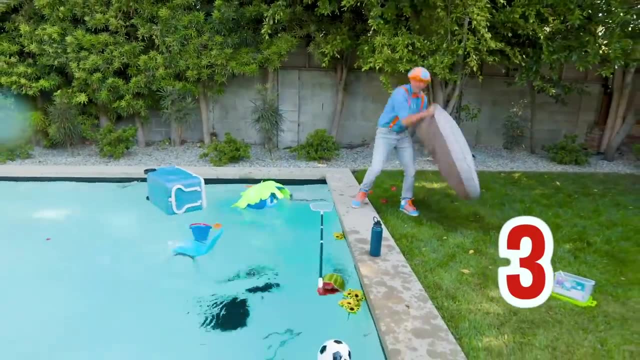 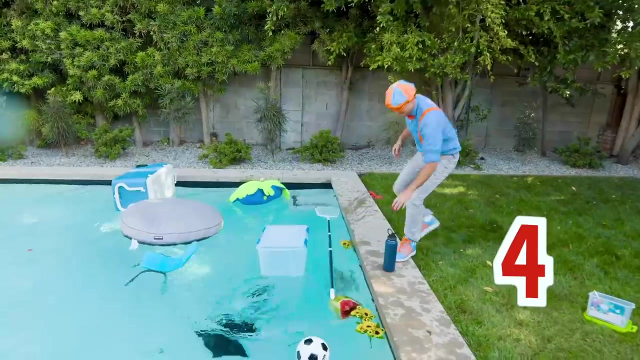 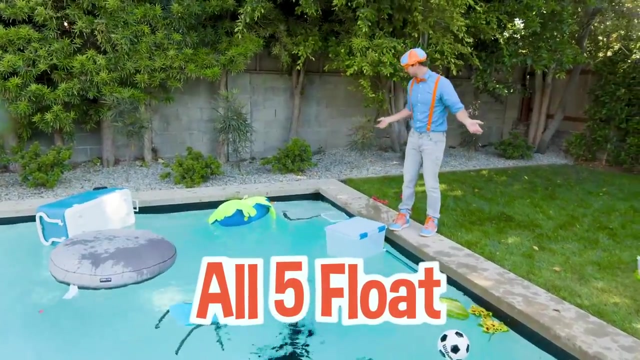 There's one, two, three, four, five more things. Let's throw them in. One, two, three, four and five. All five of these things looks like they float. Huh, There's not much else. Wait a second. 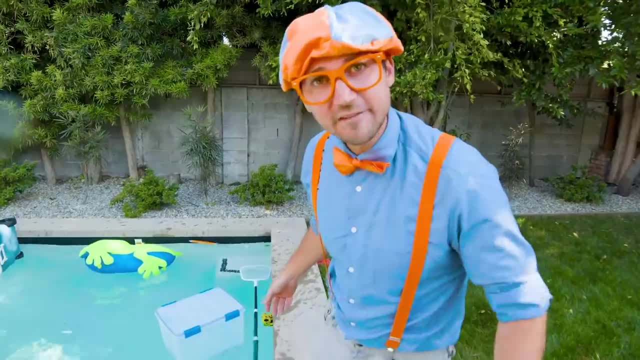 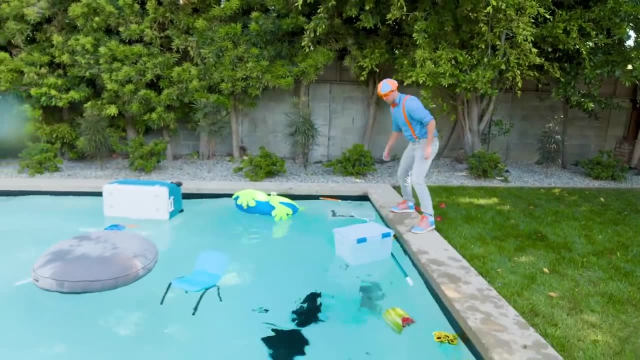 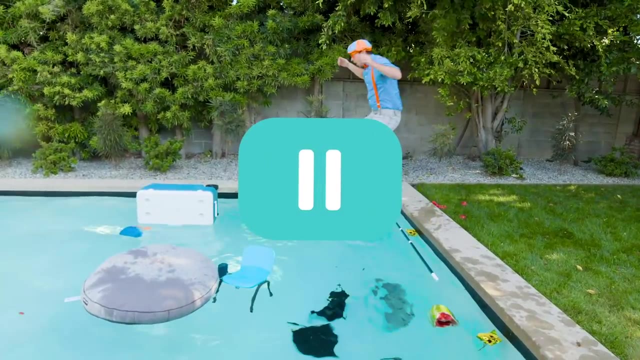 I have an idea. I wonder if I would sink or float. I'm so excited. Let's find out. Ready, Three, two, one, Whoa. Stop right there. Hey, remember you should never jump into a pool, unless a grown-up. 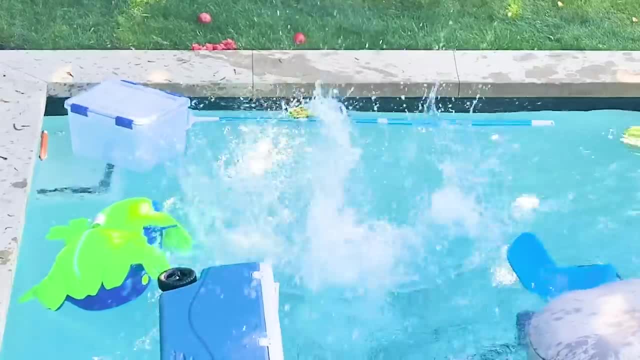 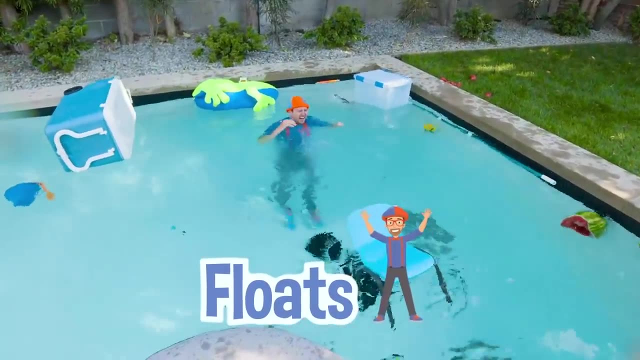 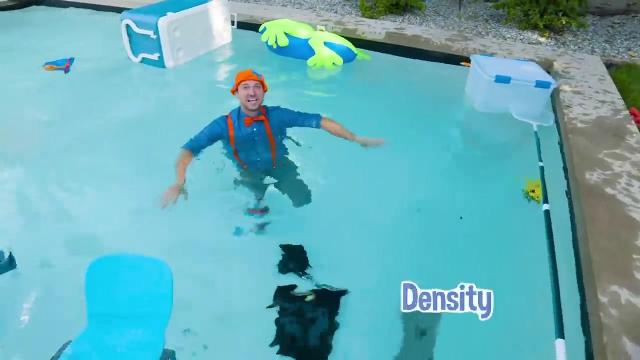 is with you. All right, Here we go. I guess I float. That's so silly. Well, that was so much fun learning about buoyancy with you and density to see what sink and what floats. All right, I guess I'll go for. 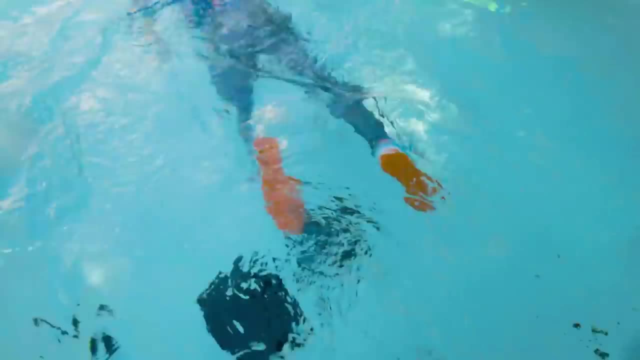 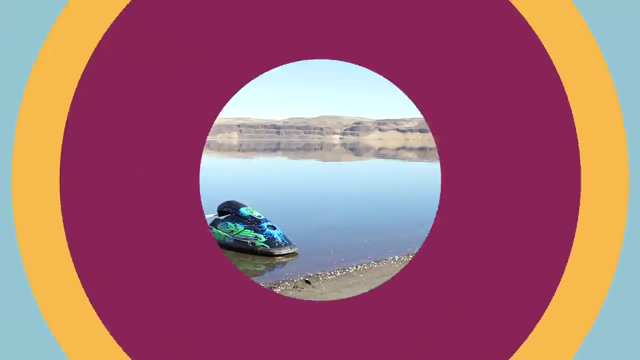 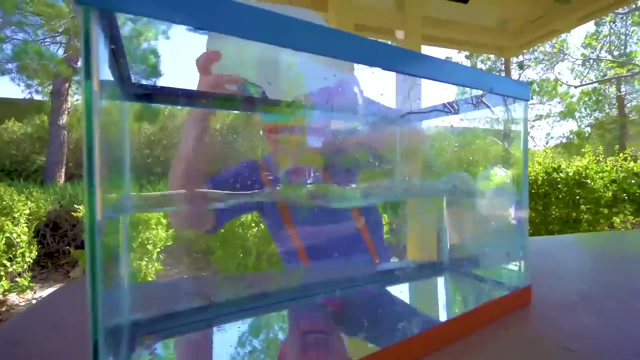 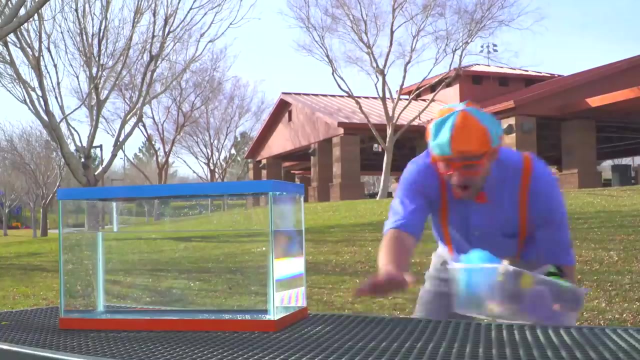 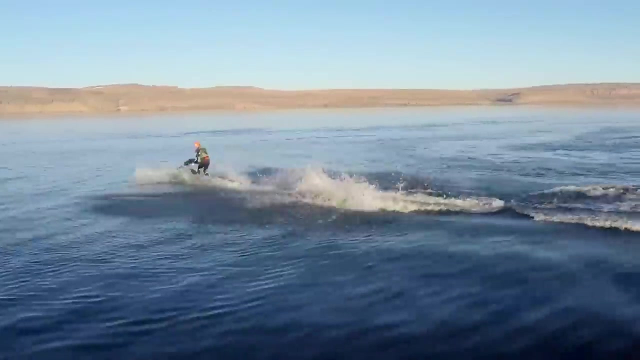 a swim. See you later. Time for an adventure. What games are we playing today? Let's splash in the water. We can play together all day. Let's go grab our toys. Will this one sink or will it float? Maybe jump on my. 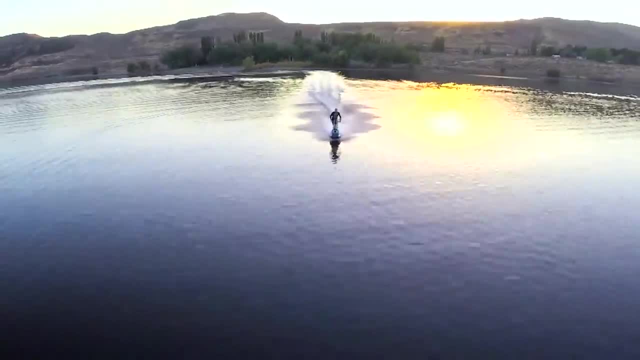 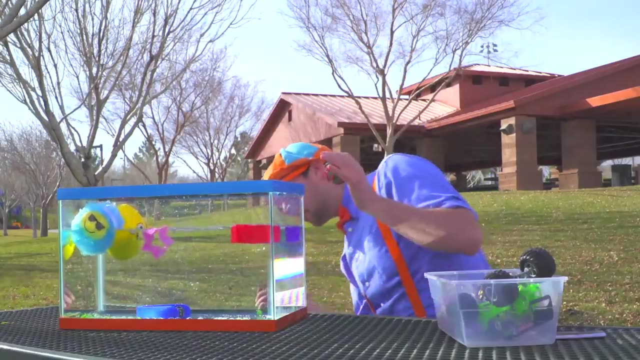 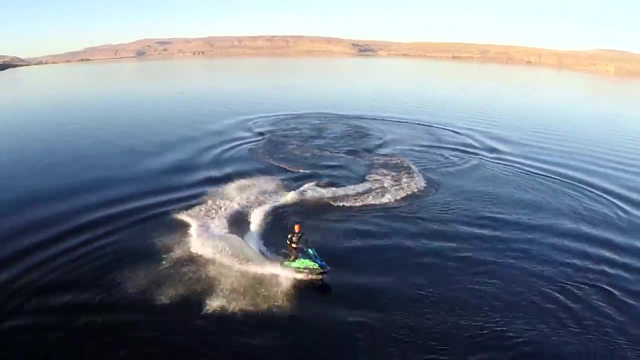 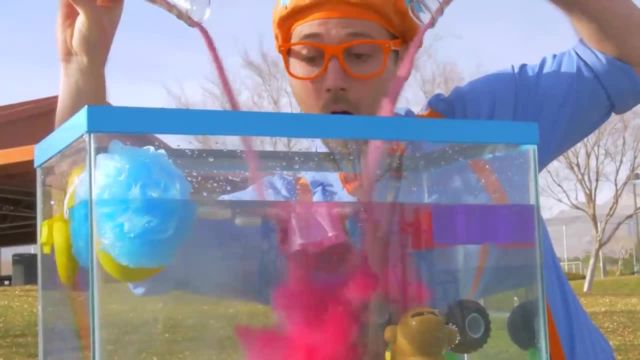 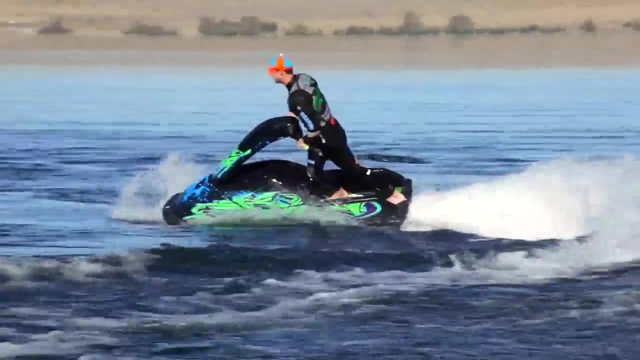 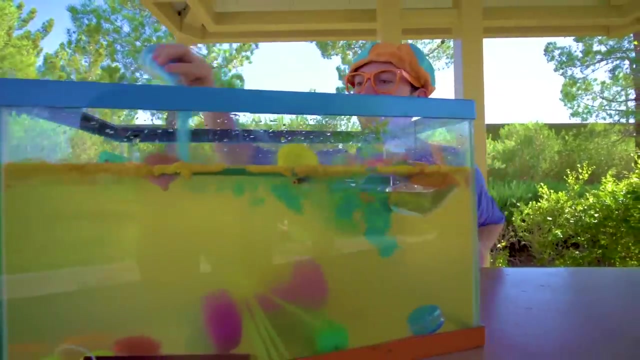 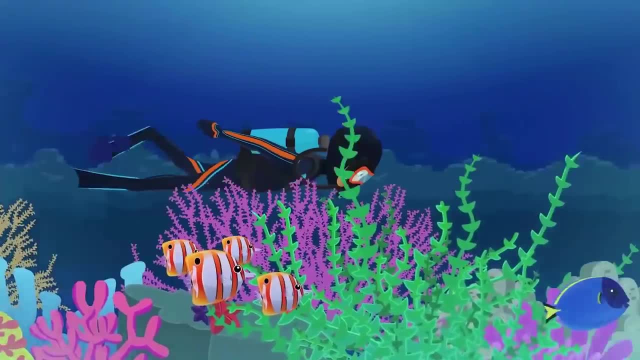 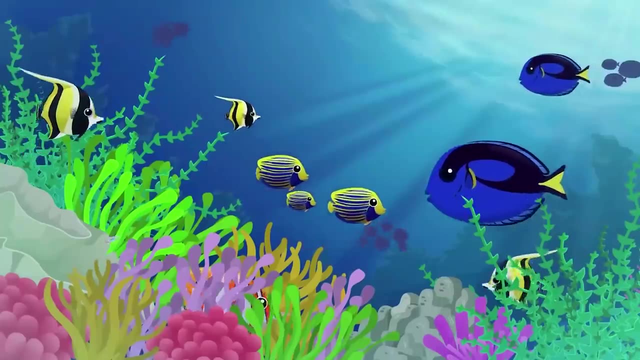 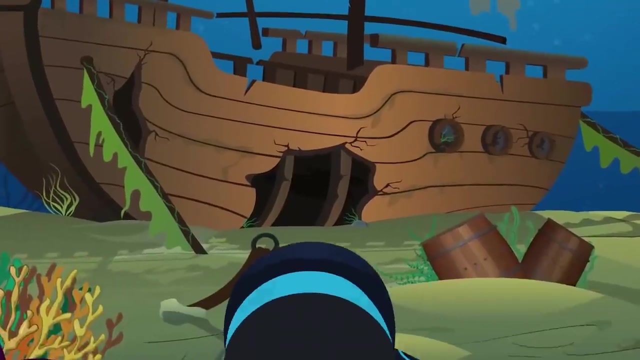 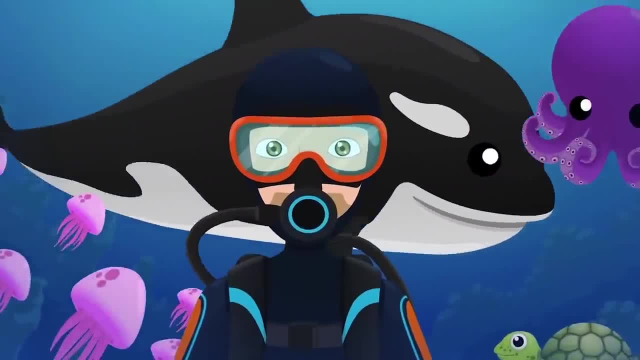 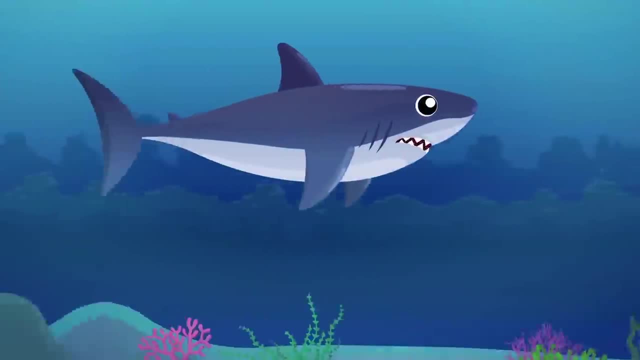 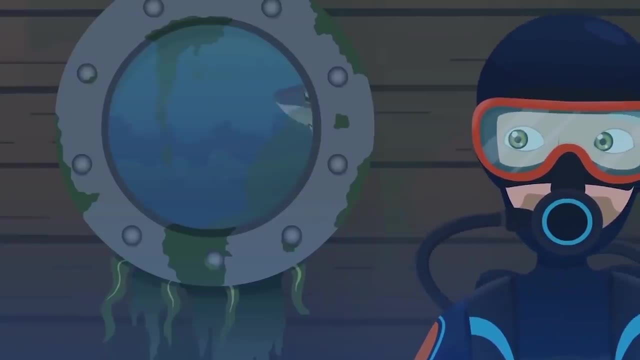 Splish splash underwater, Playing with the fishes. Yes, it's time to play. Splish splash underwater. It's the Blippi way to learn and play all day. Splish splash underwater, Playing with the fishes. Yes, it's time to play. 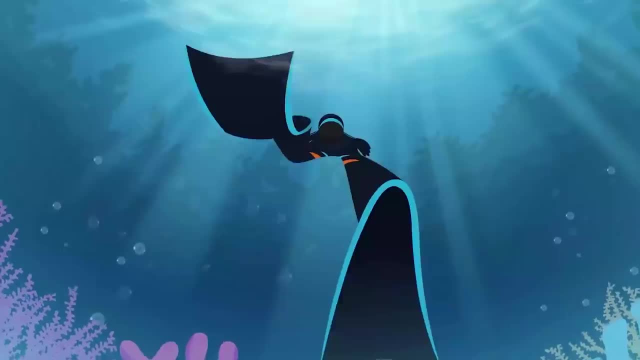 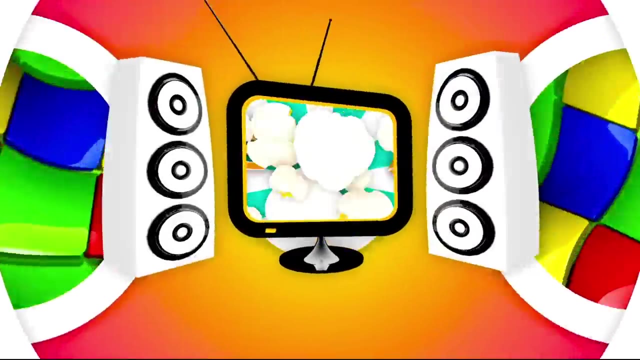 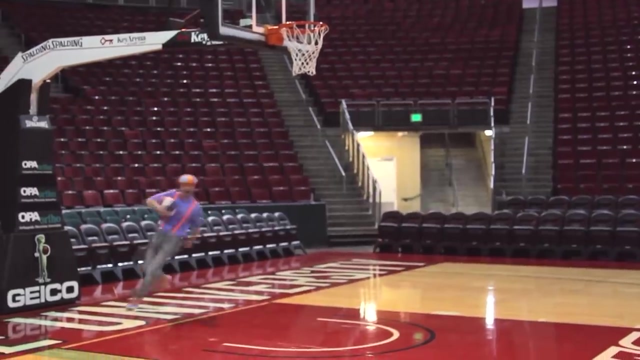 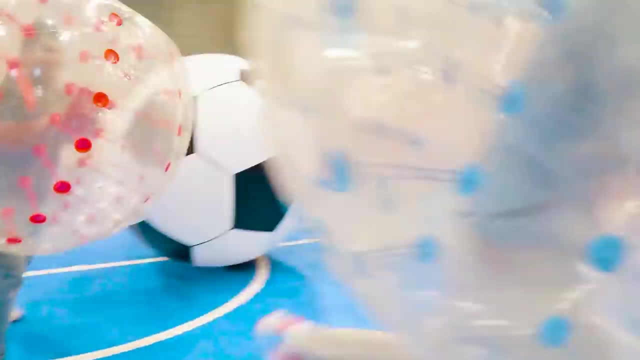 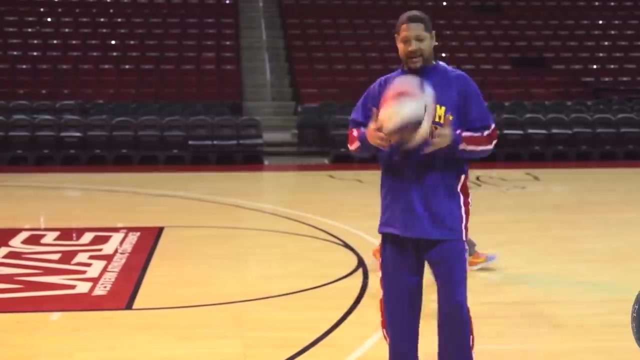 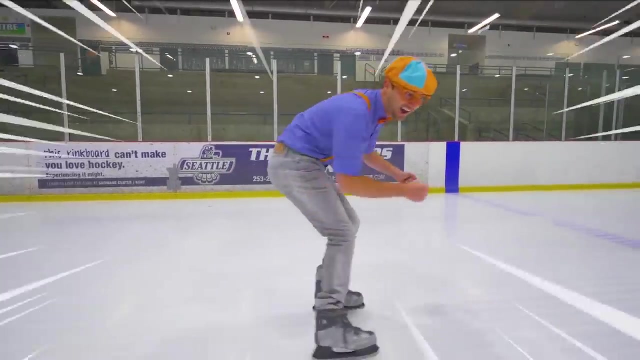 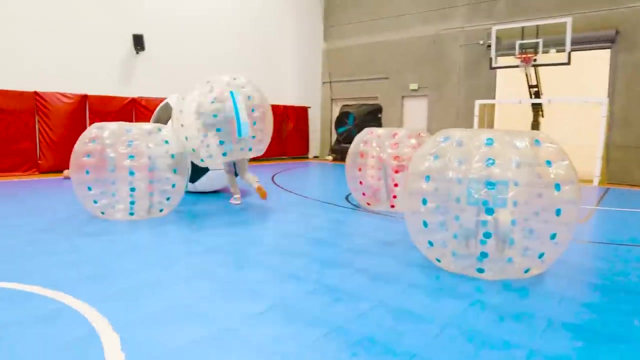 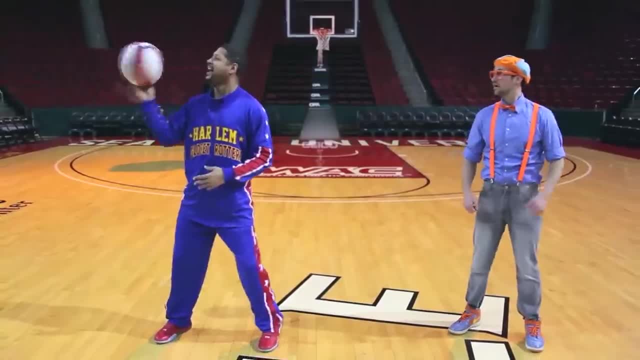 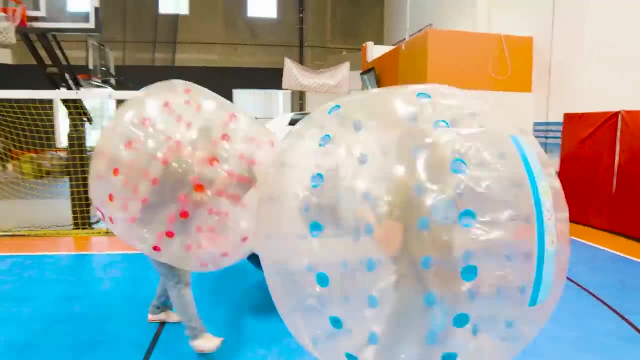 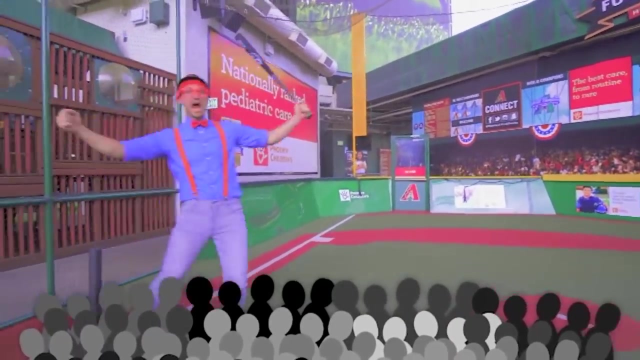 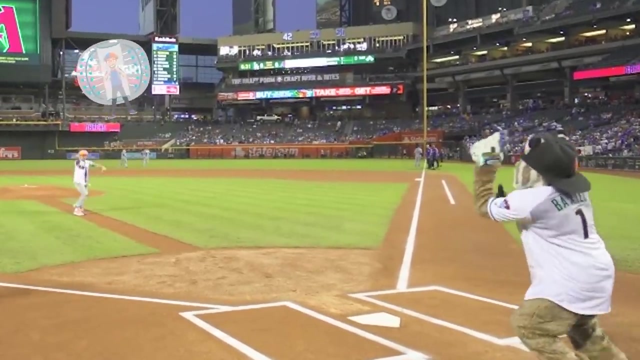 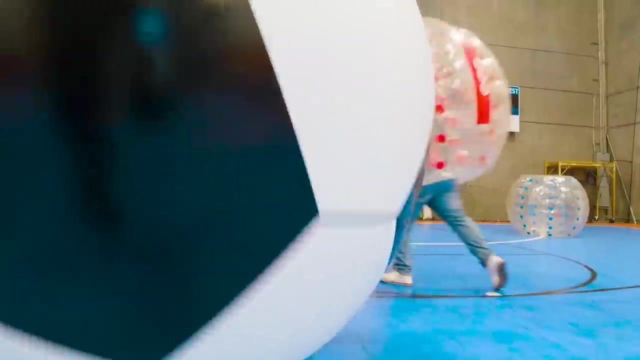 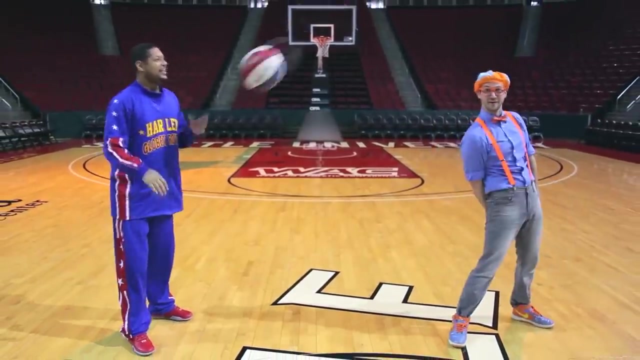 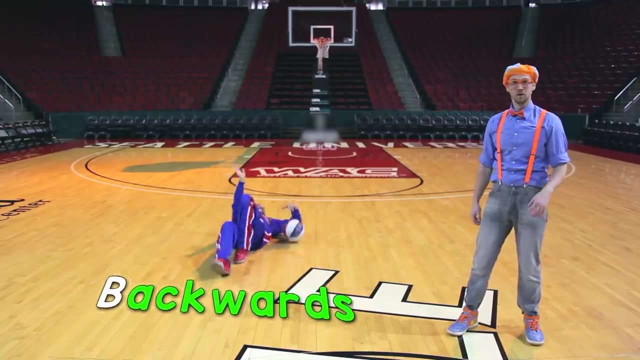 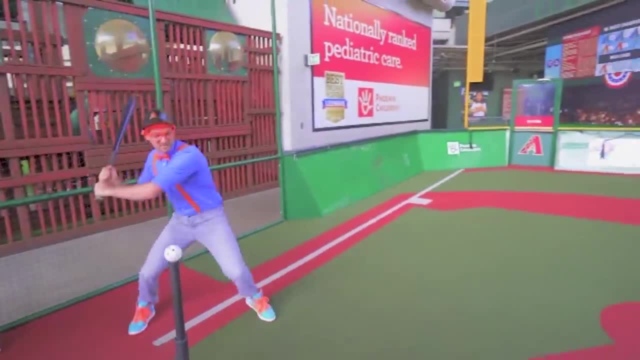 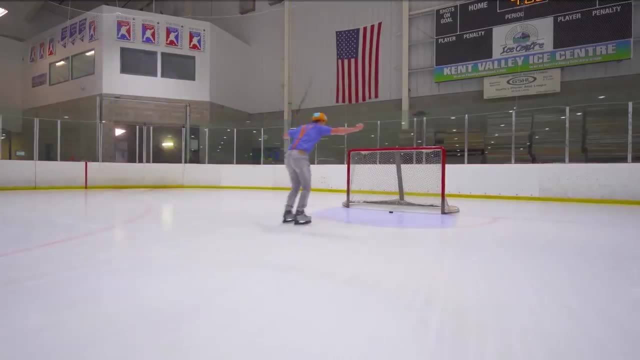 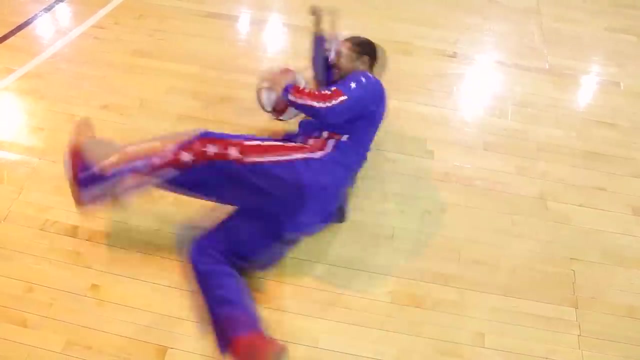 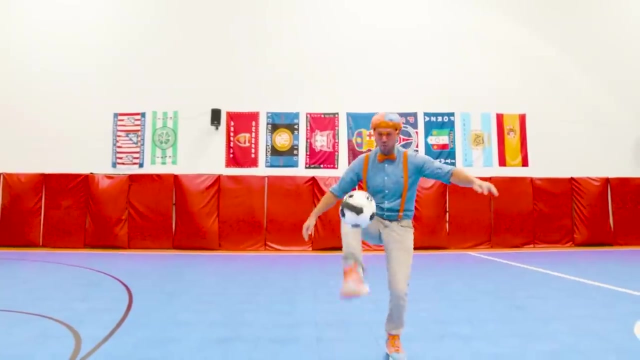 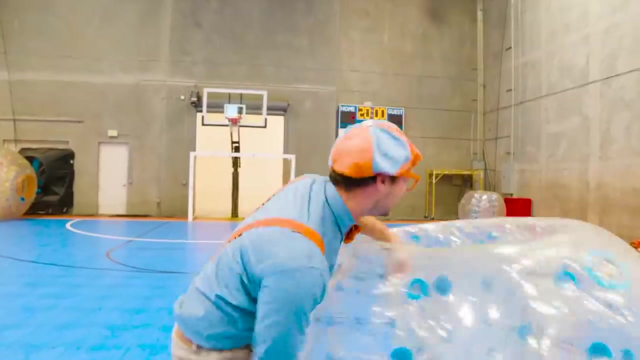 Run, pass and score. Make friends forever. All for one and one for all. Together, we can win it all. Sports take skills. You learn something new. Practice and practice, Practice is what you gotta do. Teamwork is dreamwork. We play together, Run, pass and score. 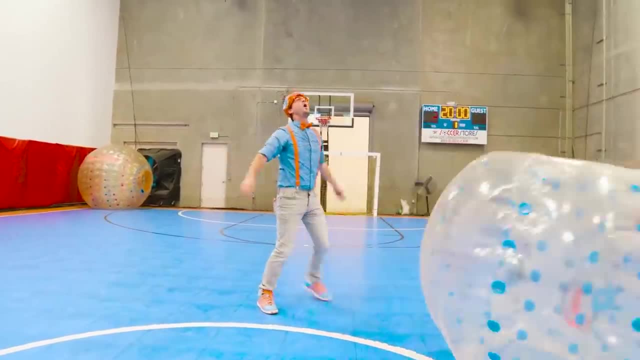 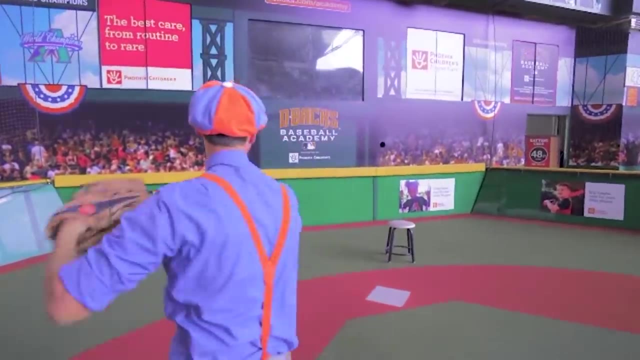 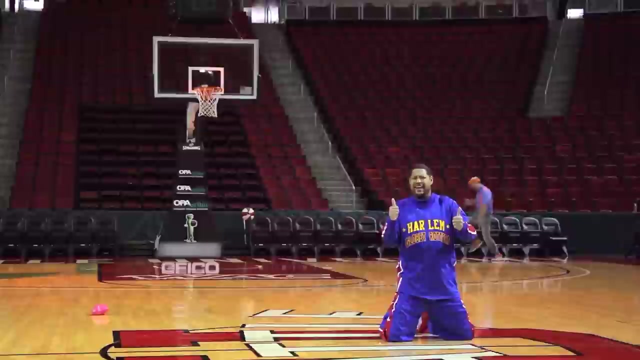 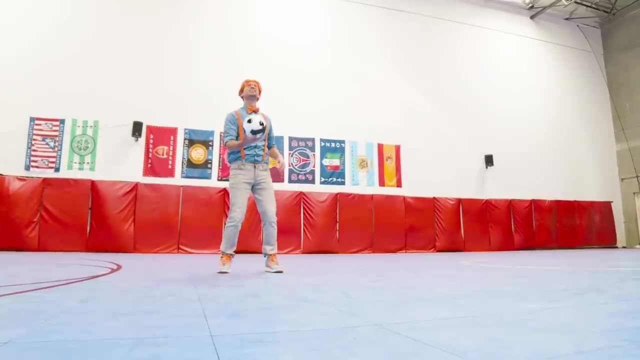 Make friends forever. Teamwork is dreamwork. We play together Dribble pass score. Make friends forever. All for one and one for all. Together, we can win it all. Teamwork is dreamwork. We play together, All for one and one for all. Ready set set. 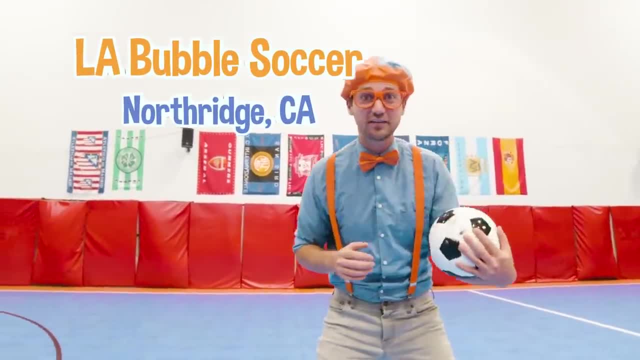 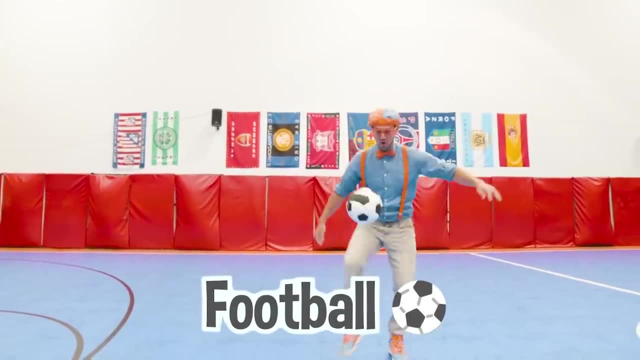 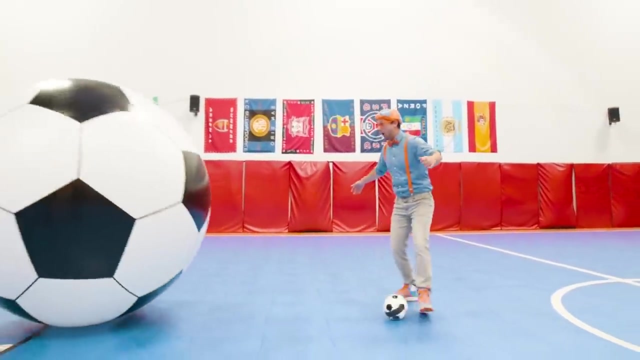 Teamwork is dreamwork. We play together, We play and we play together, We play and we play together. Hey, it's me Blippi, and today I'm at LA Bubble Soccer in North Ridge, California, and check it out. This is a soccer ball. 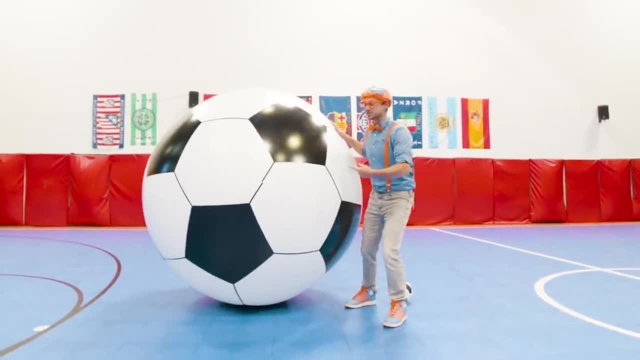 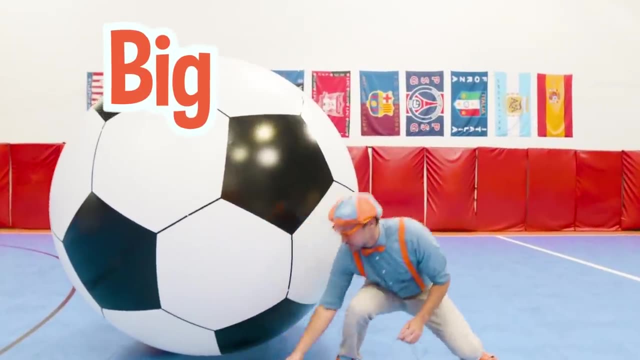 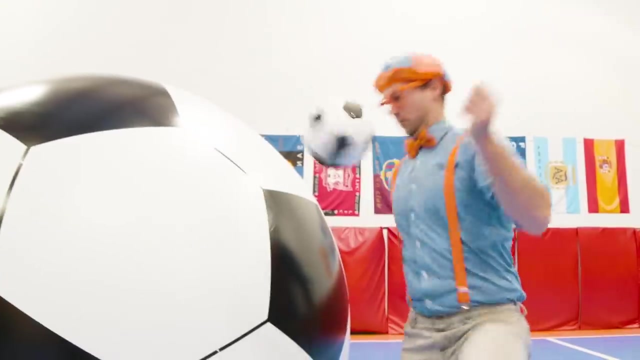 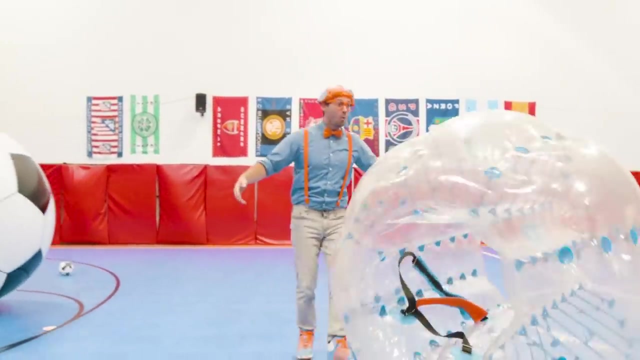 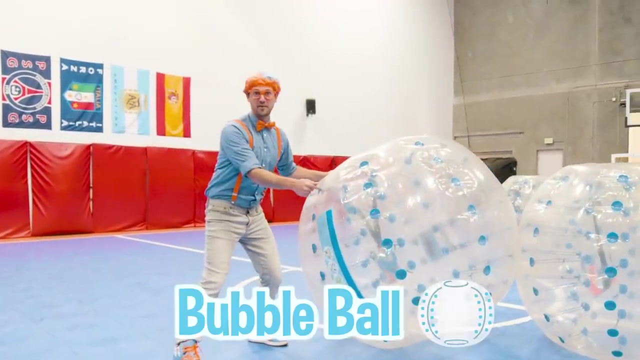 Yeah, some countries call it a football Whoa. so fun to play with whoa. and this football soccer ball is really big and this one is small. i love playing with soccer balls. whoa, what's this? whoa? it looks like a bubble. yeah, bubble, bubble ball. this sport is. 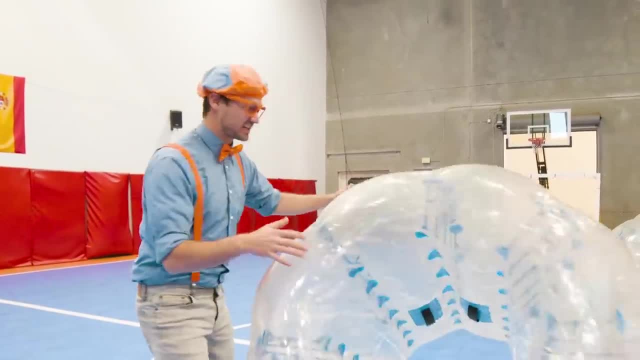 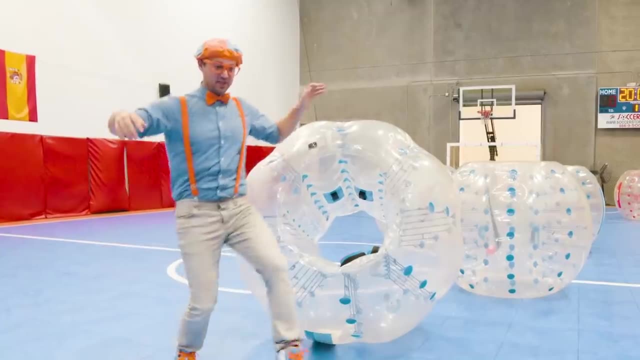 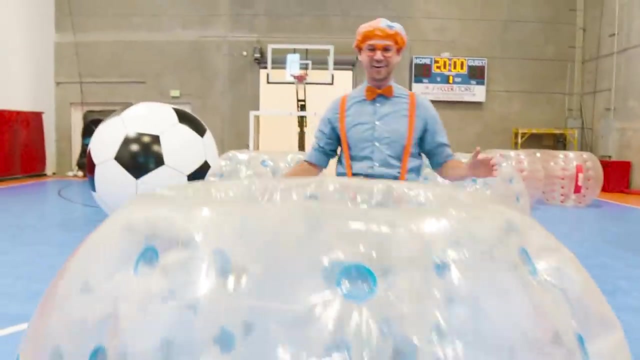 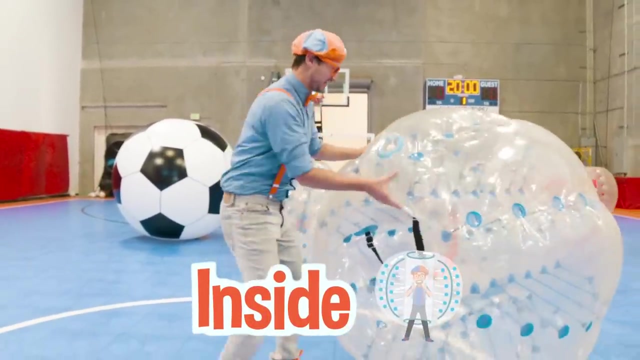 called bubble ball. it's basically like soccer football, but you get inside these bubbles with your body and then you play soccer and football. check it out, whoa. the first thing that you have to do before you play bubble ball is get inside the bubble ball. okay, hey, did you hear how i said? 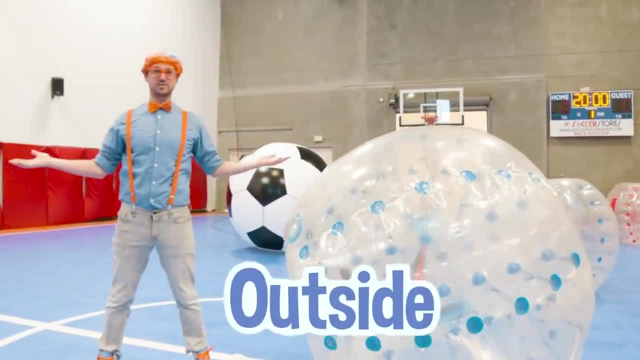 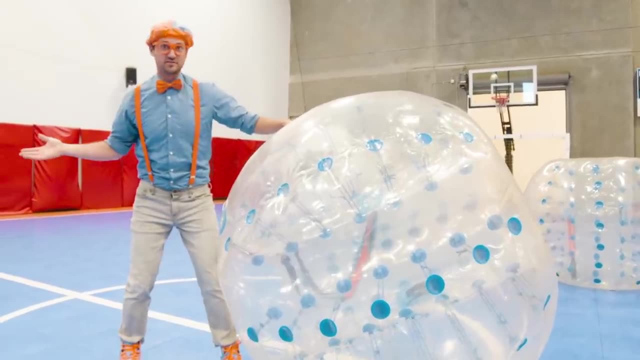 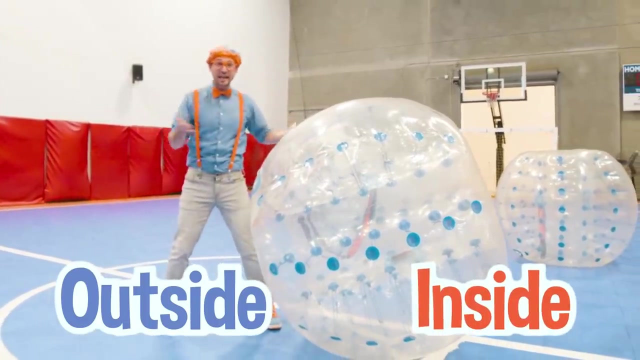 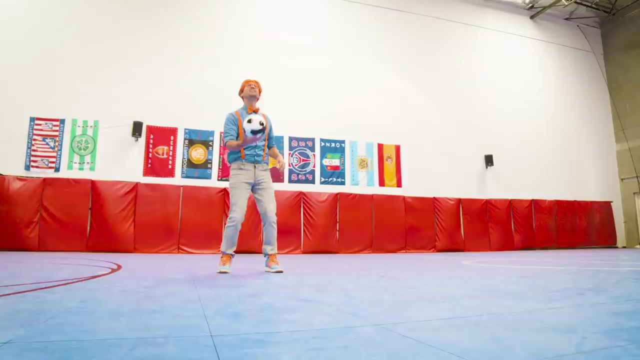 inside. yeah, that means i am outside the bubble ball. do you know what an opposite is? an opposite is the exact reverse of something totally different. so if i'm outside and then i need to go inside, inside and outside are opposites. so now that i'm outside, let me get inside. what is the opposite? what is the opposite? 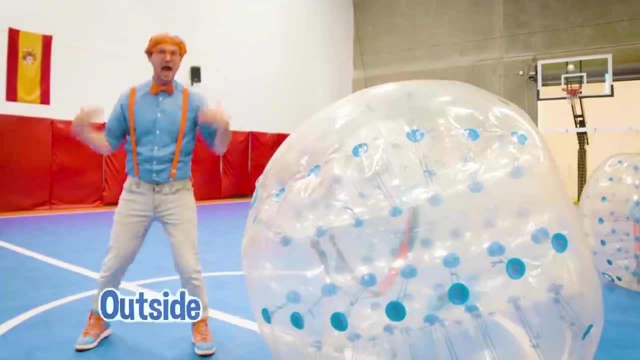 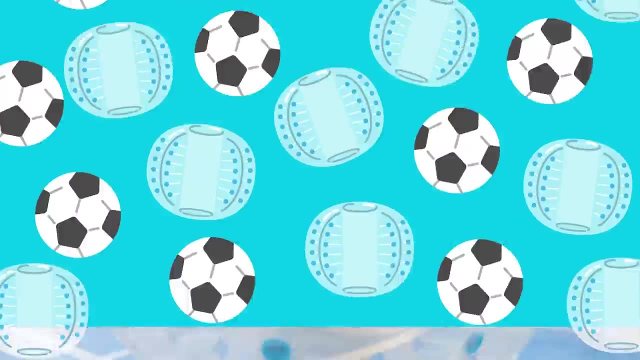 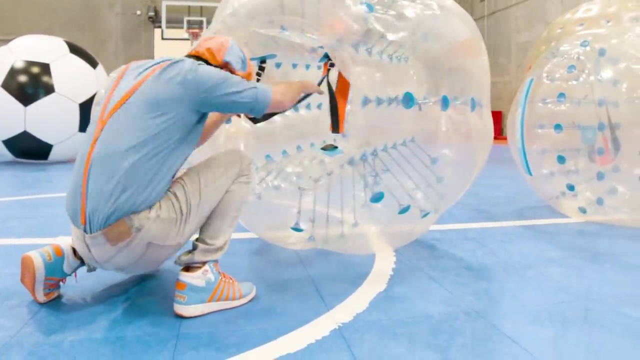 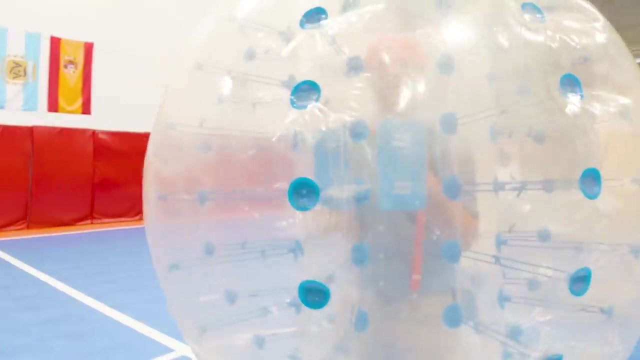 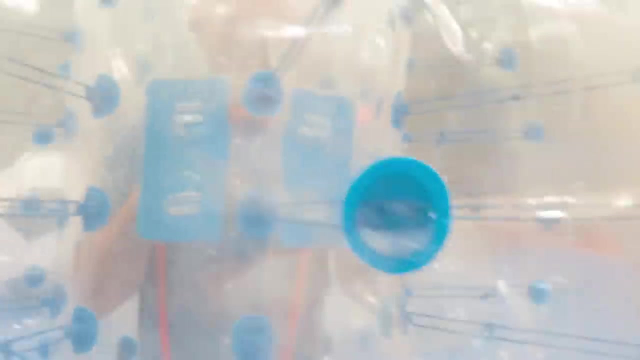 what is the opposite of inside the ball, outside the ball, outside the ball outside's the opposite of inside the ball. okay, this is pretty tricky, but see these straps. you put it on like a backpack and you put it in just like this: whoa, hey, hello. do you see me? whoa, all right, now it's time to have some fun. 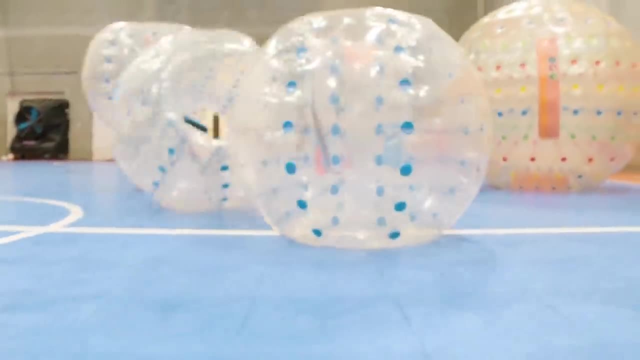 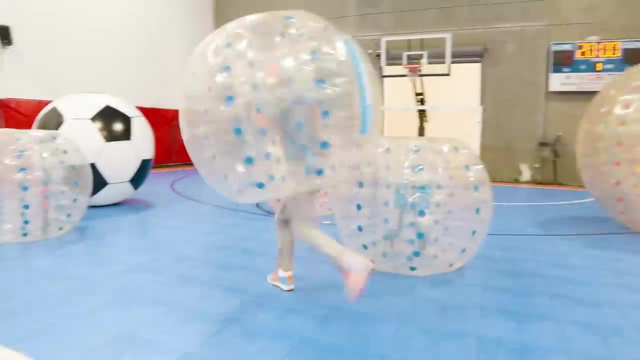 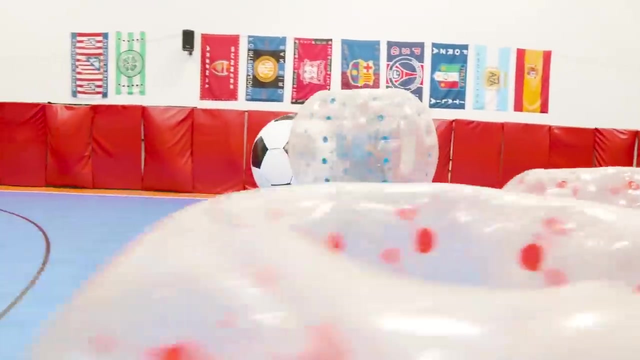 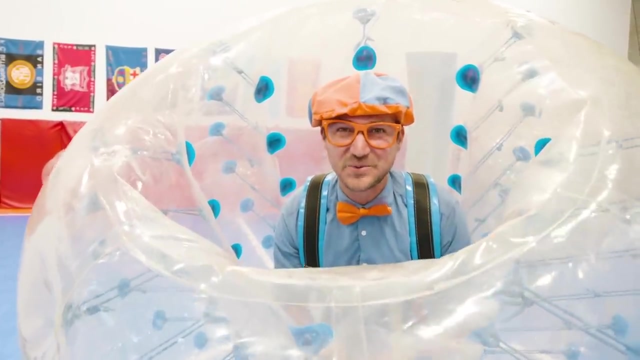 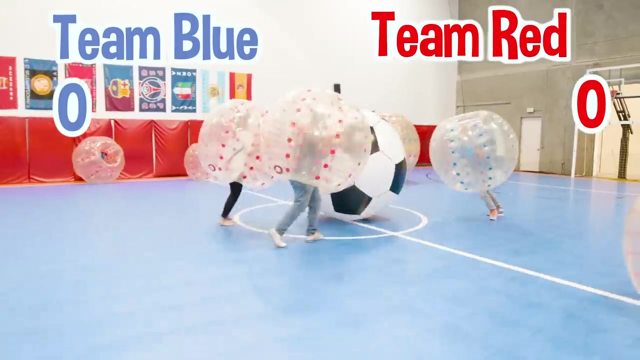 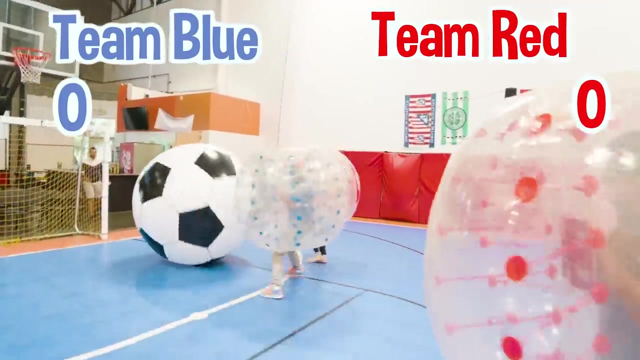 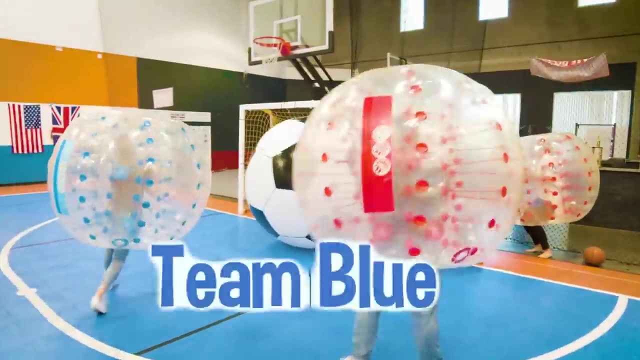 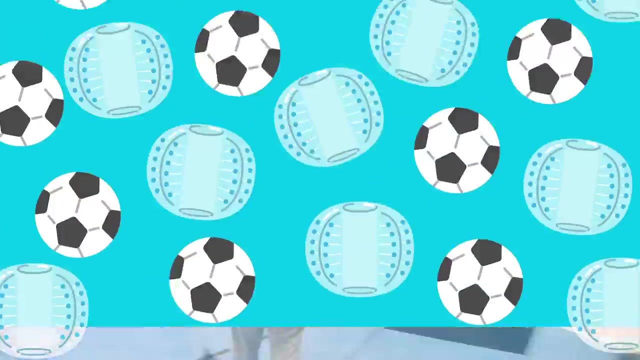 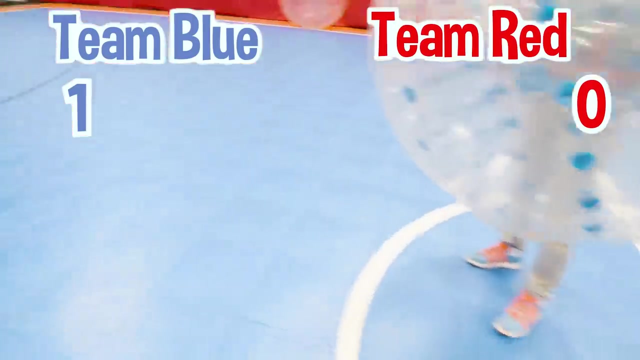 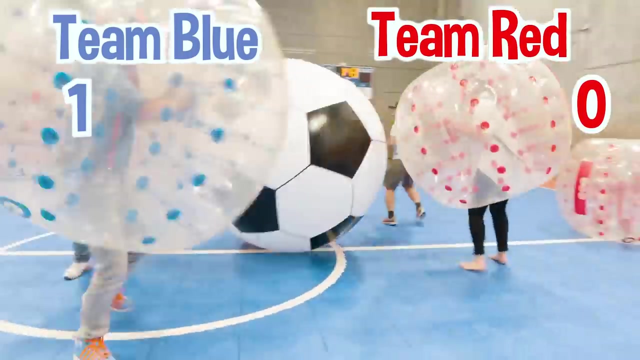 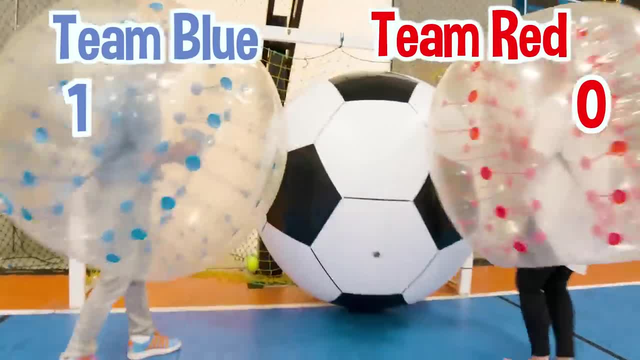 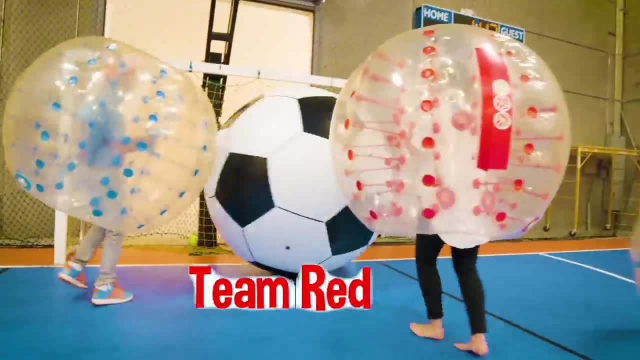 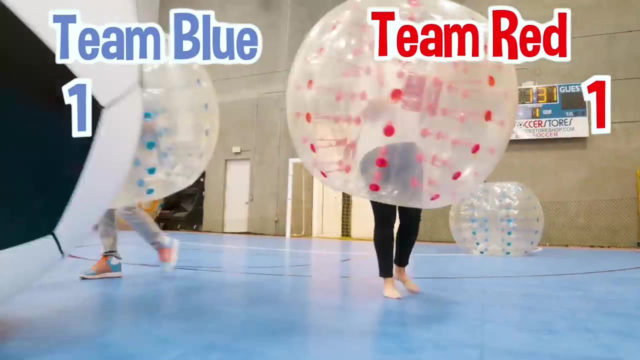 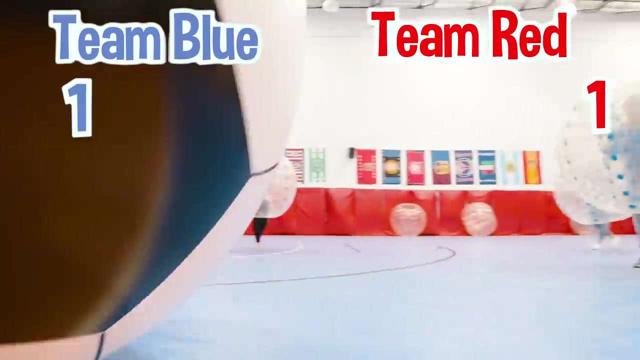 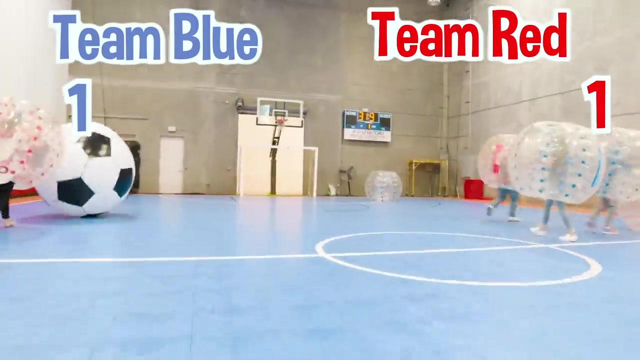 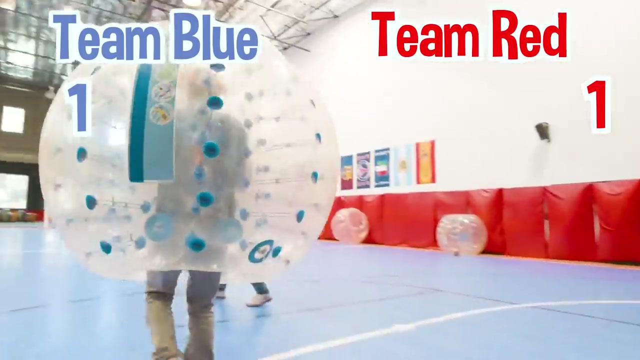 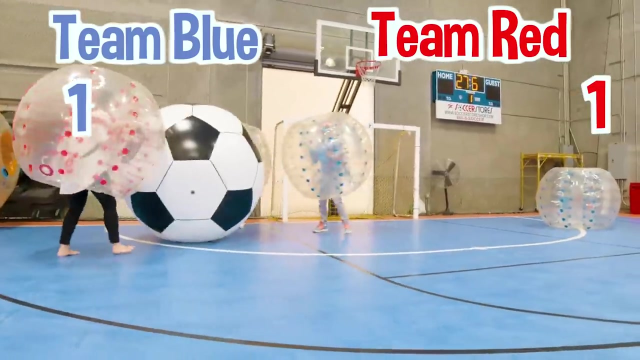 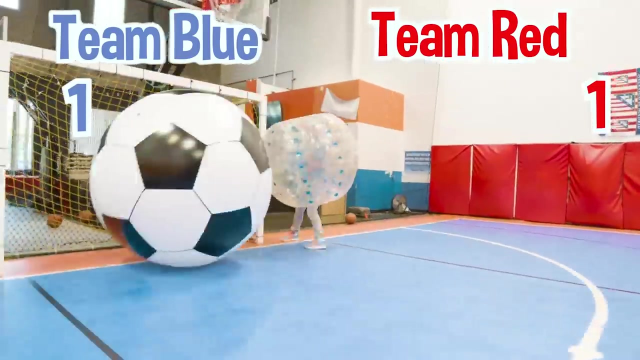 oh, oh, oh. goal for the reds. goal for the reds. we're having so much fun. goal for the reds. oh, oh, oh. so it's, it's, it should, or, oh, might be. uh okay, health ur prue. Go for Blippi, Go for Blippi. 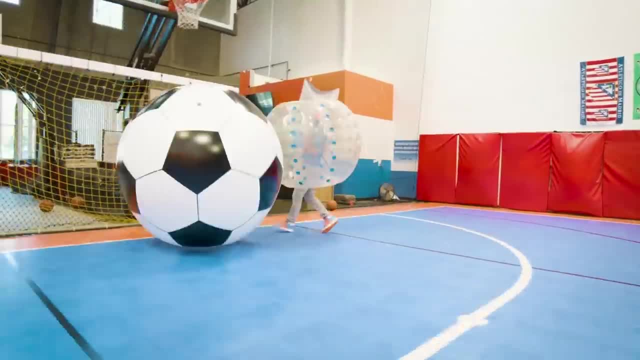 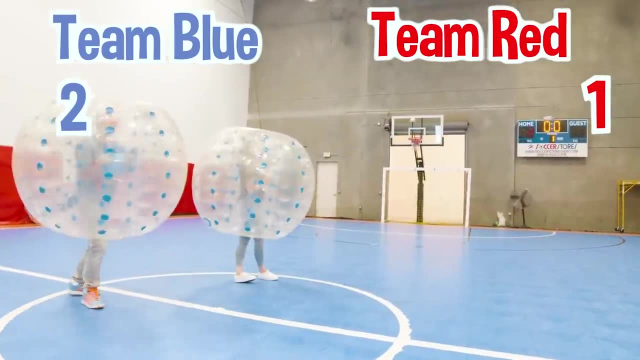 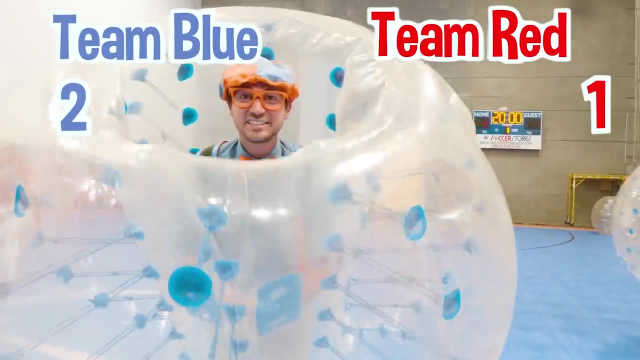 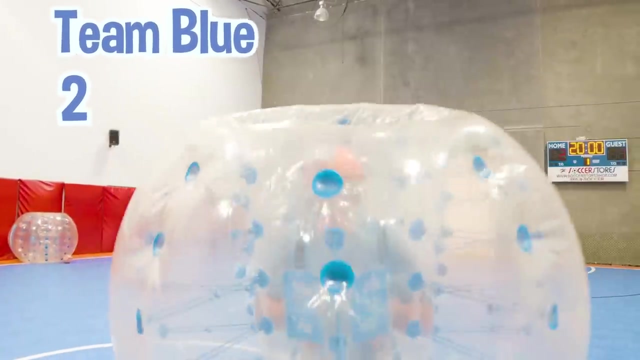 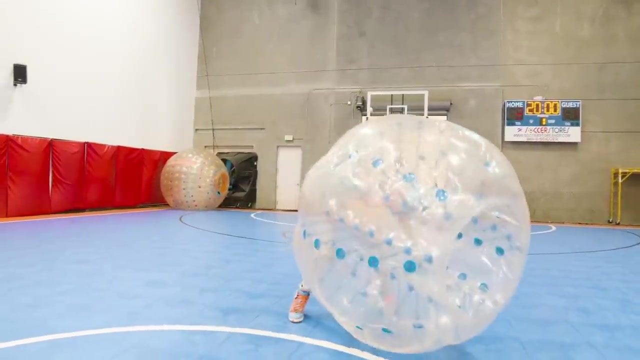 He's got so much energy, Go for Blippi. Oh, I am so tired And Team Blue won- Woohoo. Everyone did a really good job at Bubble Ball today. Oh, Oh, I am so hot and sweaty right now. 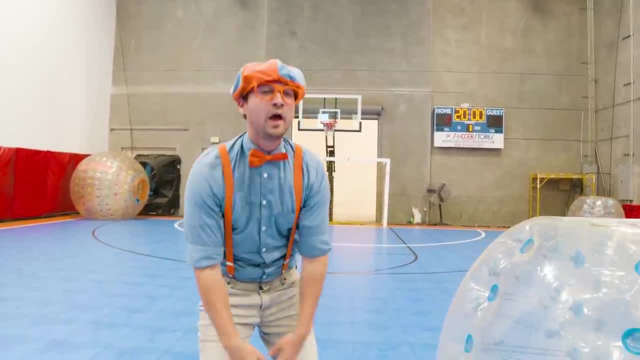 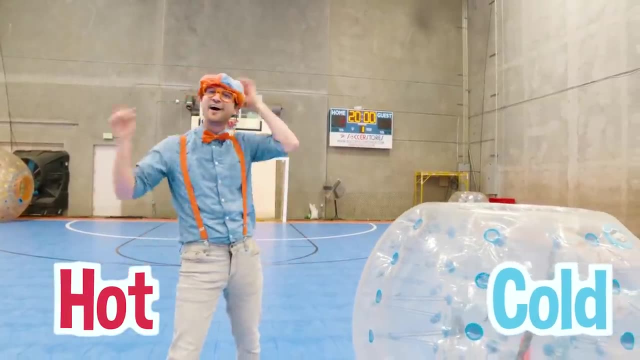 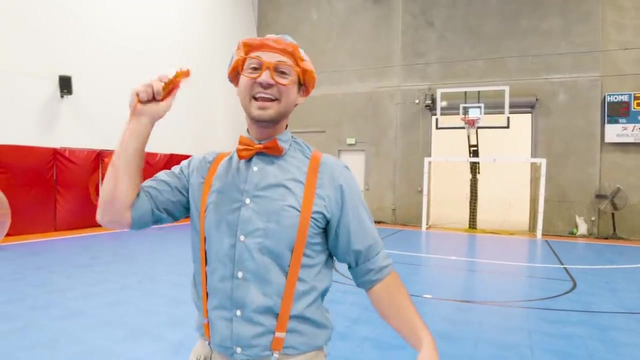 Oh, Do you see this? Oh Hey, I have an idea. The opposite of hot is cold. I have a fan right here, See, Whoa. Maybe if I put the fan I will become cold. Oh Yeah, it's working. 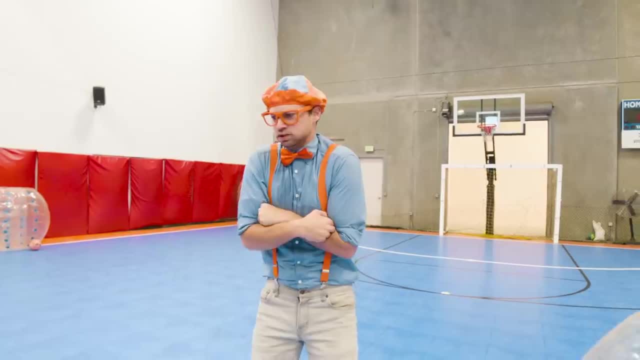 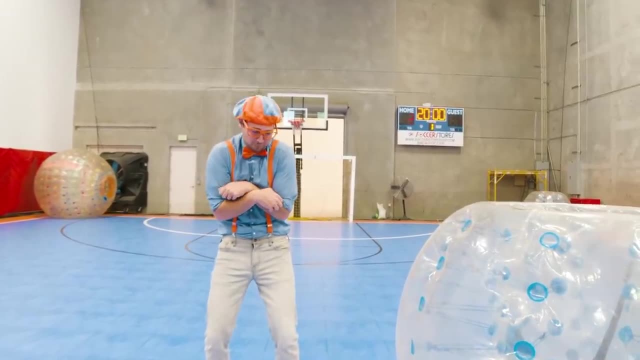 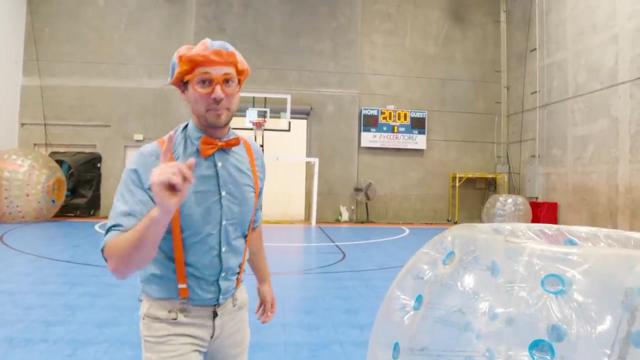 Brr, Oh, brr, Brr. Oh, I'm so cold now. Oh, I used to be hot and then now I'm cold, Hehehe. Ah Well, this was so much fun learning about Bubble Ball with you. 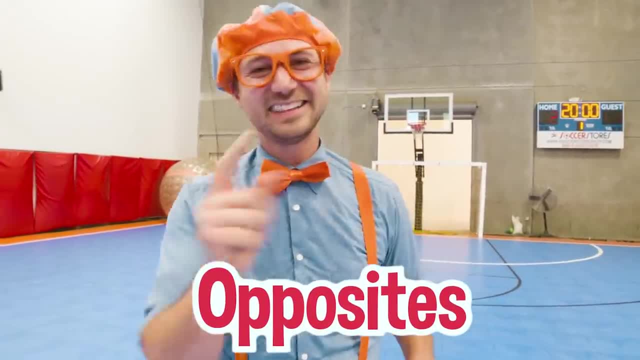 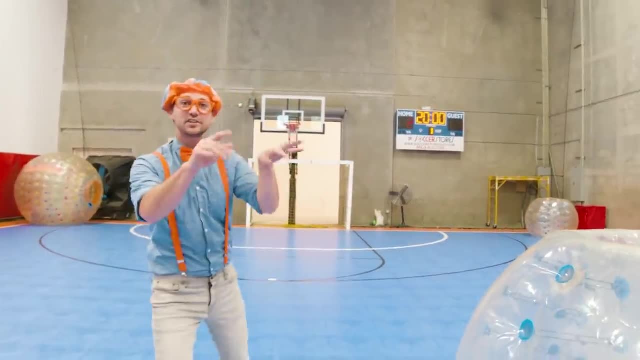 And opposites. Yeah, I love learning with you, But this is the end of this video. But if you want to see more of my videos, all you have to do is search for my name. Will you spell my name with me? 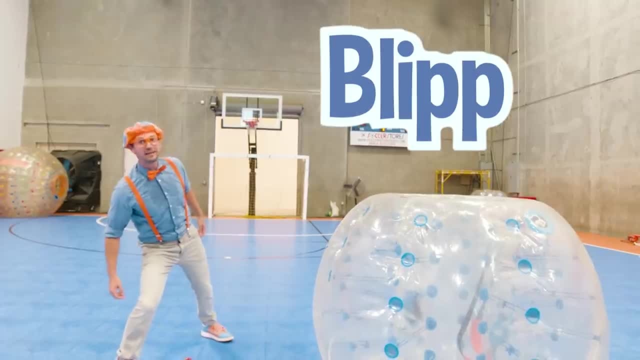 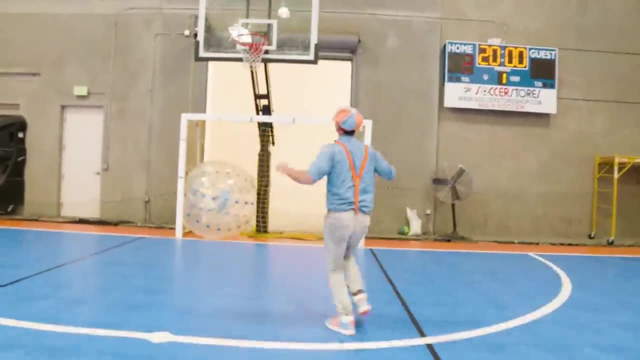 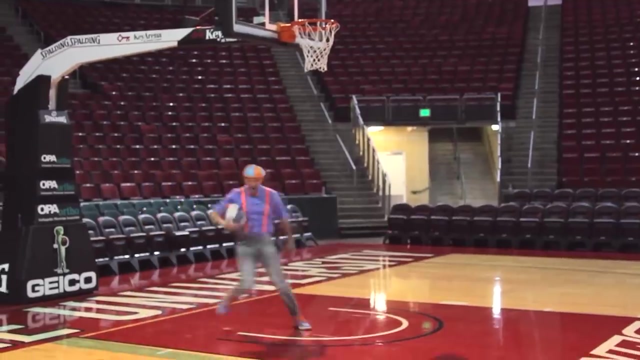 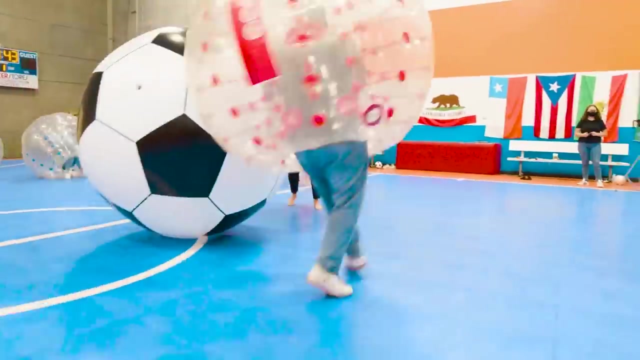 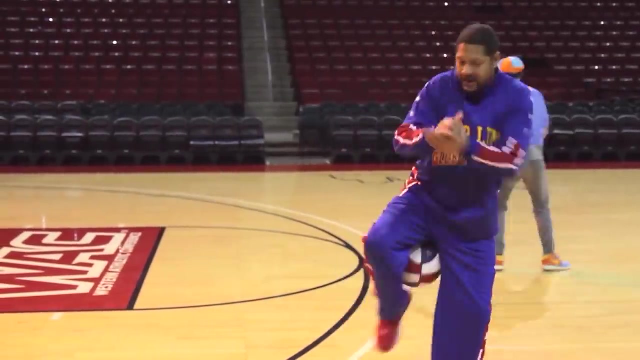 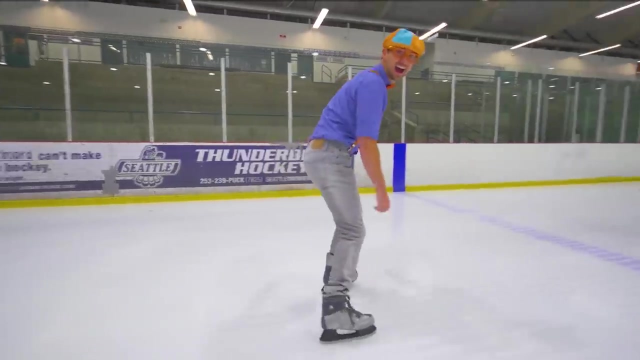 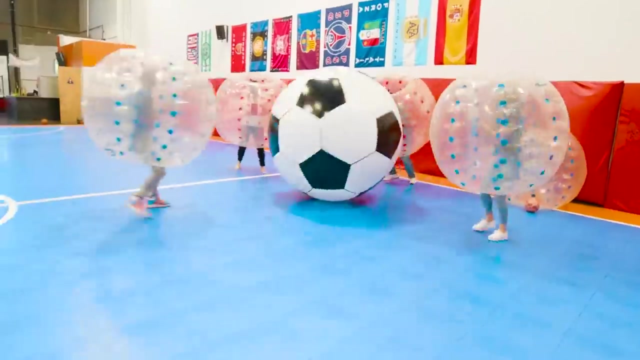 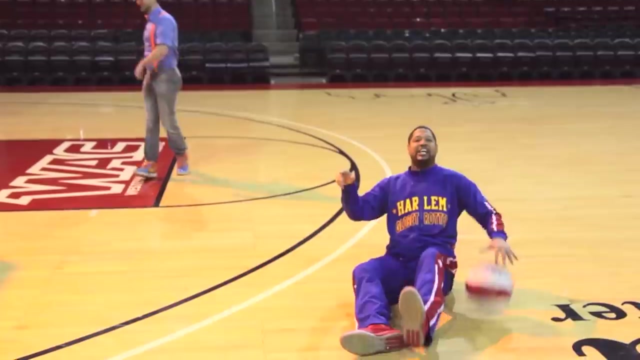 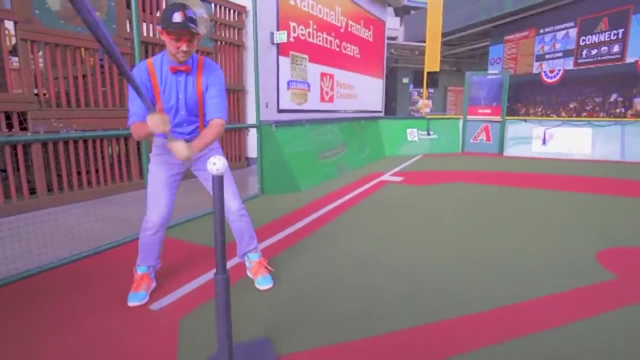 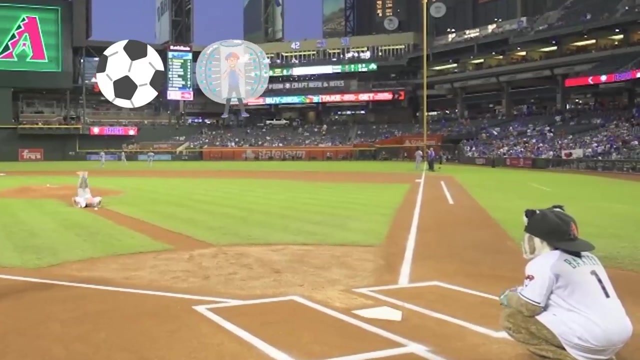 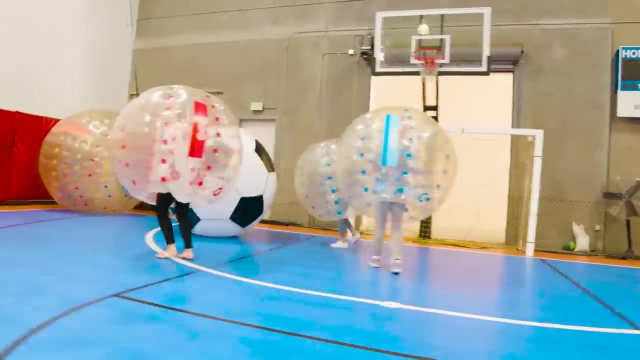 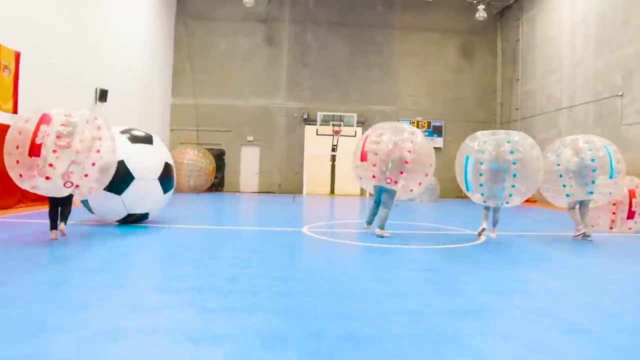 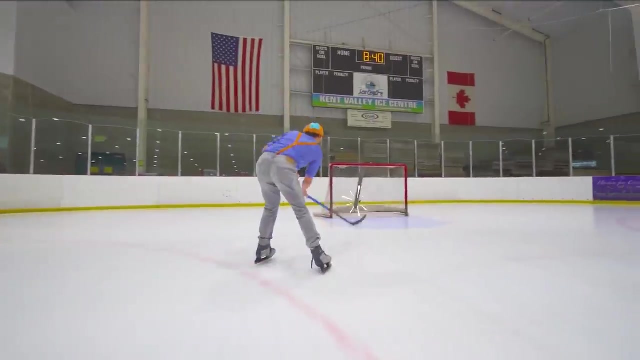 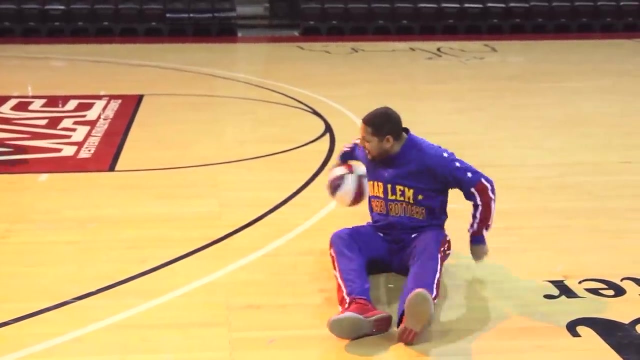 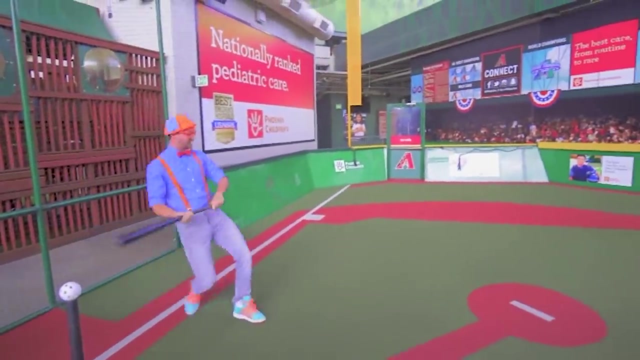 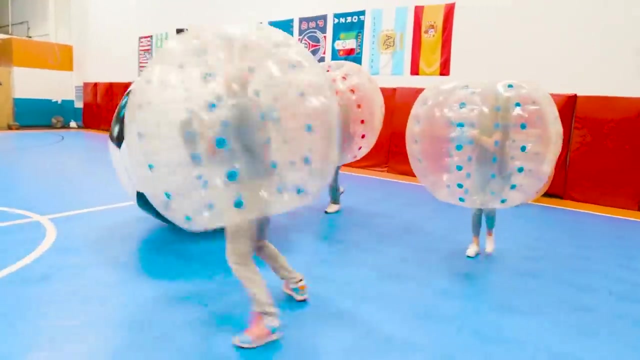 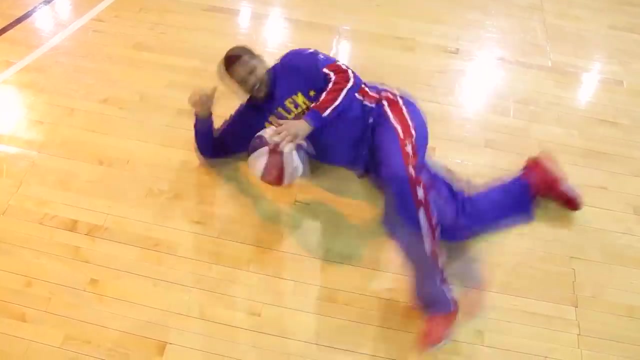 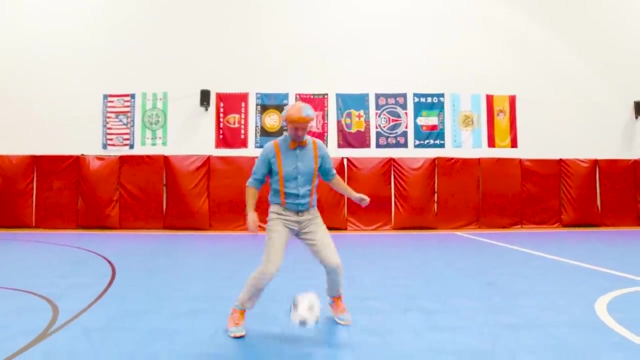 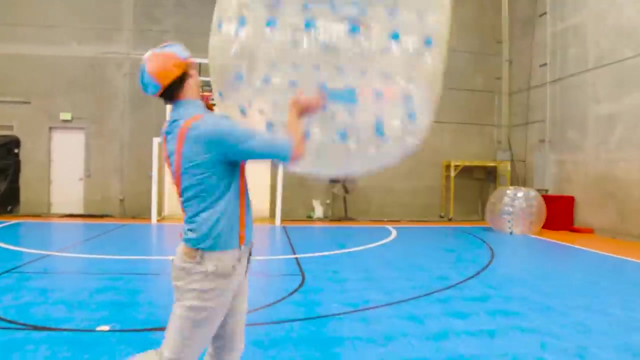 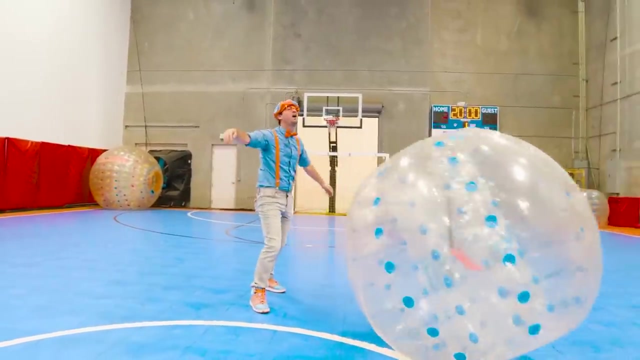 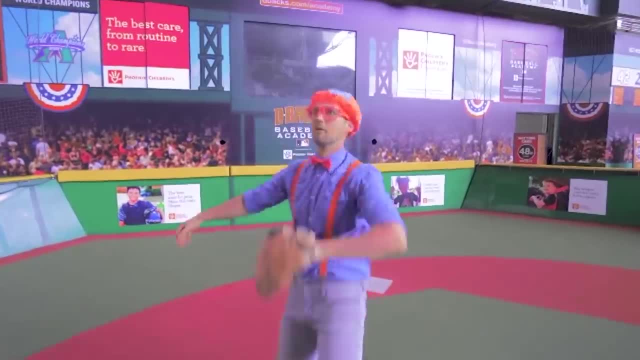 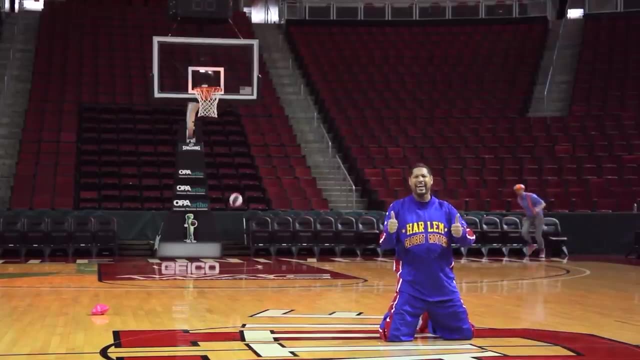 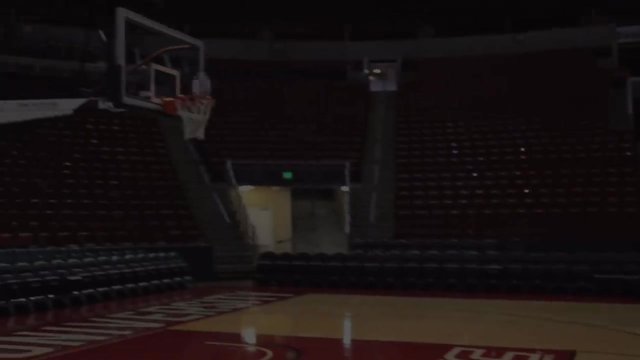 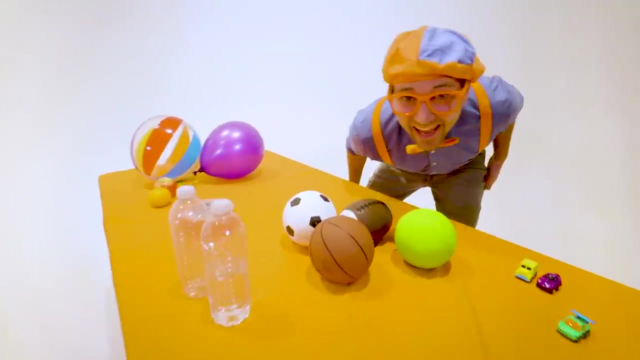 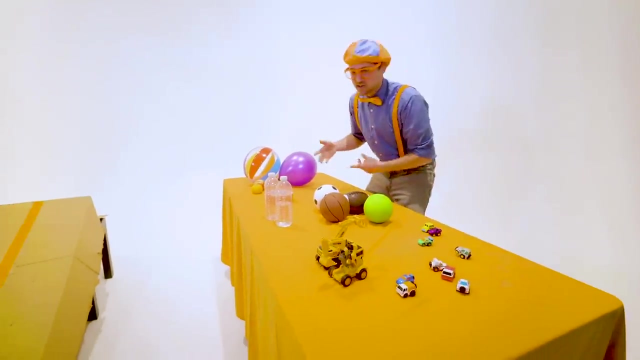 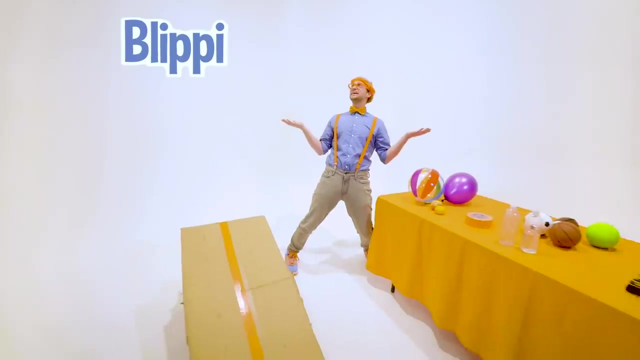 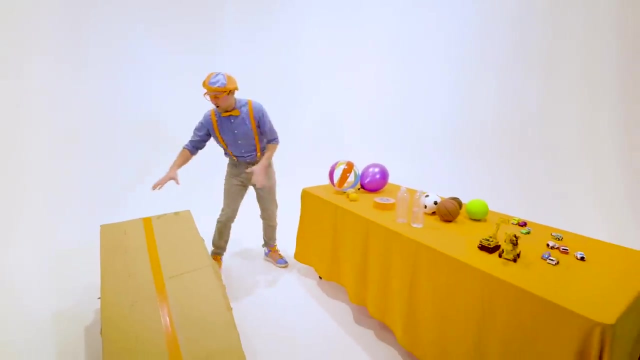 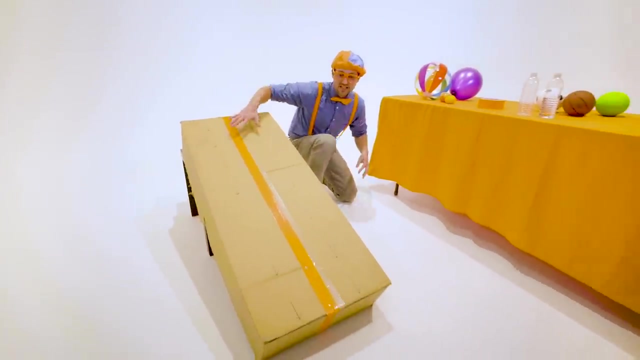 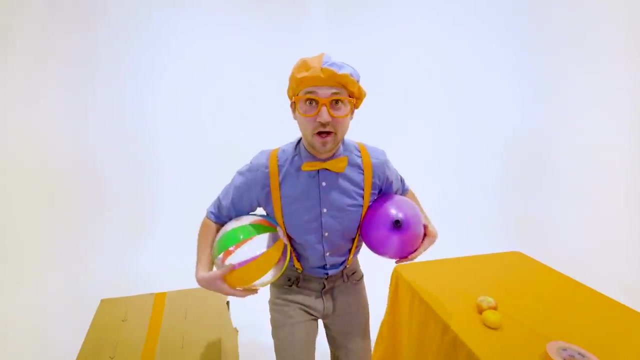 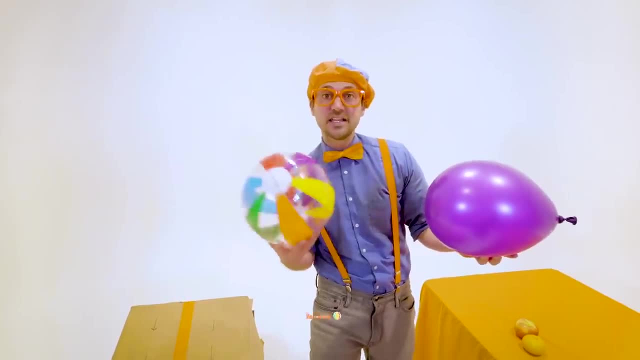 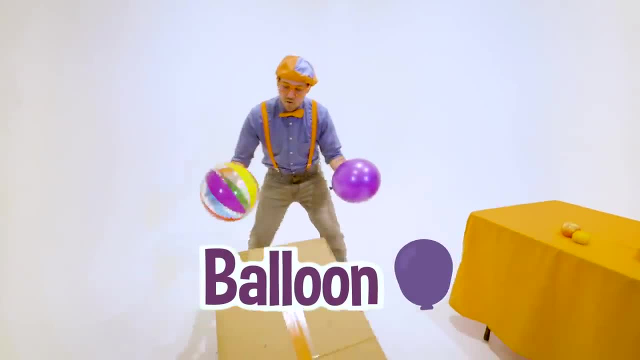 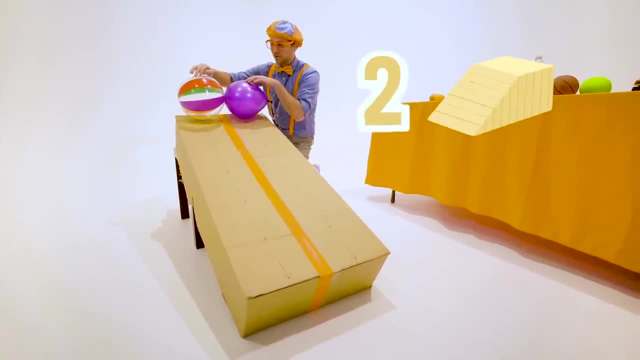 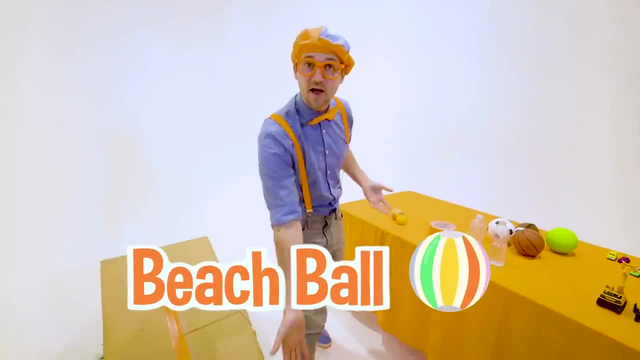 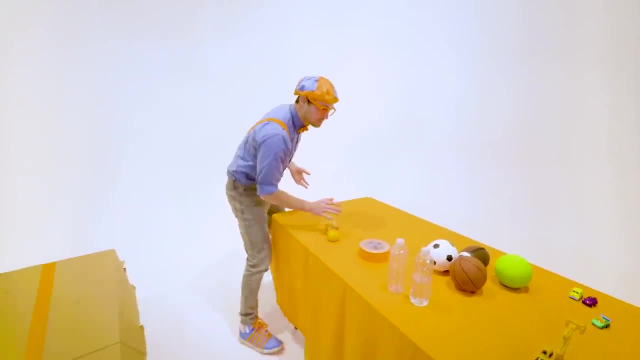 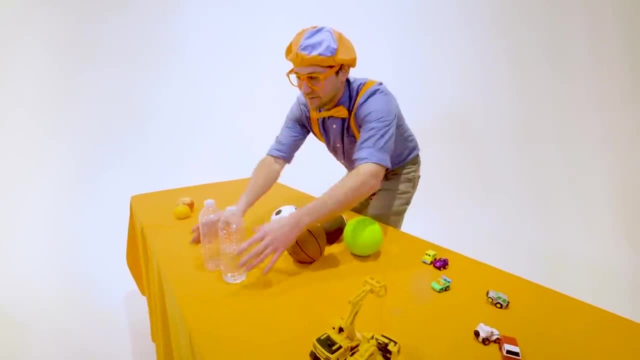 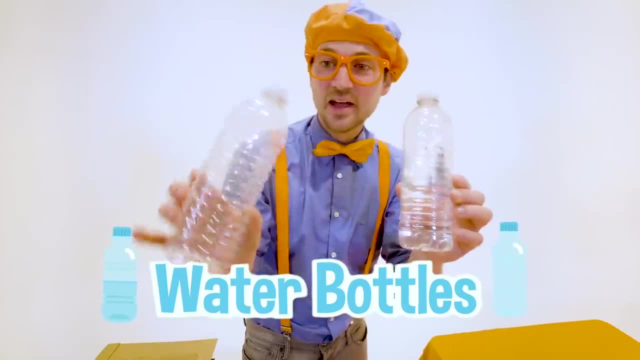 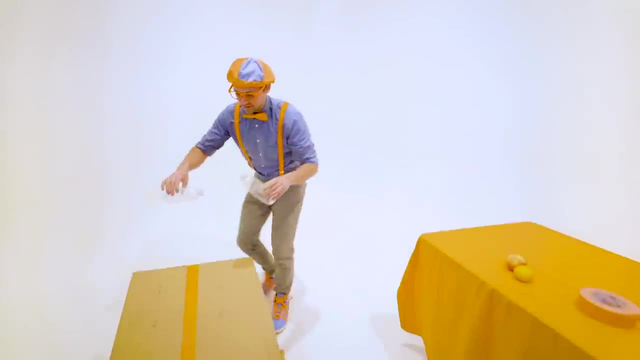 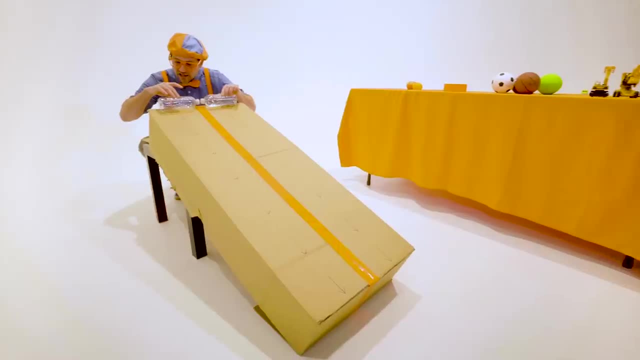 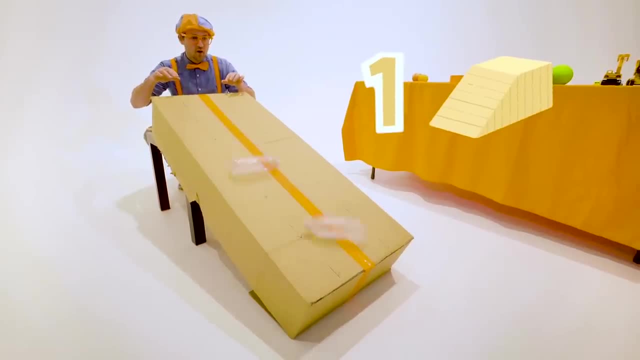 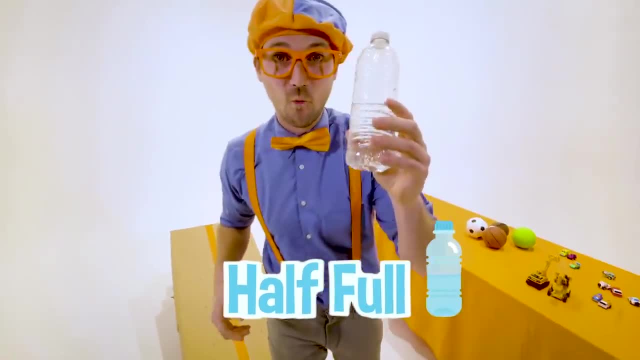 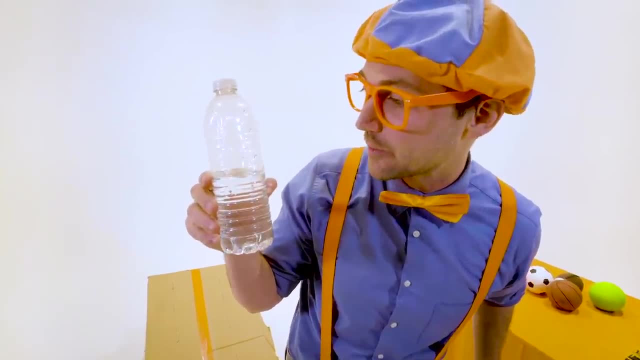 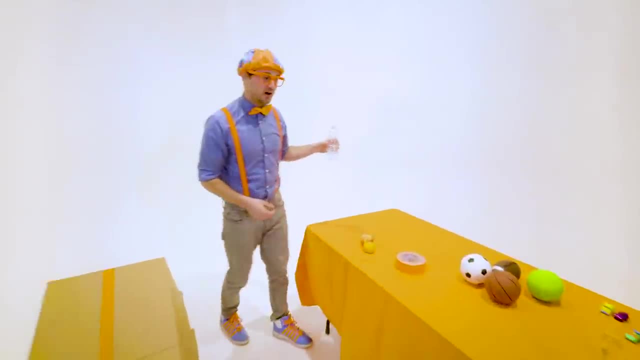 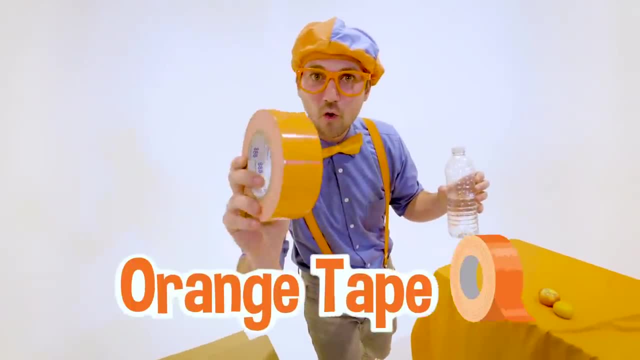 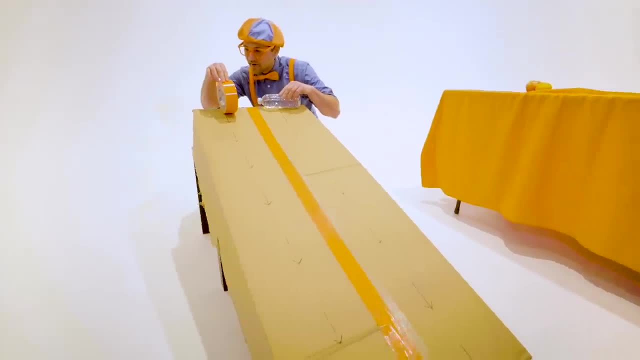 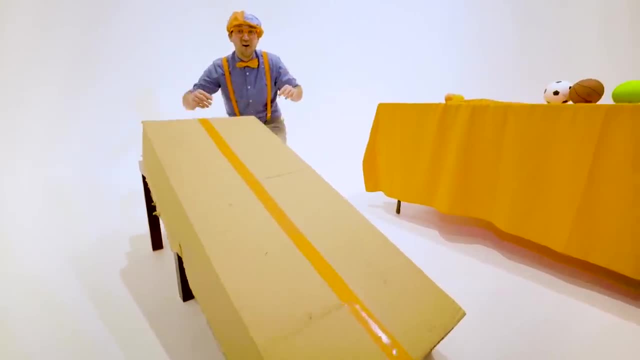 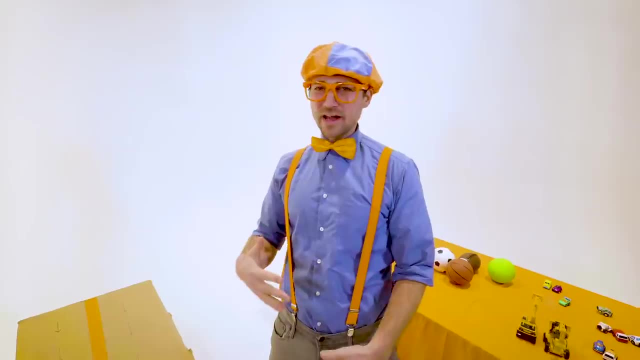 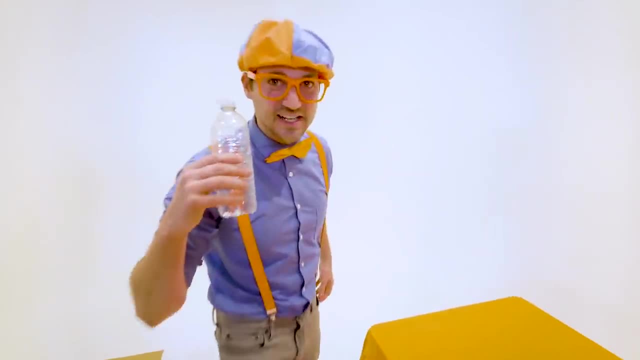 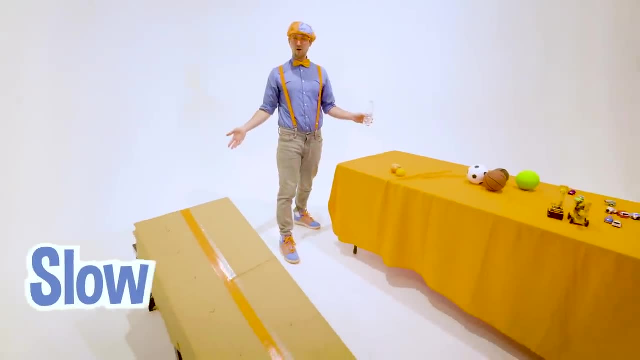 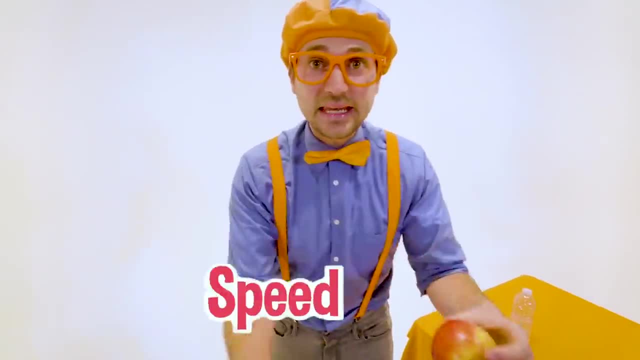 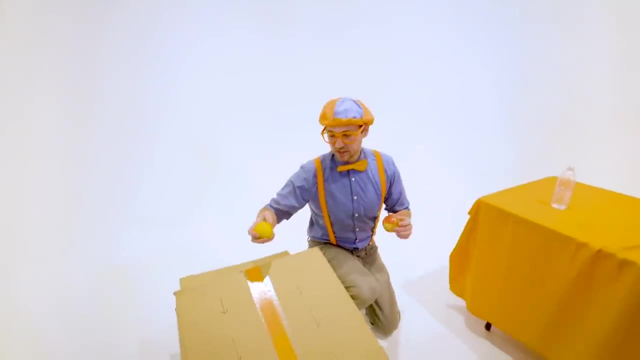 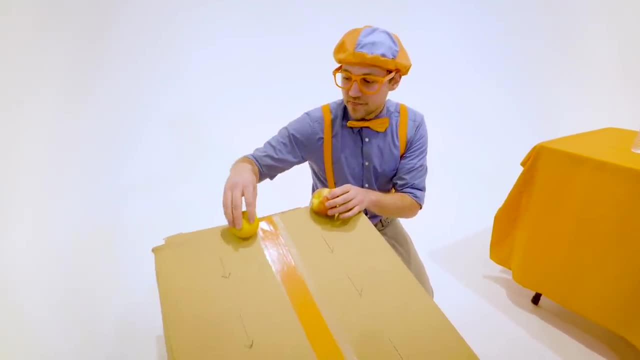 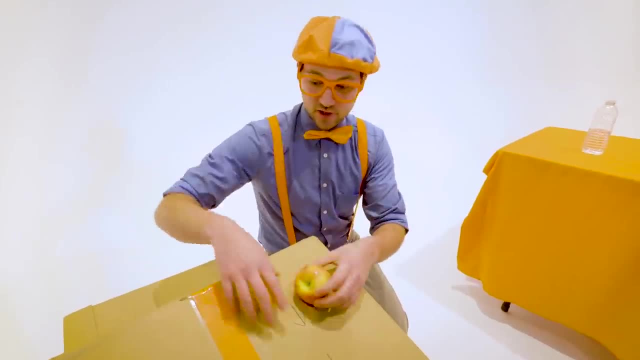 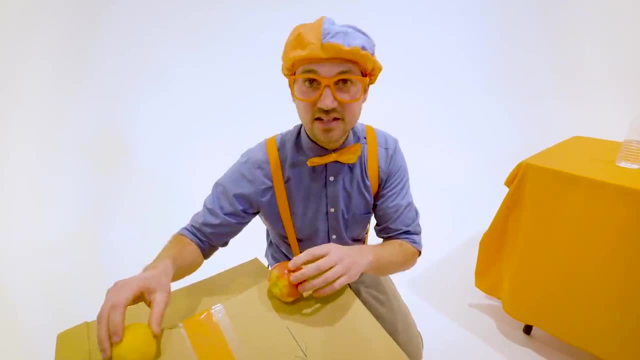 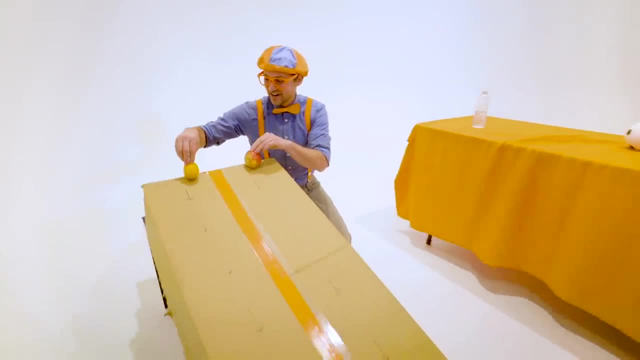 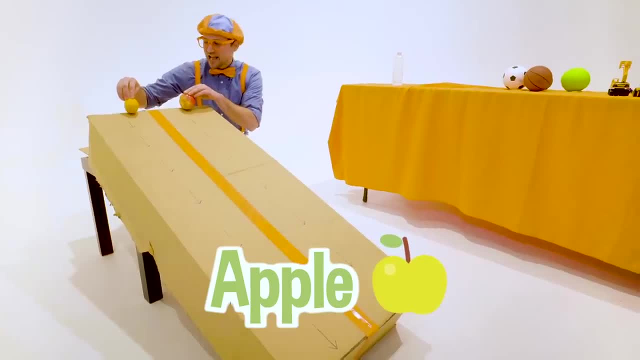 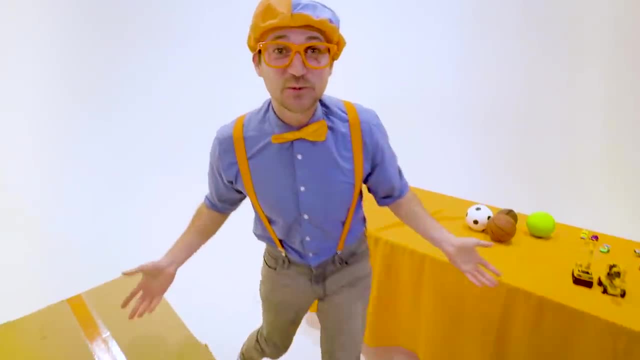 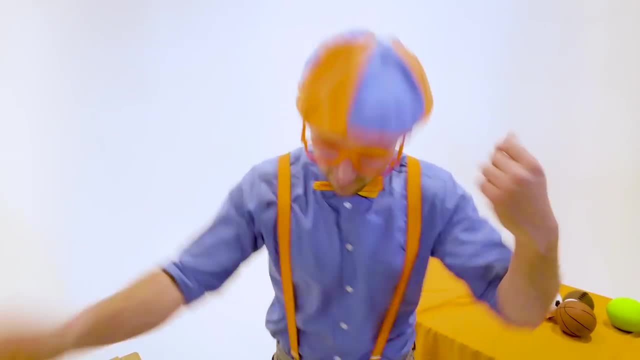 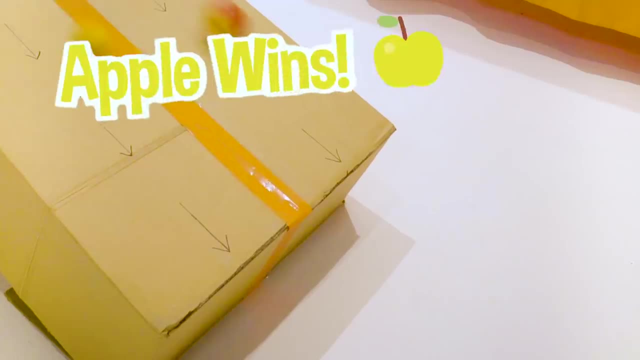 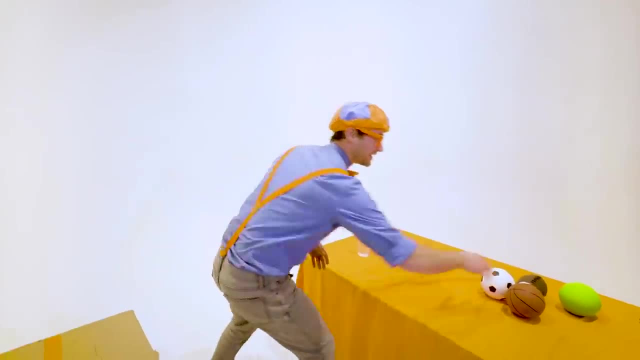 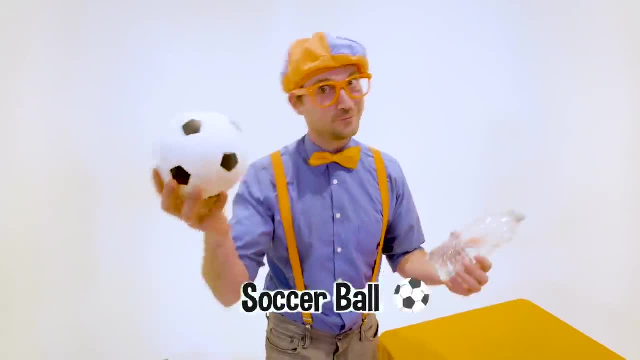 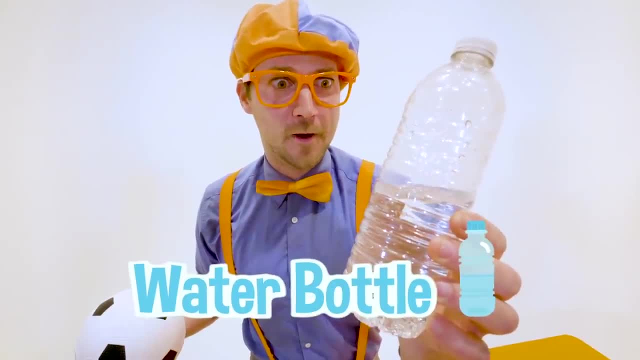 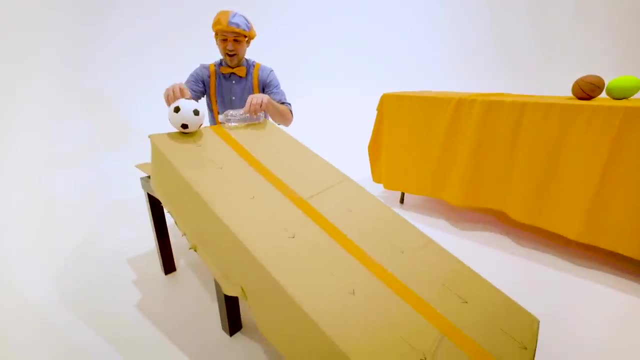 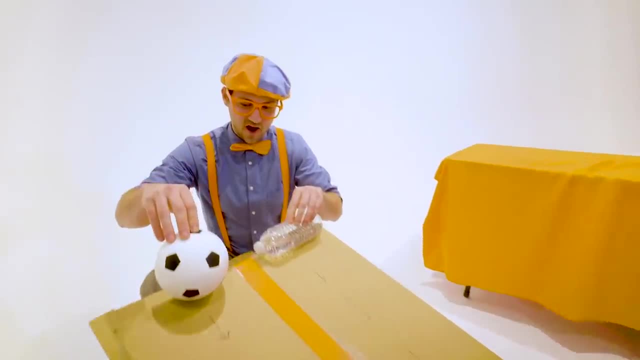 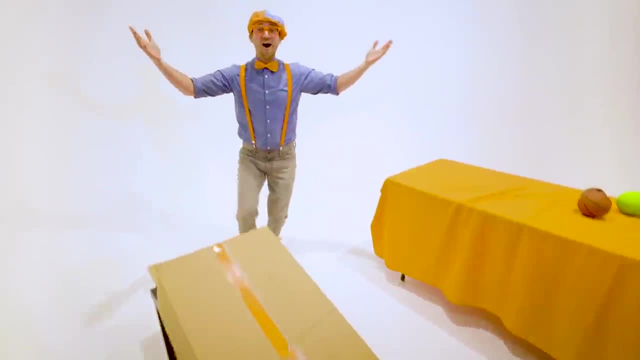 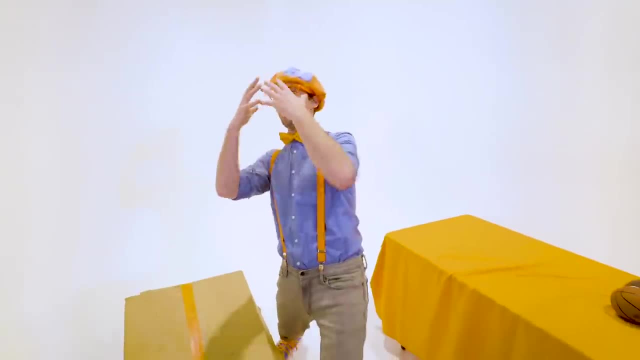 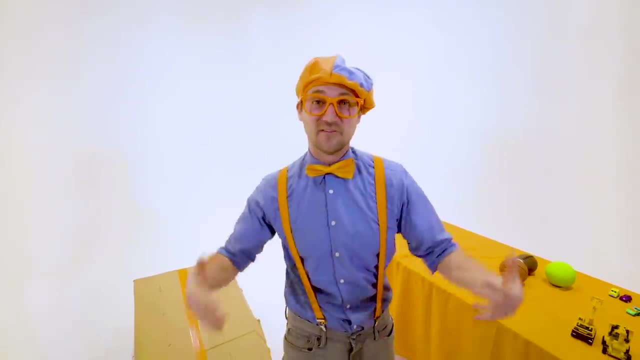 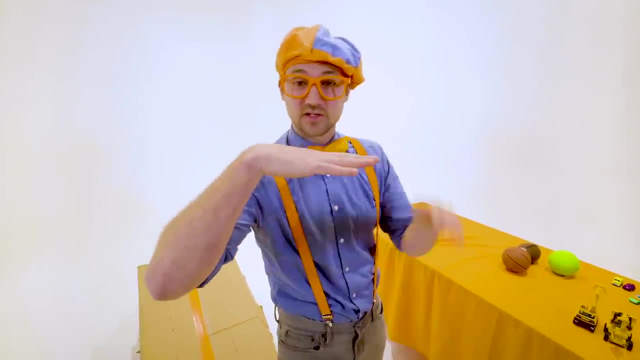 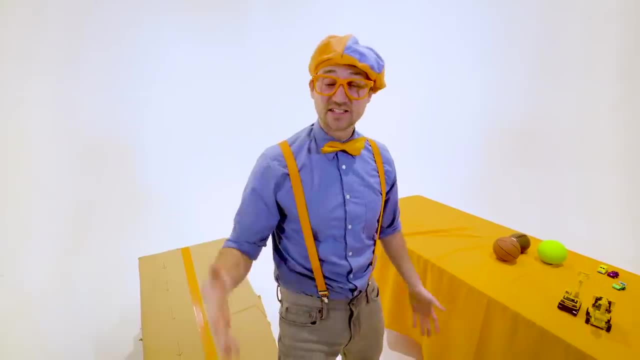 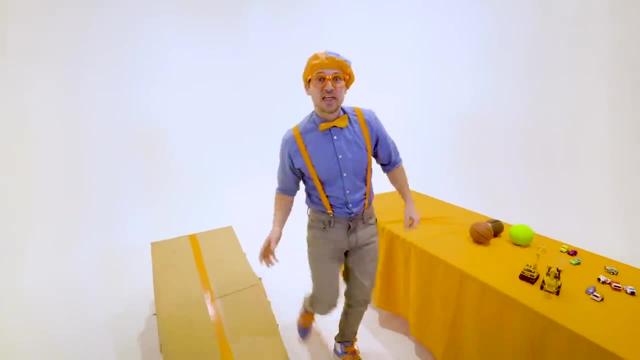 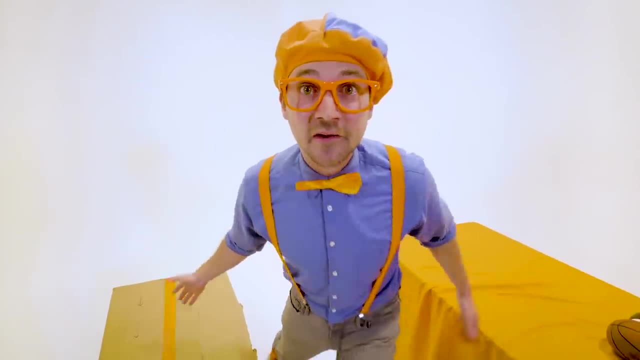 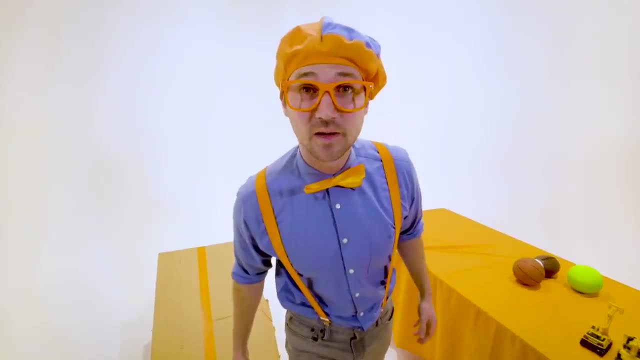 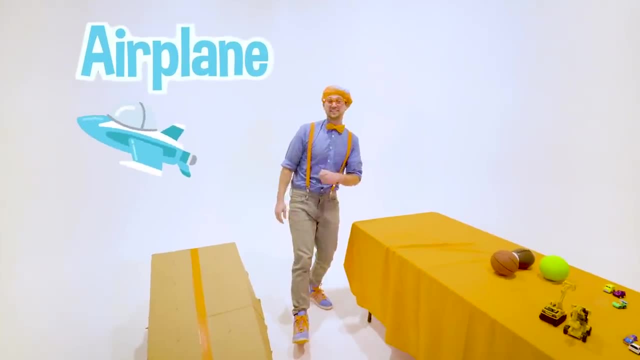 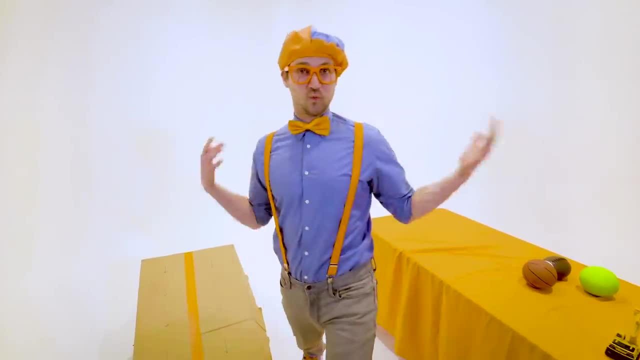 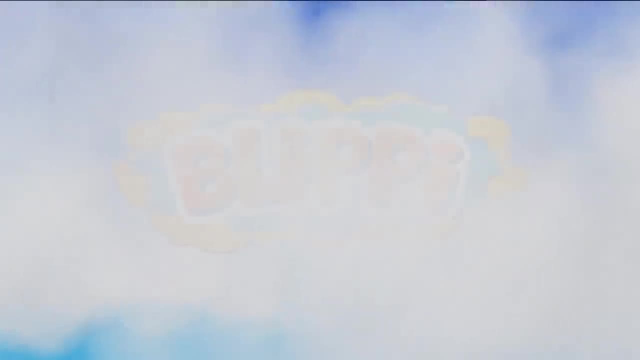 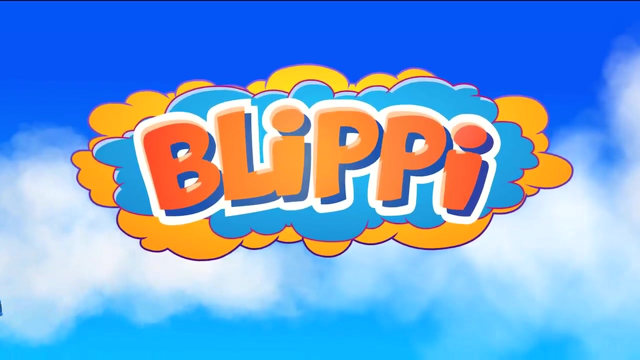 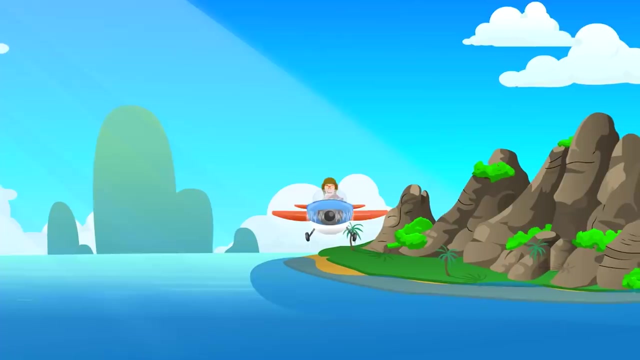 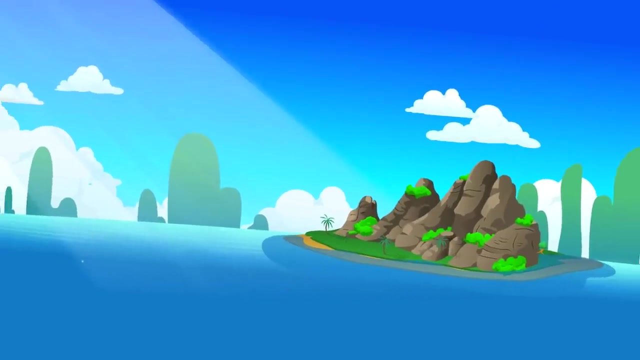 Subtitles by the Amaraorg community. speed and velocity. I think you and I should watch the airplane video: Vroom, vroom, vroom, Music. Airplanes. airplanes flying all around the sky. Airplanes, airplanes flying way up high. 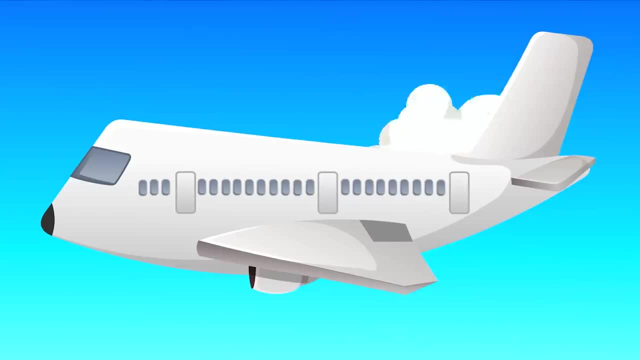 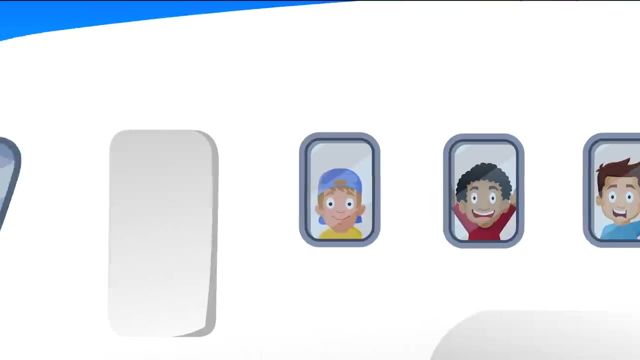 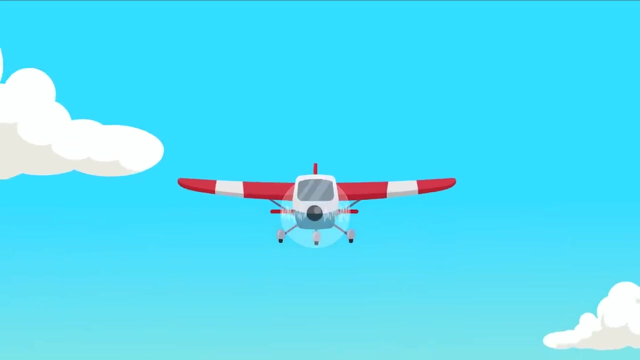 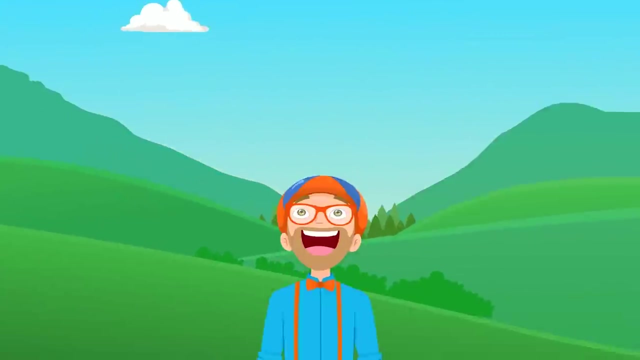 Music. Some airplanes are as big as a building. Some are as small as a car. That's amazing. Some airplanes transport people. Some fly near to the stars. That's four. Some airplanes fly with propellers. Some airplanes fly with jet engines. I love to look up and see their wings. 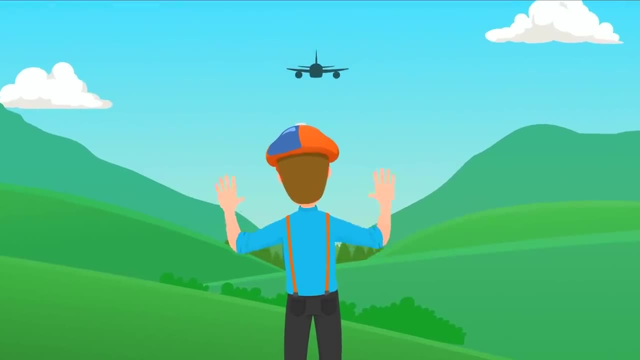 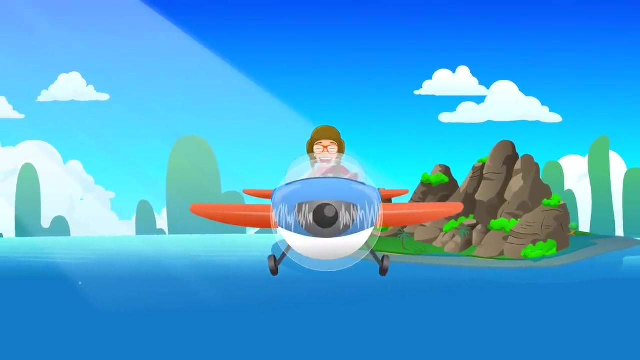 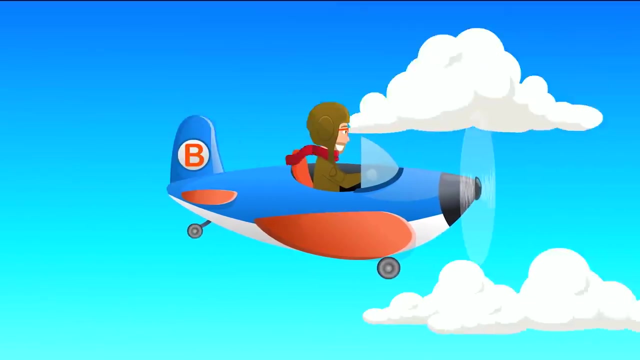 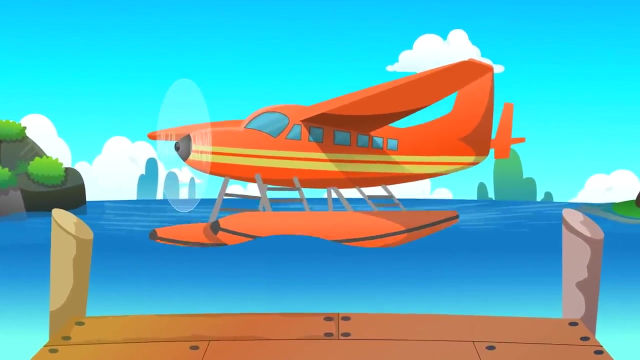 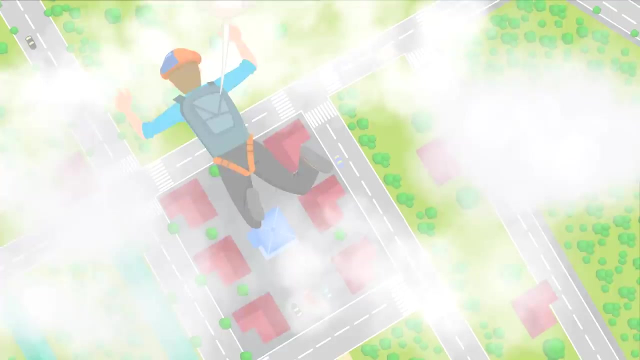 Waving down at me Music, Hey, airplane Airplanes, airplanes flying all around the sky. Airplanes, airplanes flying way up high. Some airplanes can land on water, But most land on landing strips- So versatile. Some airplanes fly just for fun, Some fly for business trips. 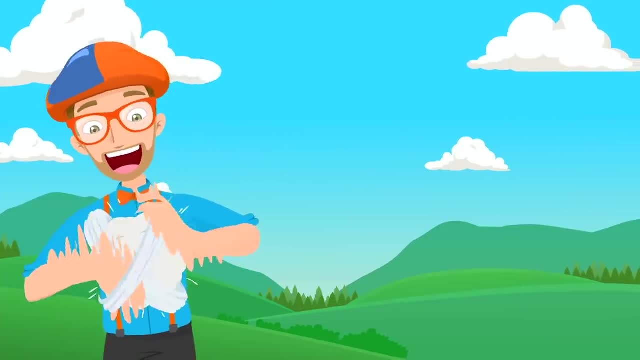 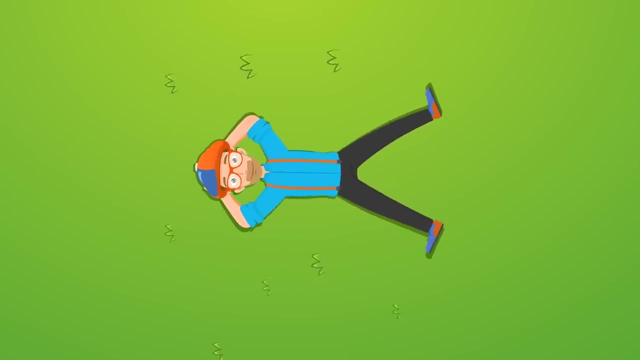 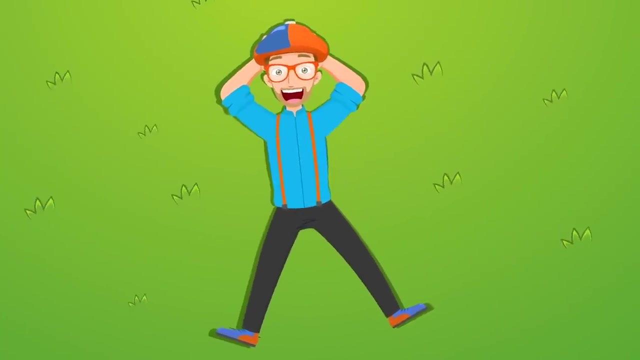 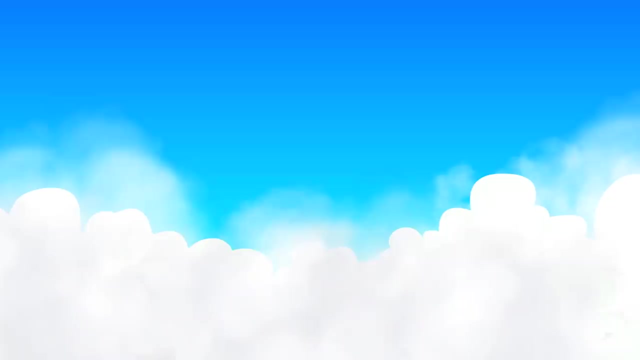 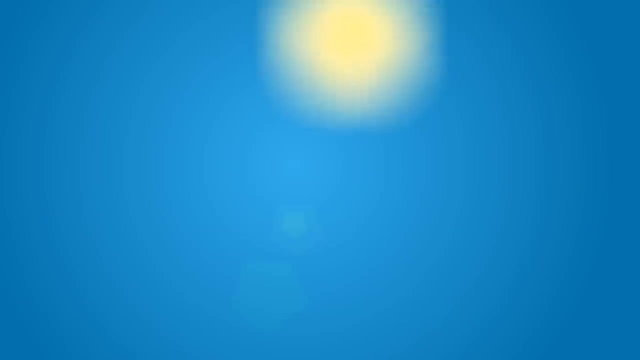 Business or pleasure. You can make an airplane out of paper, Throw it in the air and watch it go. I love to look up and see its wings Waving down at me. Hey, airplane, Airplanes, airplanes flying all around the sky, Airplanes, airplanes flying way up high. 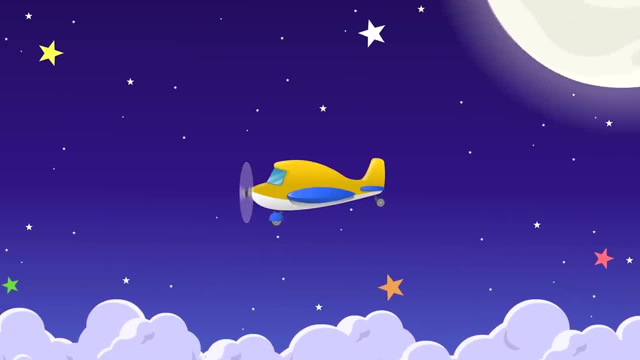 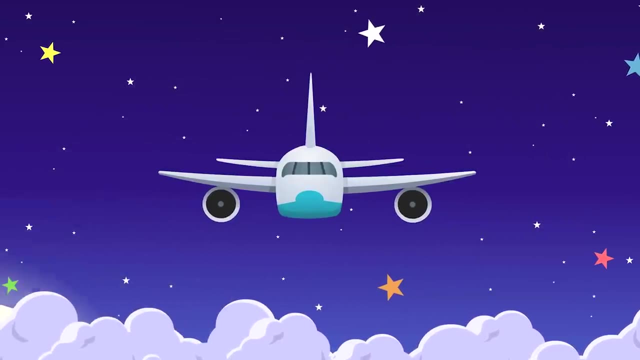 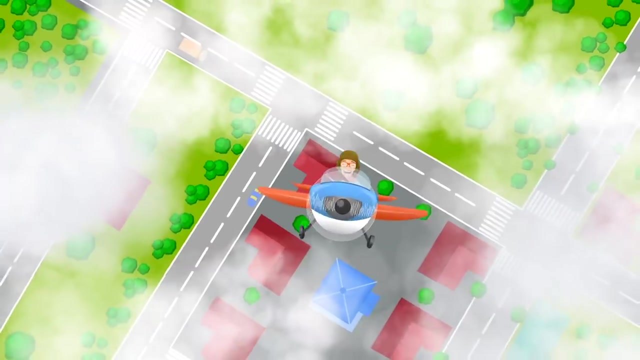 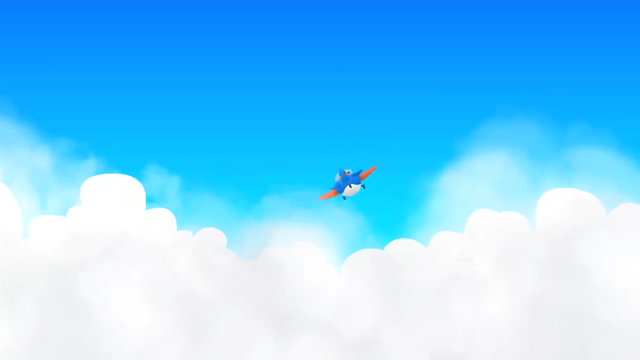 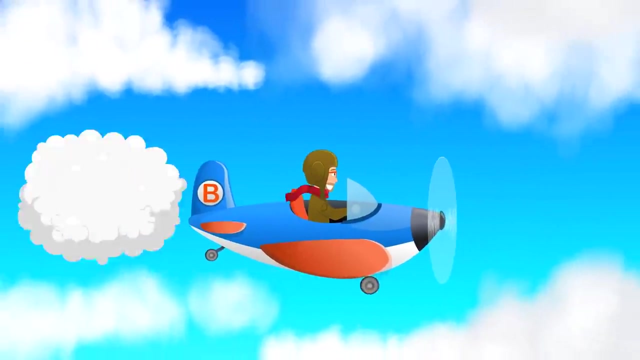 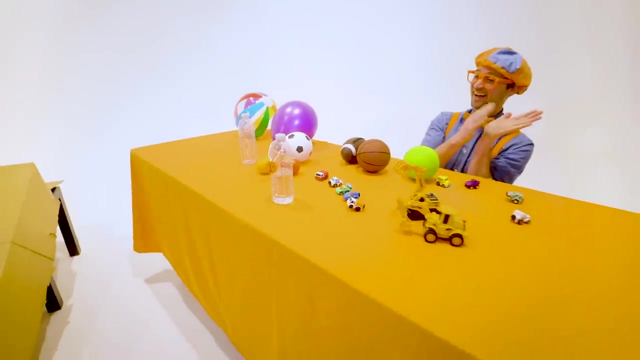 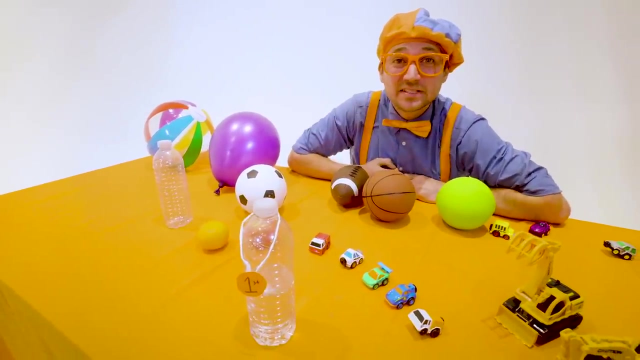 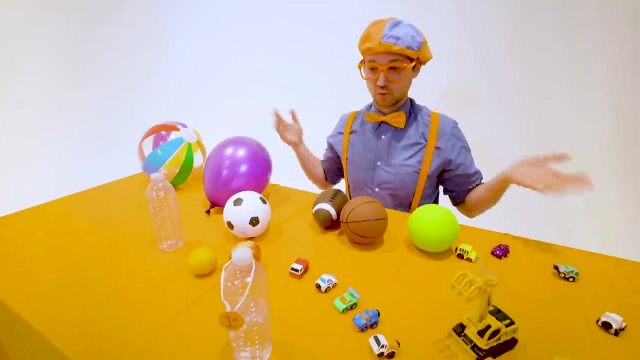 Music Airplanes. airplanes flying all around the sky Airplanes. airplanes flying way up high- Wow, Good job. Water Bottle. Wow, That was so much fun learning about velocity with you. It was really fun seeing all these great items compete at the great Blippi Velocity Race. 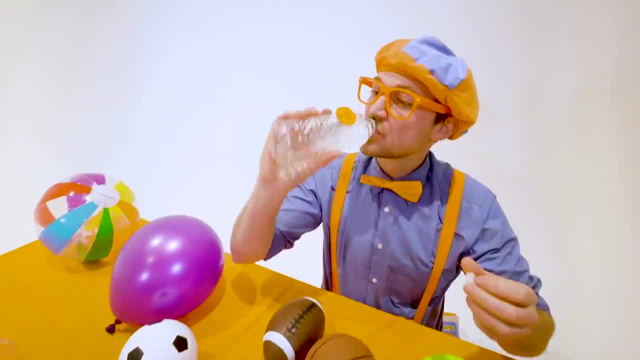 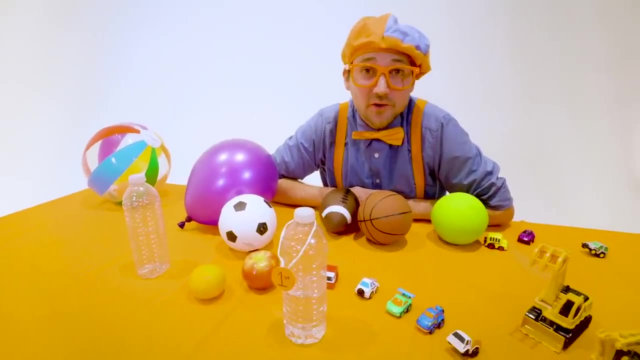 But there's only one champion, and today that was water. Wow. Well, this is the end of this video, But if you want to watch more of my videos, all you have to do is search for my name. Will you spell my name with me? 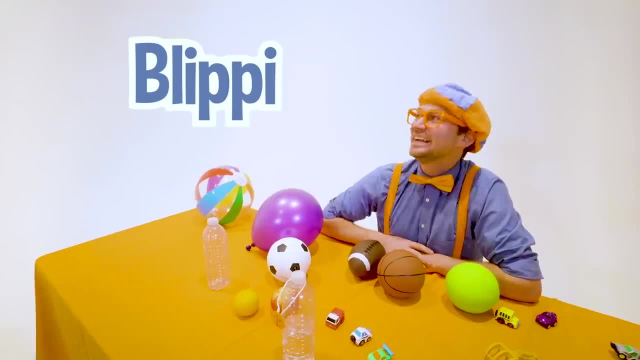 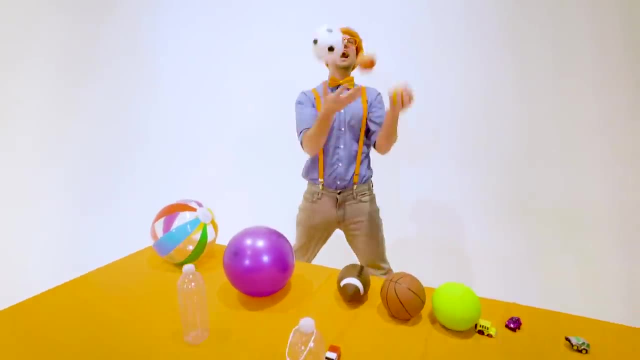 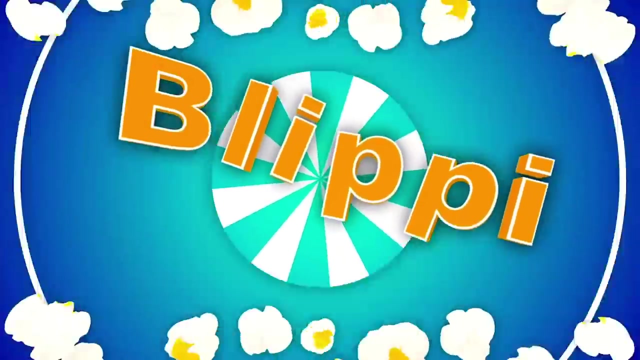 B-L-I-P-P-I. Blippi. Good job, All right, See you again. Bye-bye. So much to learn about. It'll make you want to shout: Blippi, Hello, Hey, it's me Blippi. 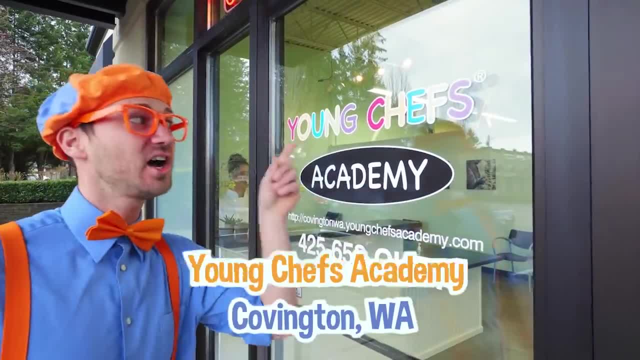 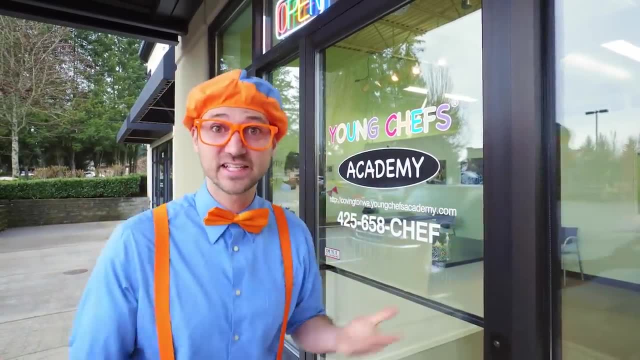 And look at where I'm at Whoa. Today I'm at Young Chefs Academy in Covington, Washington. This place is so cool, Yeah, where young chefs, kids just like me and young chefs are all together And young chefs like you can come here and learn to cook some delicious treats. 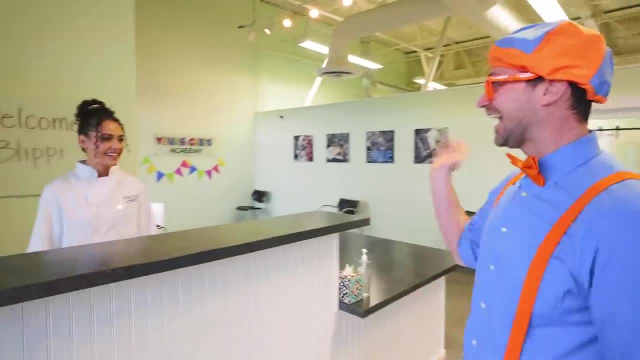 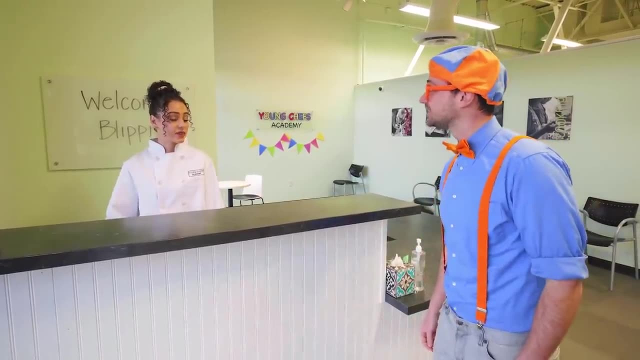 Let's go. Hi Blippi, Hey, who are you? My name's Chef Riley. Oh nice to meet you, Chef Riley. Hey, do you mind if we go explore the kitchen? Go for it. I'll see you in a sec. 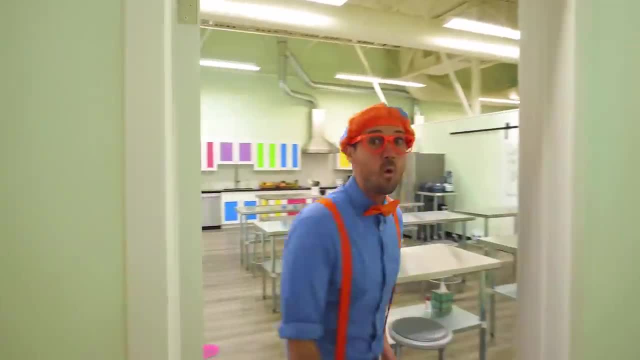 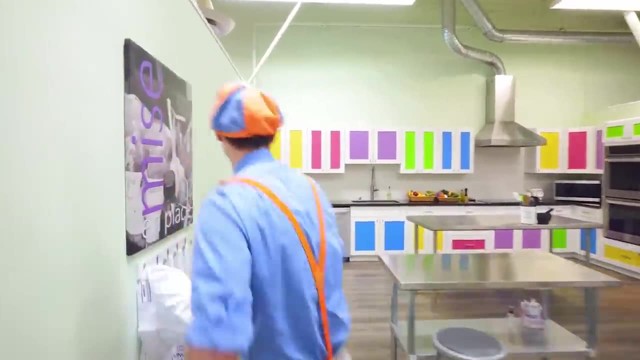 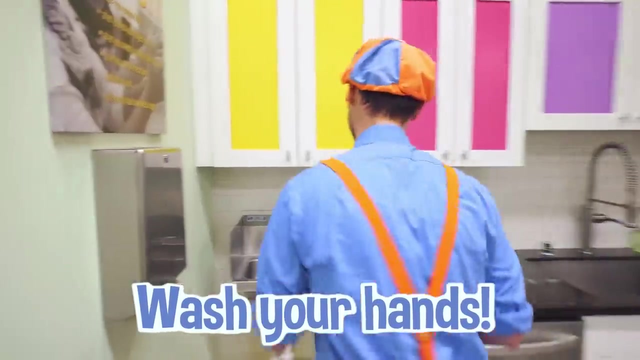 Okay, let's go. Wow, look at this kitchen. It is so bright and colorful. Whoa, come on. Okay, Okay, So the very first thing that I need to do when we enter a kitchen is wash our hands. Okay, I'm going to turn on the hot water and then I'm going to rinse them. 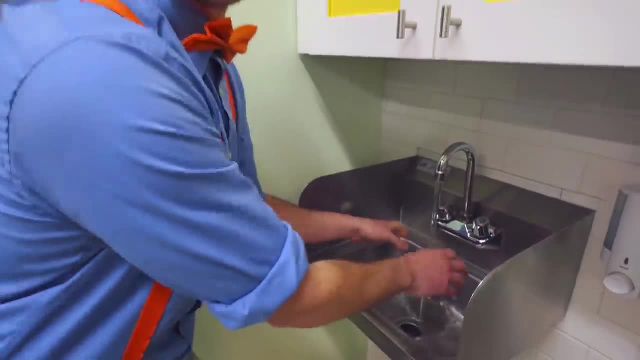 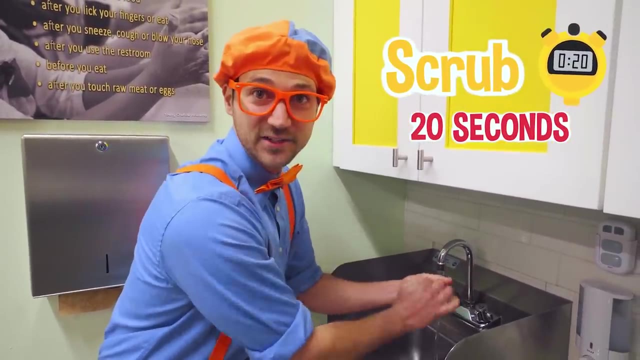 Okay, get them nice and moist. And then we need some soap, Okay, and we need to scrub for 20 seconds. And one way to do this is to sing the ABCs Ready: A, B, C, D, E, F, G. 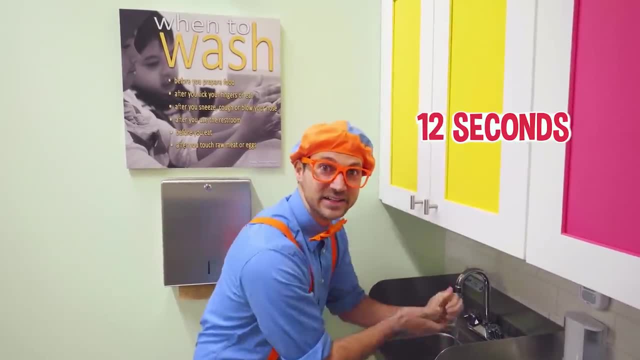 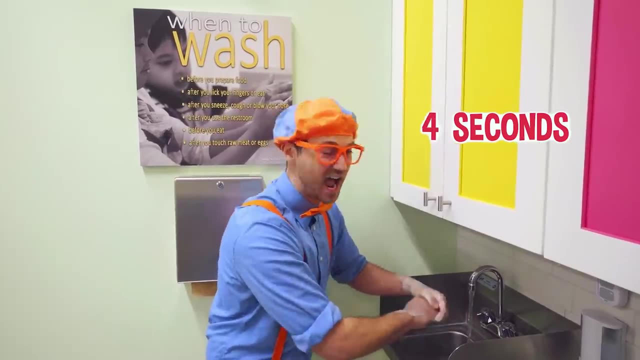 H, I, J, K, L, M, N, O, P, Q, R, S, T, U, V, W, X, Y and Z. Okay, now we're going to rinse off our hands. 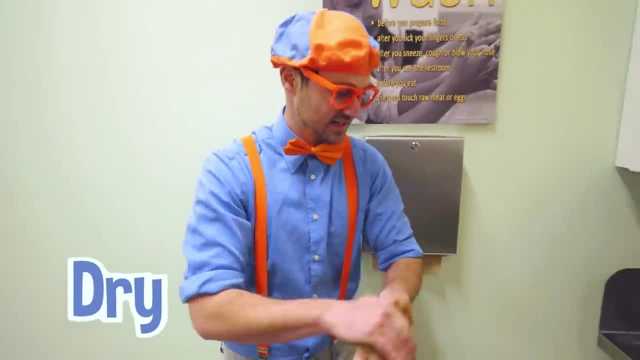 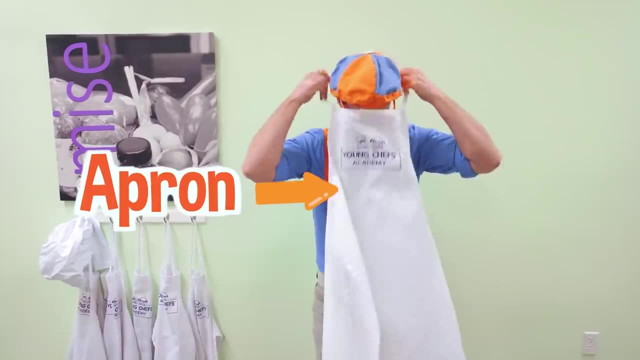 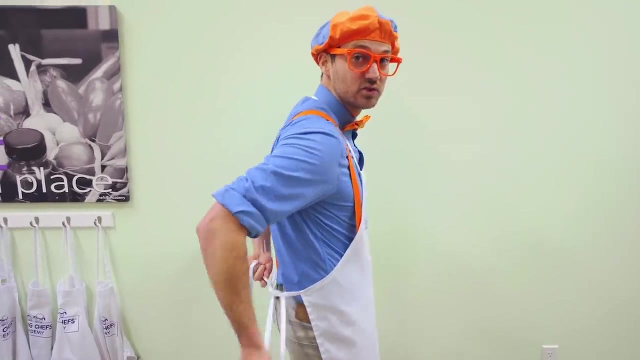 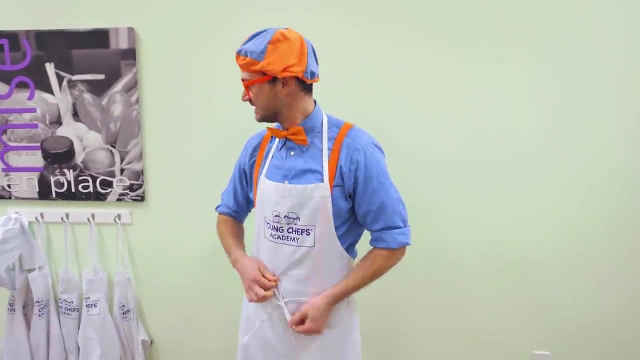 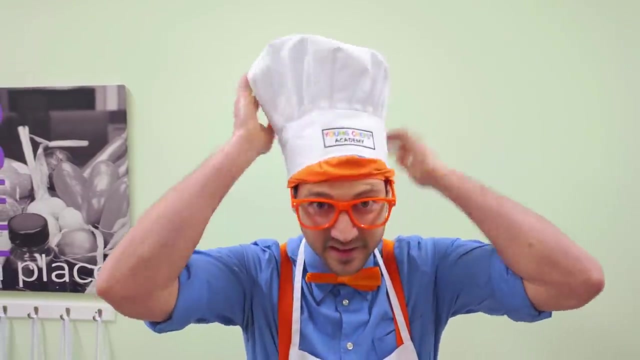 Get them nice and dry. Now, once our hands are dry, clean. Okay, Now I can put on an apron. Yeah, an apron is used. so then, clothes not get dirty when you're cooking with some food, All right, and I can't forget my young chef's academy chef's hat. 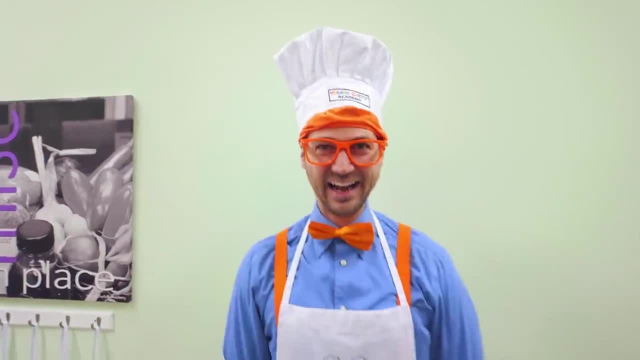 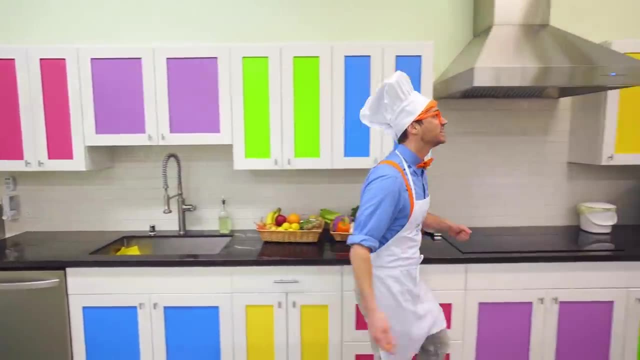 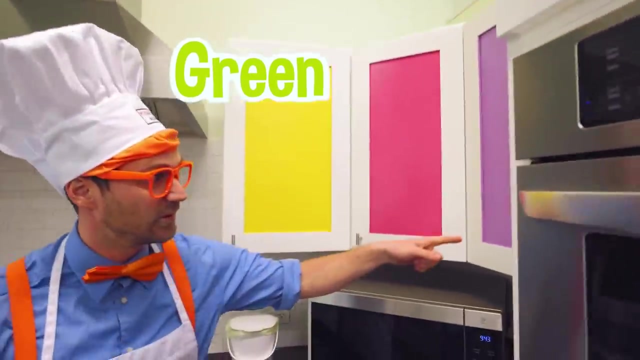 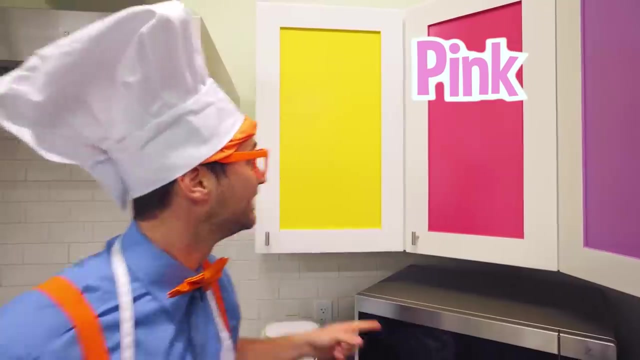 How do I look? All right, check it out. This kitchen is so cool, It's so colorful. Do you see? all these cabinets? Yeah, Whoa, These, yeah, are the color green. Ooh, this over here. yeah, that cabinet is purple, pink, yellow and blue. 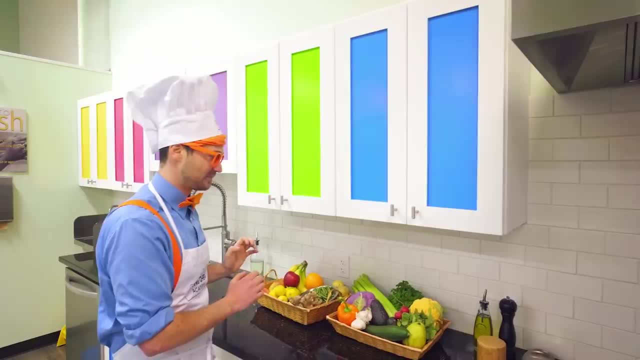 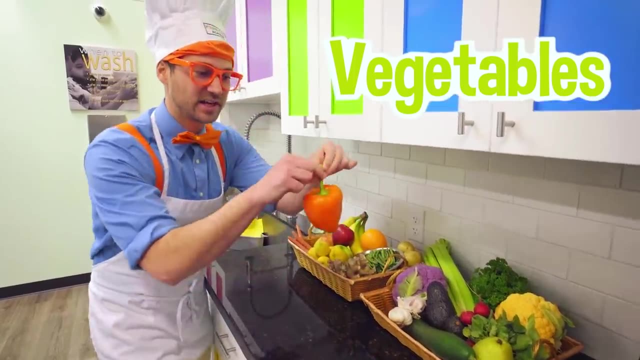 Whoa, I bet there's a lot of cool things in these cabinets. Whoa, Look at this- Some yummy vegetables. Hey, Do you know what kind of vegetable this is? Yeah, This is an orange pepper. Look at these. 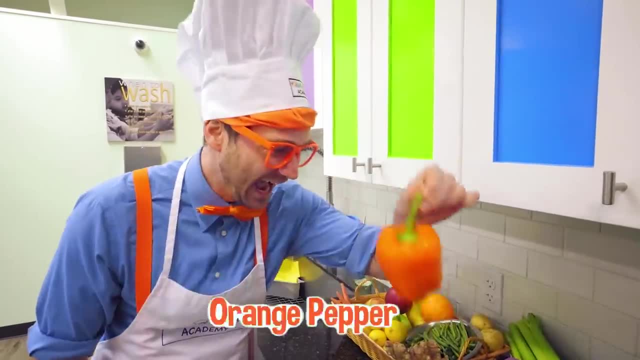 Yeah, some green beans. I sure do love vegetables. All right, I'm so excited. Whoa, I am so excited. This is going to be tasty. I am looking at the recipe of what we're going to be making today. 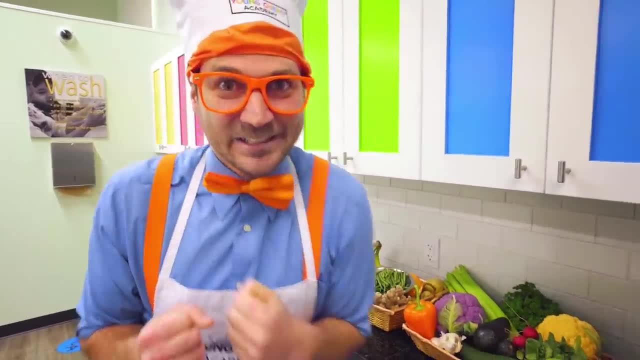 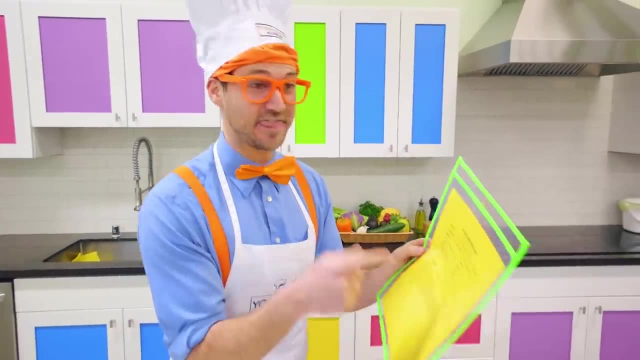 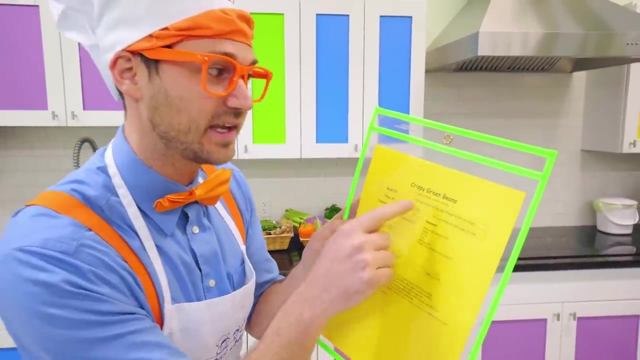 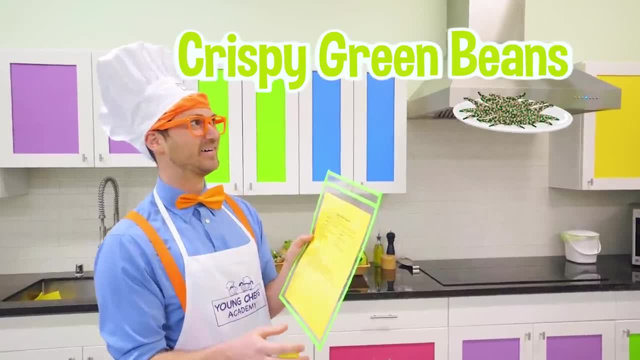 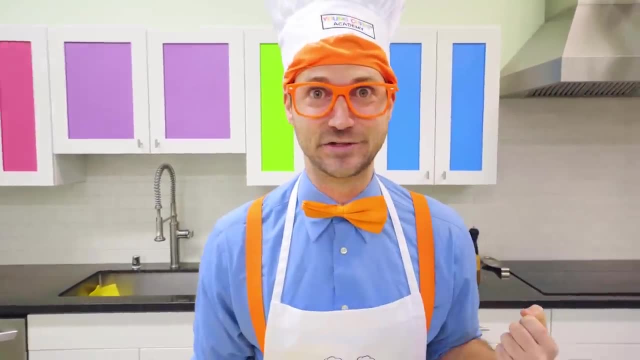 First, let's look at what we're going to be making today. Looks like we're going to be making crispy green beans- Whoa- Those look tasty- And creamy ranch dip. Oh, this is going to be so yummy and healthy. 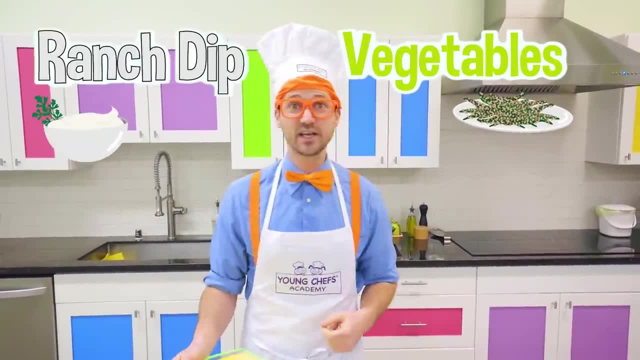 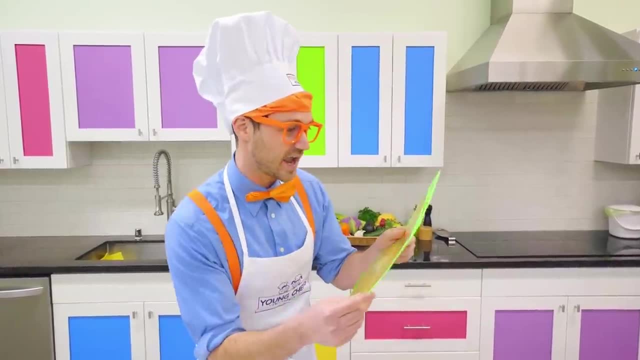 I love vegetables and I love ranch dip. I wonder if we're going to be able to dip the green beans into the ranch dip. Yeah, Okay, So it seems like we need a lot of tools and a lot of ingredients, Right? 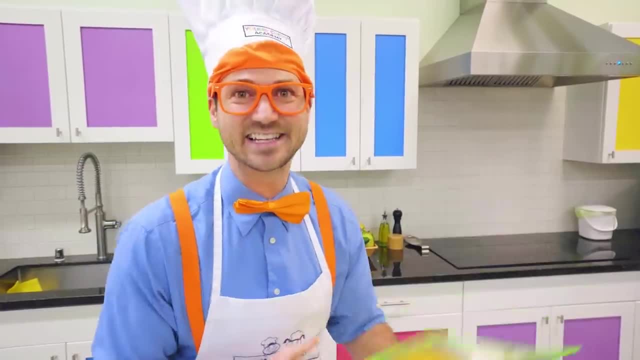 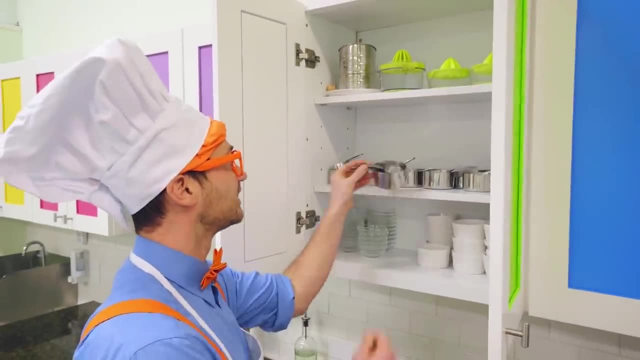 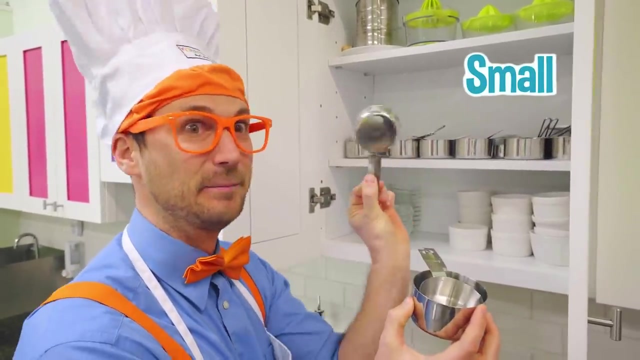 lot of ingredients. So, uh, let's get to it. All right, let's see what's in here that we need. Okay, looks like we need some measuring cups. Oh, a small one, a medium-sized one, another medium-sized one. 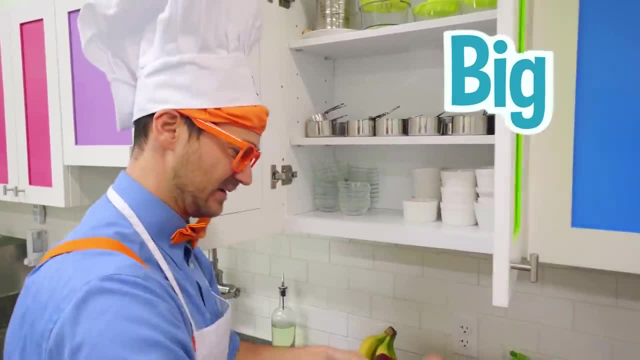 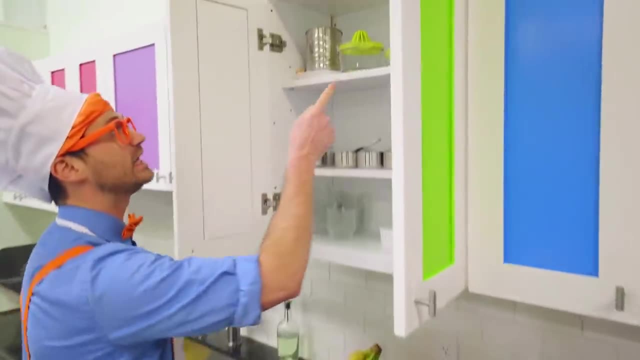 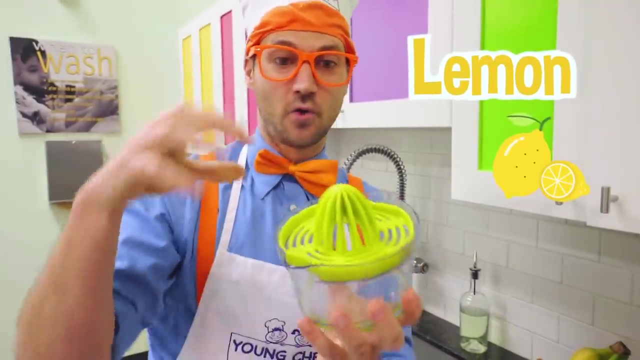 and a big one. Okay, Put those right back here. Perfect, Then we need a juicer. This is where you can put a lemon or an orange or a lime, squeeze it on top and then all the juice comes out. the. 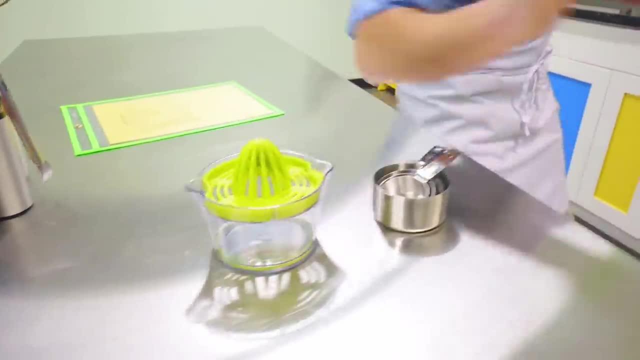 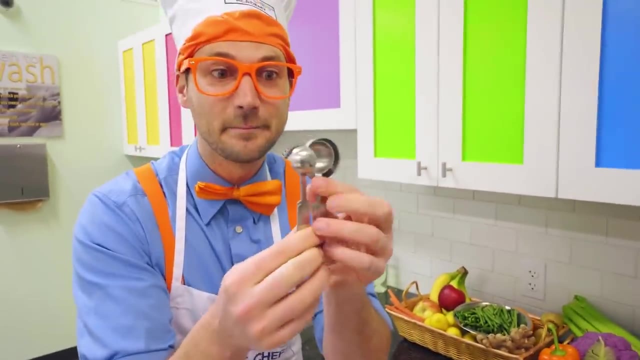 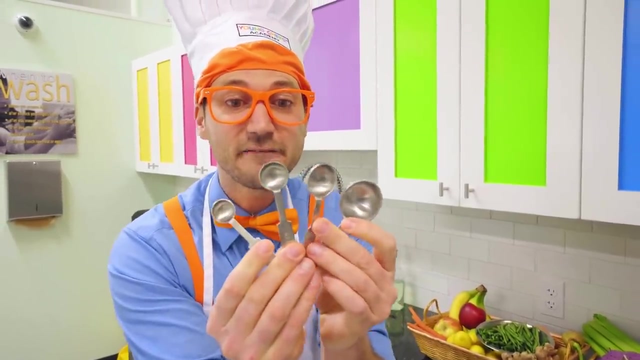 bottom. Okay, we'll set that down right there. Alrighty, let's see what's in here. Hmm, oh, we definitely need some measuring spoons. Whoa, yeah, same thing, just like the measuring cups: Measuring spoons of four different sizes. 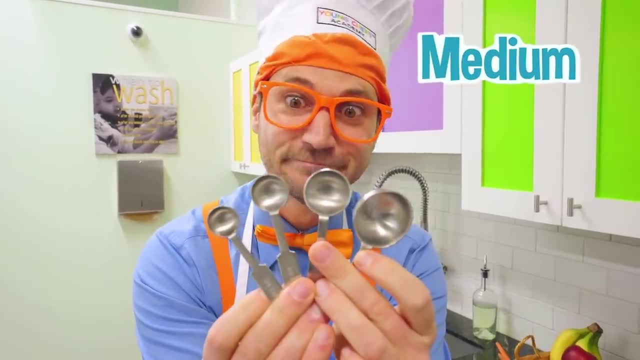 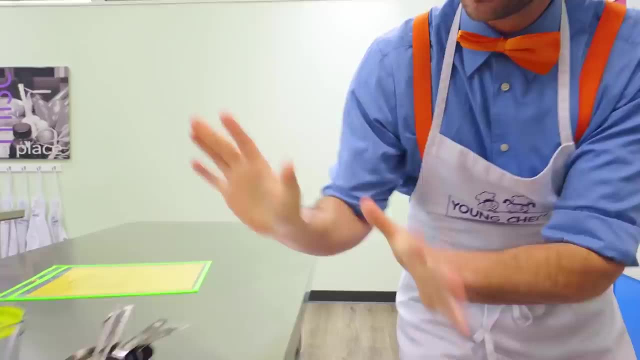 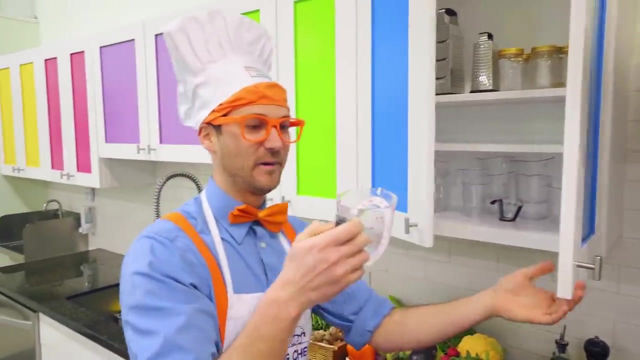 From small to medium to medium to large. Okay, put them right about right in there, Perfect, okay, let's see how about? oh wow, A measuring cup. This is what you put: liquids, and you could do solids. 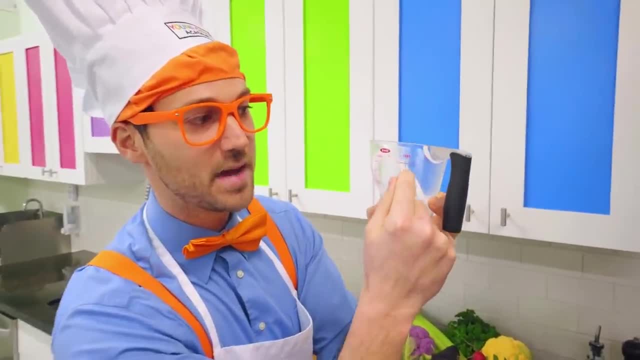 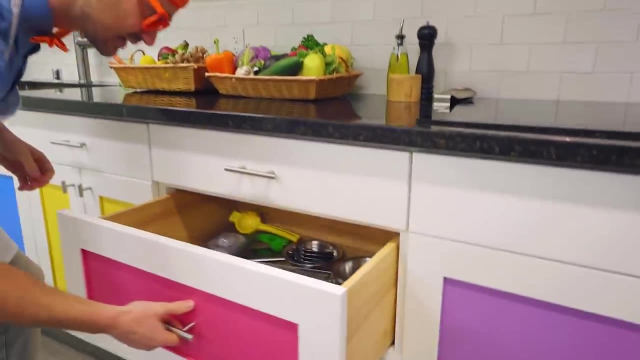 but this is primarily for liquids, And this is what you measure to see how much you have. Okay, put that down right there. Oh, let's see, is there anything in here? Hmm, there's a lot of cool things in here. 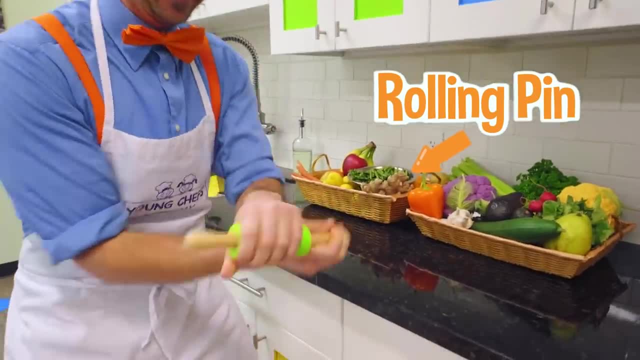 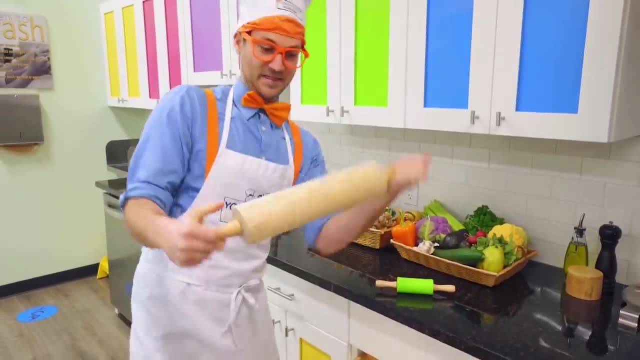 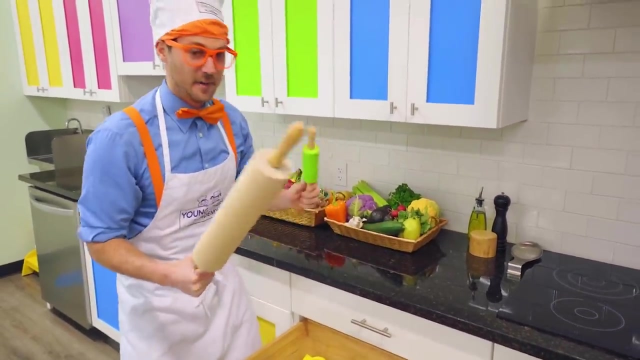 Whoa. look at this, it's a rolling pin. Oh, so cute. This is a small rolling pin Whoa. and this is a big rolling pin Whoa. they're used to flatten things out. I don't think we need those today. 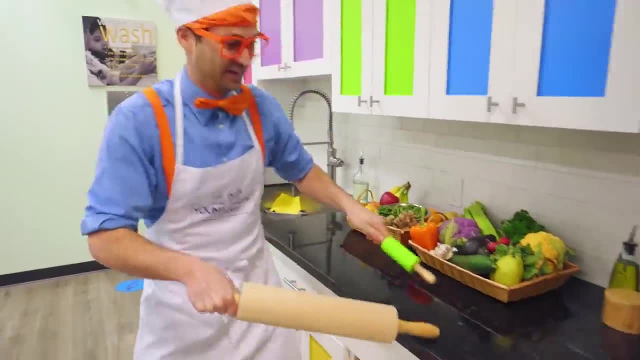 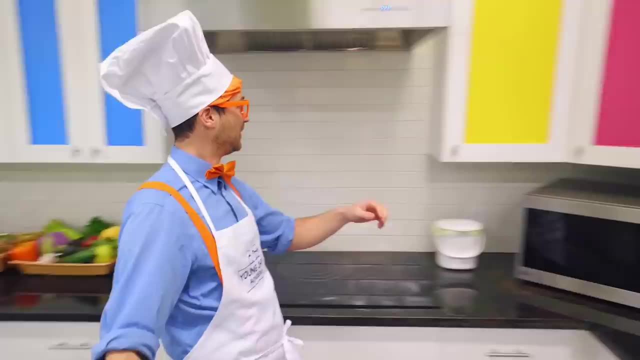 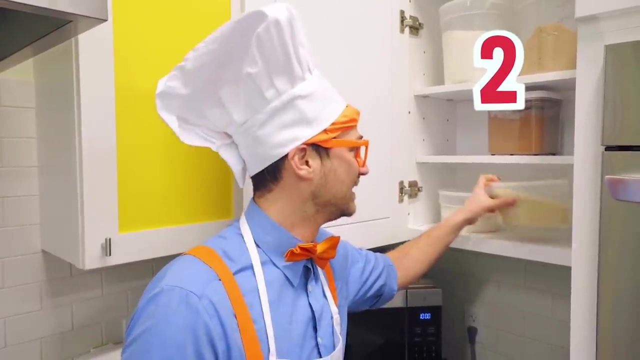 but they're pretty cool because you can use them for drums. Okay, enough playing, let's get to cooking. All right, let's see probably right in here. Oh yeah, two ingredients that we need: Breadcrumbs And flour. 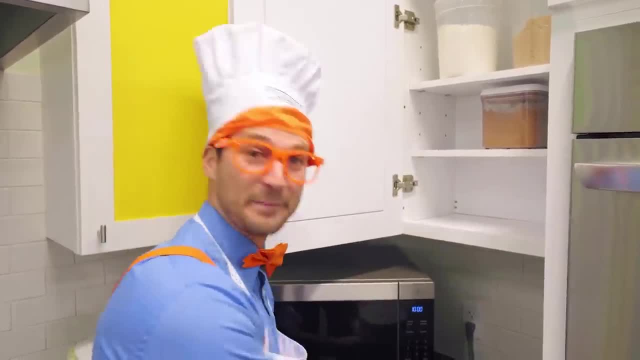 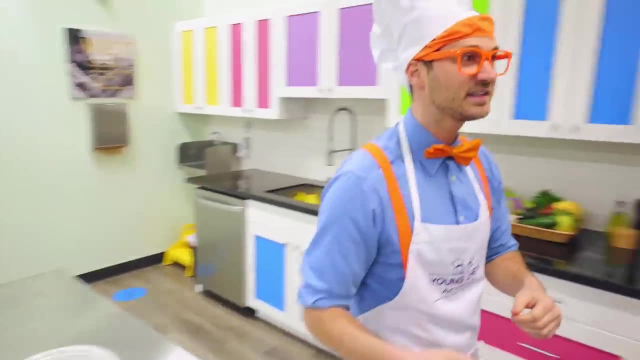 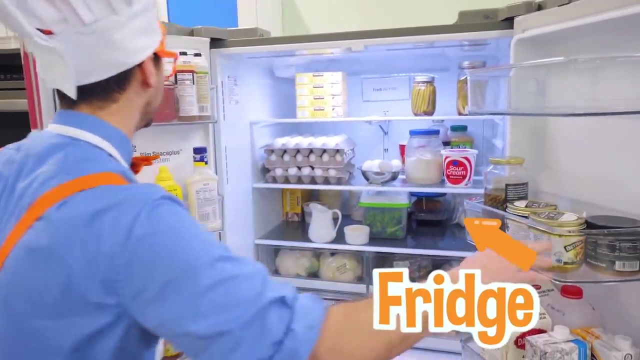 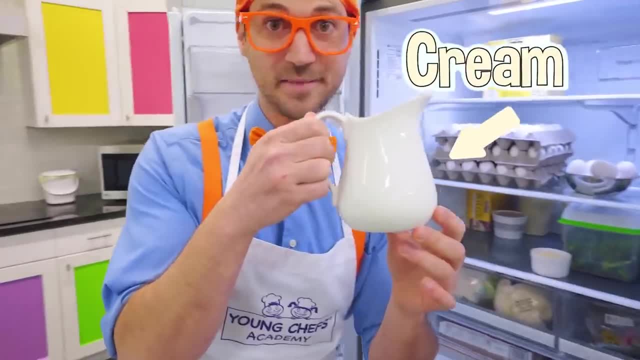 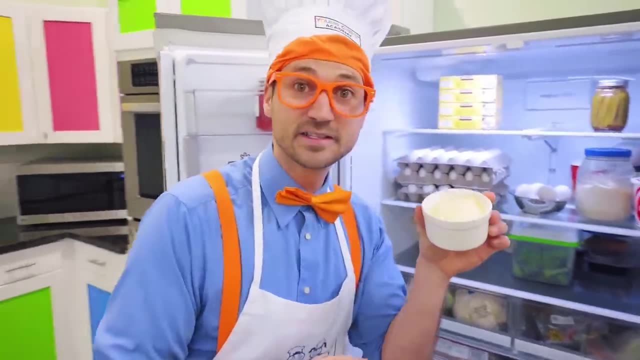 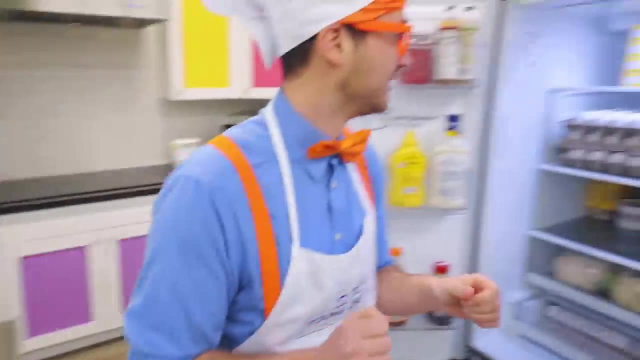 Okay, looks like we have some cream, probably for the ranch dip. We'll set that down right there. Ooh, some cheese, Parmesan cheese. Okay, we'll put that down right there. And then we have some eggs. Yeah, check this out. 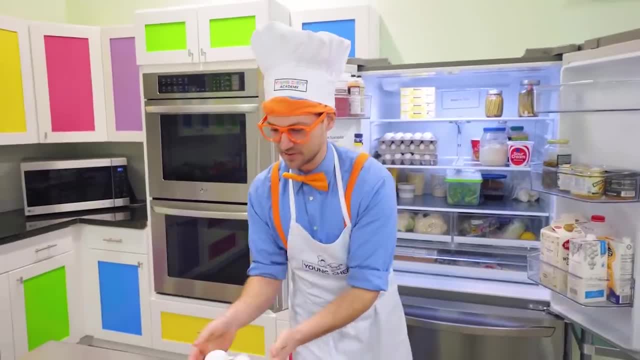 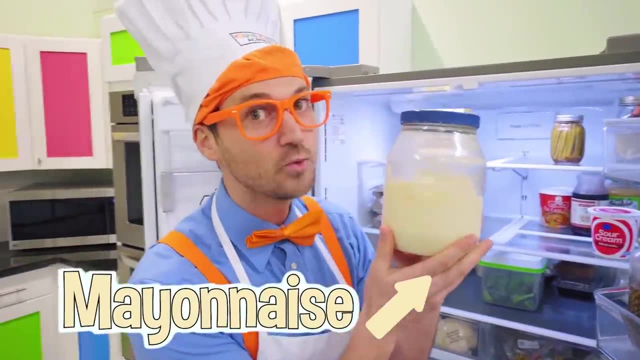 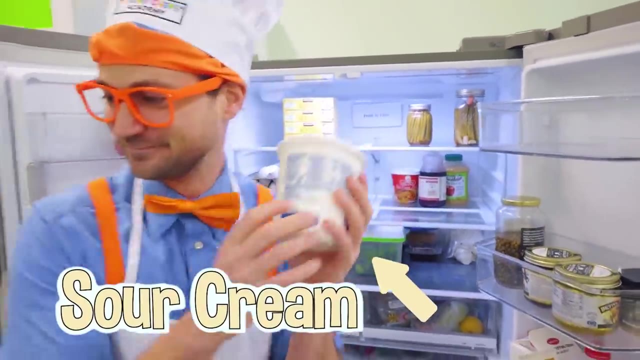 Whoa, whoa. Okay, we'll put those down right there for later. Probably shouldn't do that at home. And then we have some mayonnaise- Put that down right here. and some sour cream- Okay, put that down. and now I think we're ready. 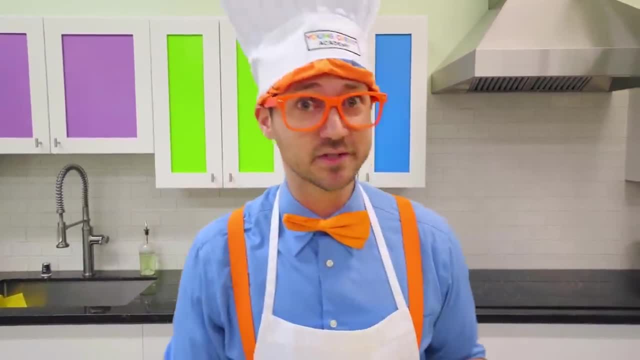 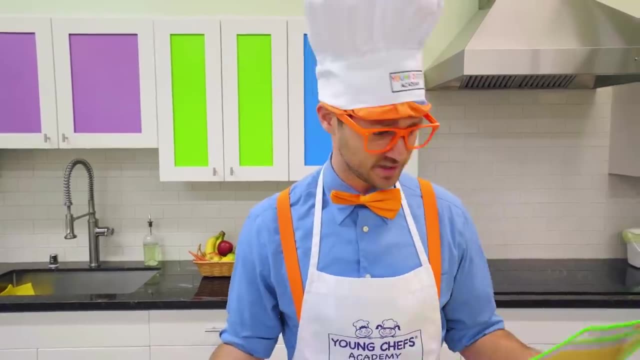 Looks like we have most of the ingredients and tools, but this looks really hard. Oh no, If only I had some help. Want some help with these? Oh sure, Hey Hi, I brought the rest of our ingredients that we need. 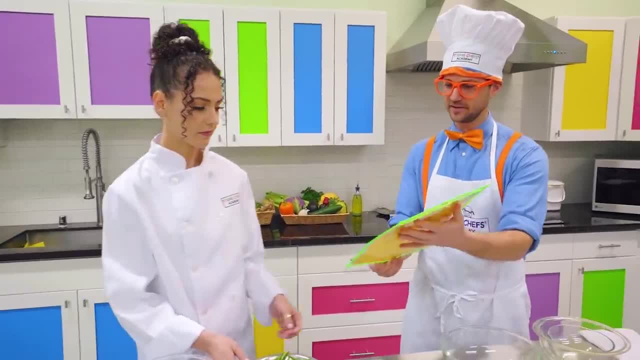 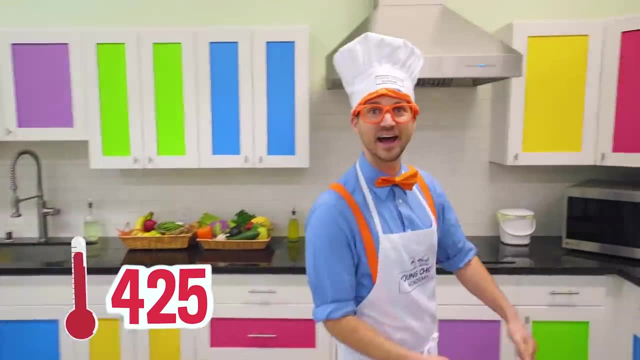 Oh, thank you, You're welcome. Oh, perfect, Okay, well, here's the recipe. What do we do first? First, we're gonna want to preheat the oven to 425.. Okay, Uh, I know how to do that. 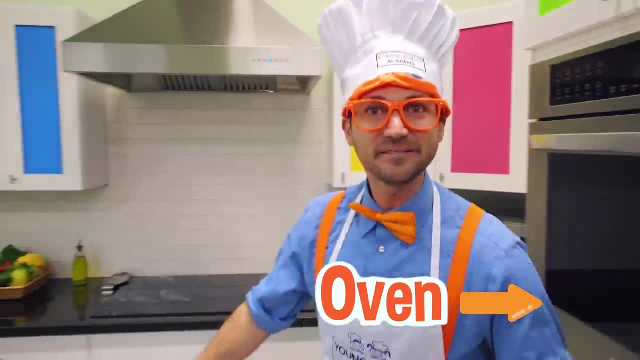 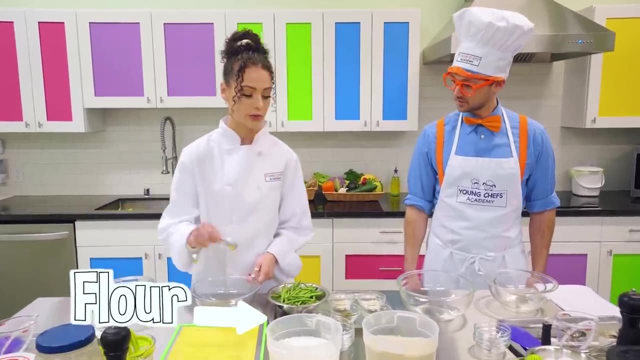 Okay, preheat the oven to 425.. Perfect, Good job, Whoopi. Thank you All. right, first we're gonna want to do a tablespoon of flour into our bowl. Okay, We're gonna want to make sure that we get a true tablespoon. 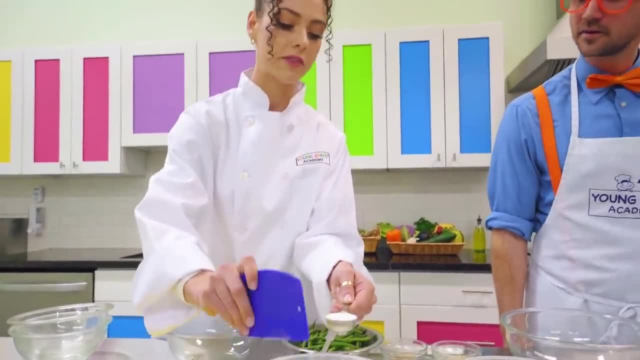 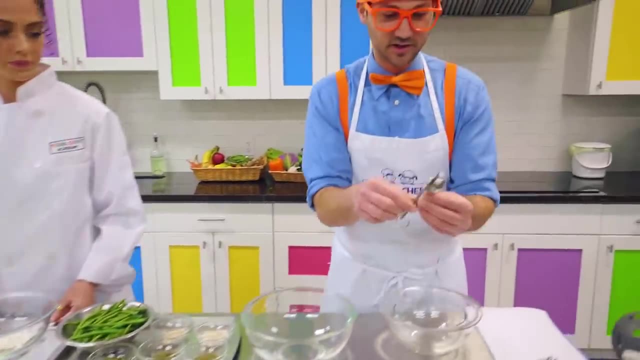 because that is not accurate. So we want to scrape off the extra flour. Okay, Okay, can you do that? Sure, Okay, Looks like we need some flour. Let's do a little scoop And there we go And perfect. 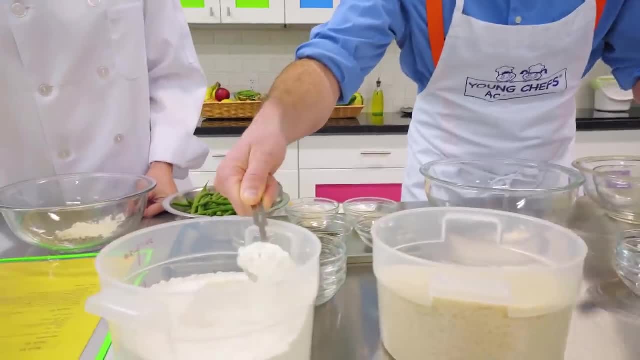 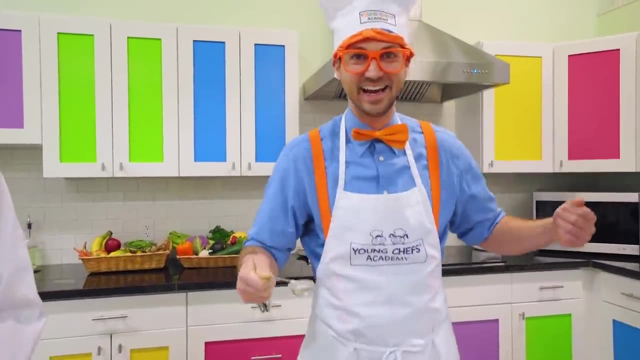 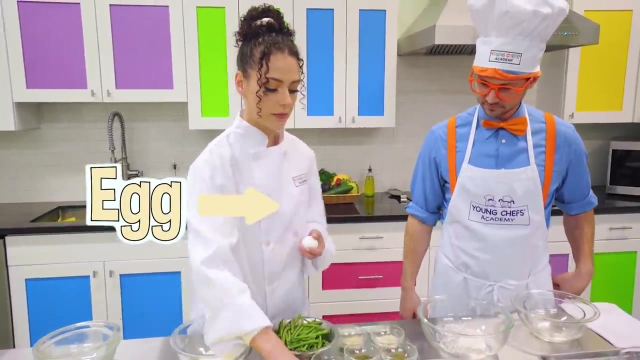 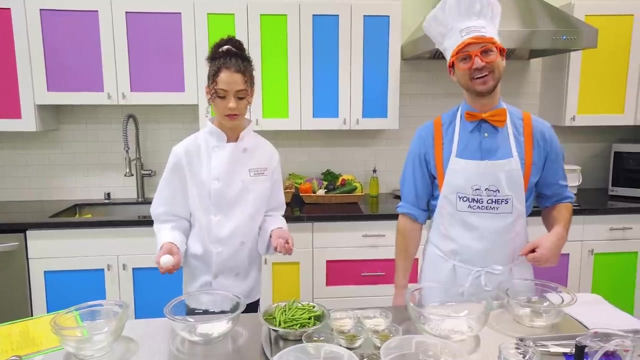 Great job, Whoopi. Thank you All right. Next we're gonna want to crack an egg. Okay, See. so at Young Chefs Academy, we crack an egg using the table, not the edge of the counter, So that it doesn't get all over the floor if you miss. 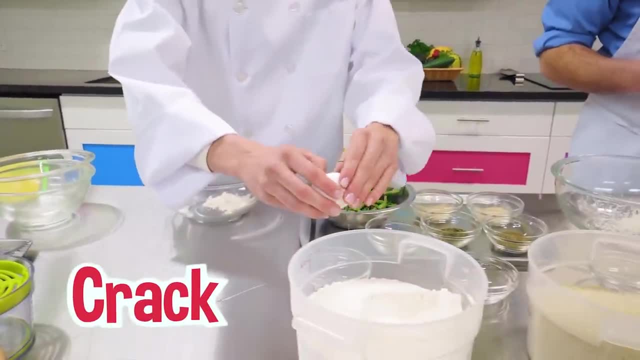 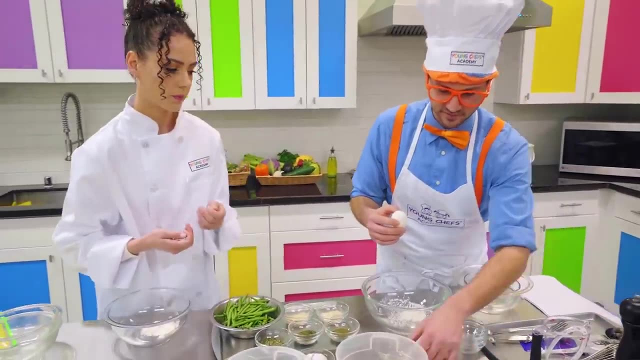 Okay, You want to crack hard and use your thumbs to break open the egg, Just like that. Perfect. You don't want to put the shell in a separate bowl? Okay, Here we go. Let's use the table. There we go. 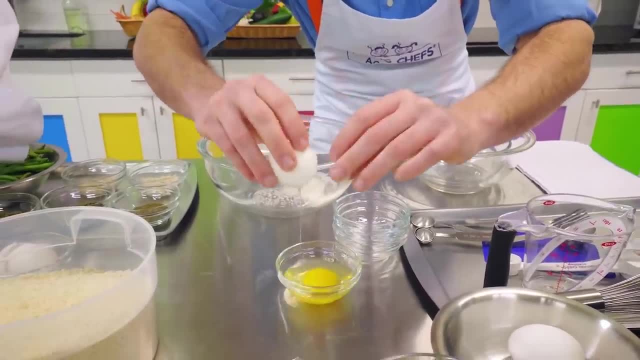 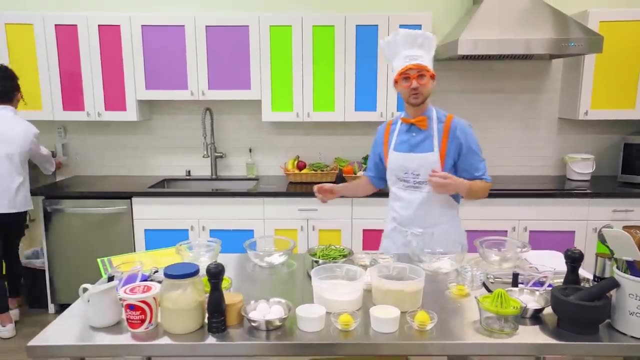 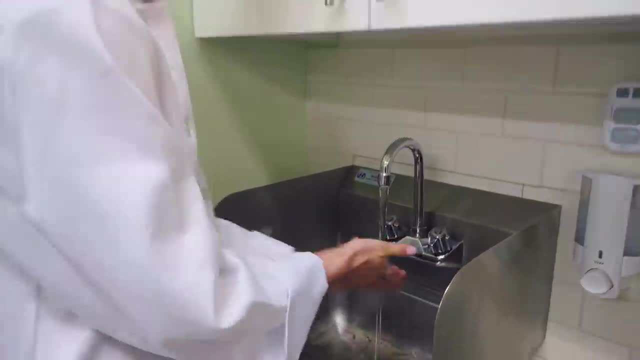 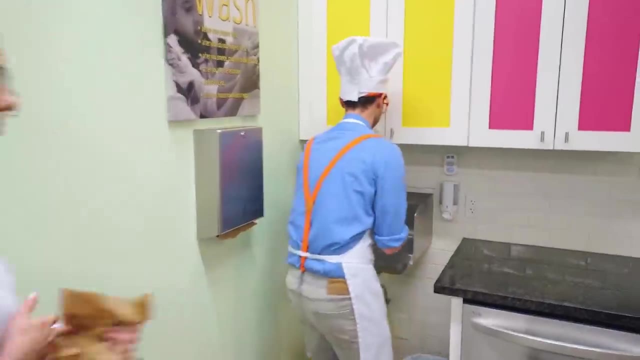 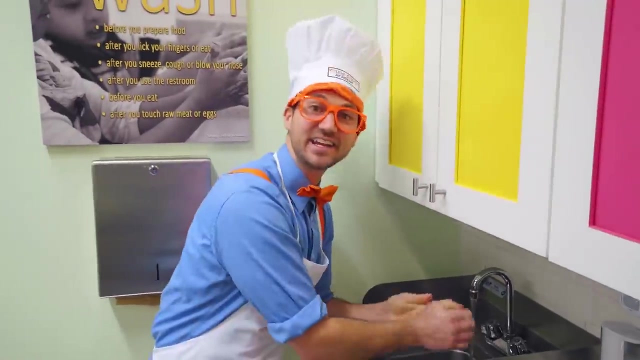 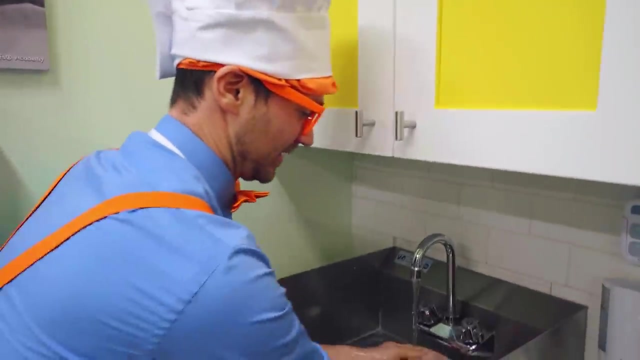 All right, Here we go, There we go. All right, All right, There we go, Let's rinse them off. Alright, There we go, Let's rinse them off. It's really important to rinse off your hands and wash them, enough or otherwise. 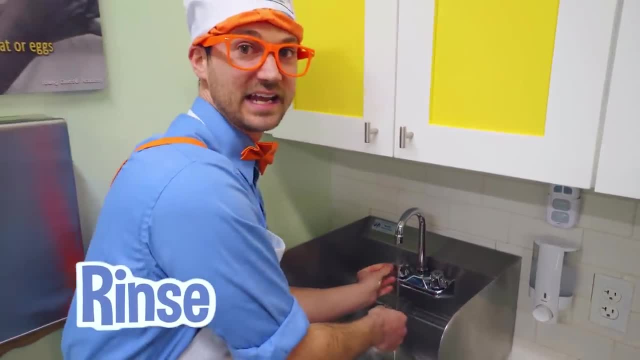 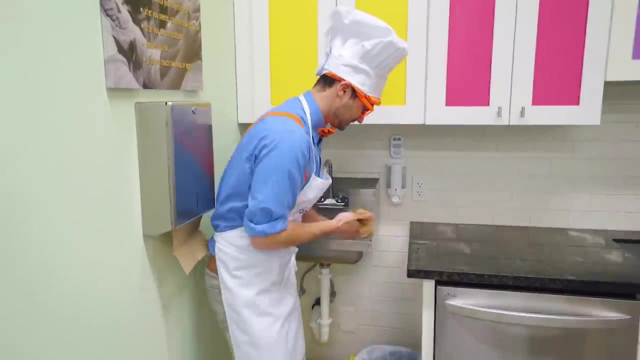 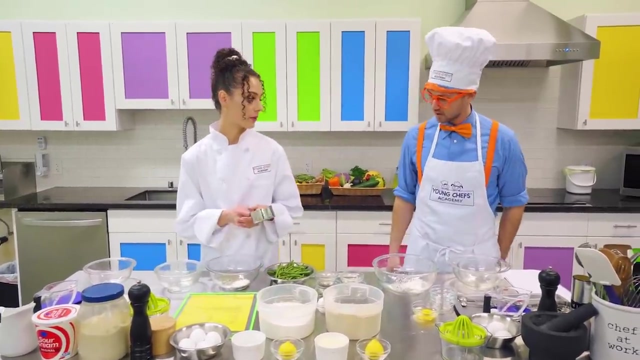 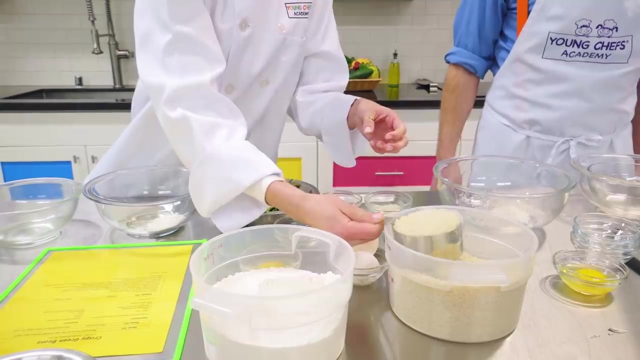 All right hands and wash them completely after touching raw eggs or meat or anything like that. now we're ready. okay, all right. next we're going to want to do a cup of panko. okay, so this looks about right. yeah, it says panko, just like breadcrumbs. it is. it's dried breadcrumb, okay. 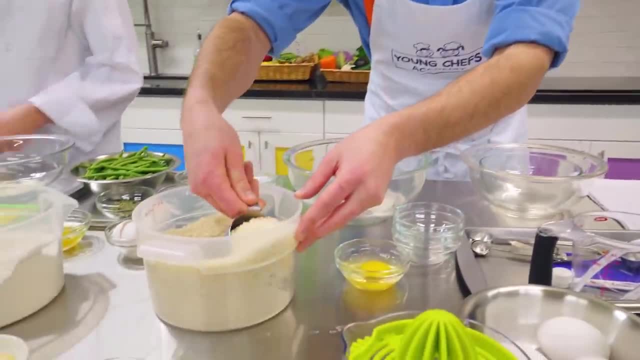 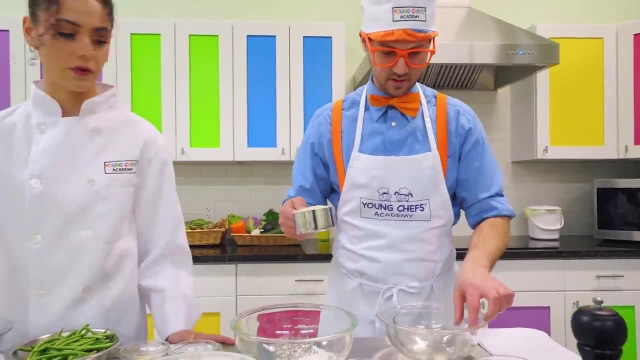 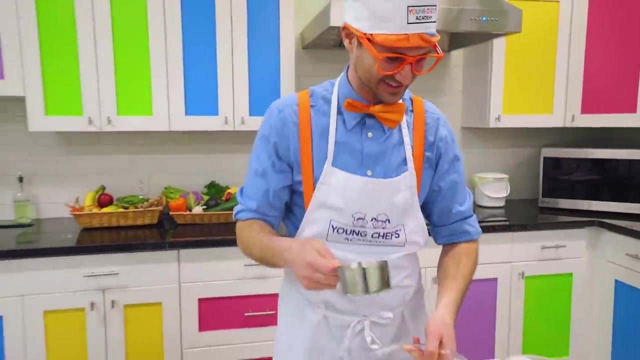 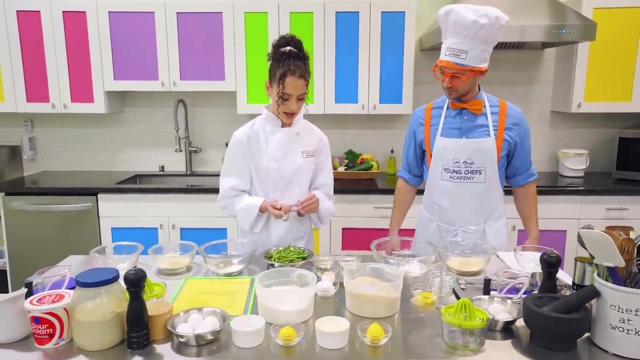 all right. oh, let's use that one big scoop, all right, in the same bowl. yeah, oh, so sorry, in a different bowl. oh, okay, oh, thank you. okay, here we go, perfect, all right. next, we're going to want to add the rest of our spices, which is garlic, salt and salt. okay, so we're going to want to use a tea. 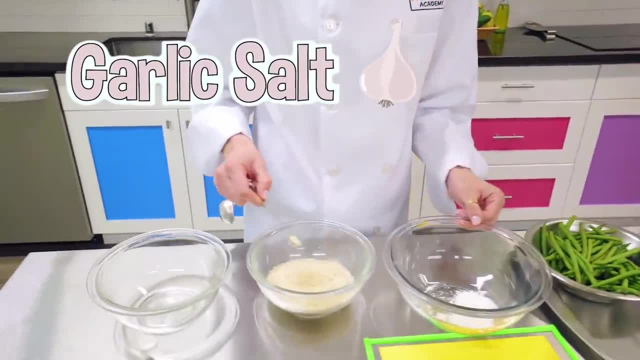 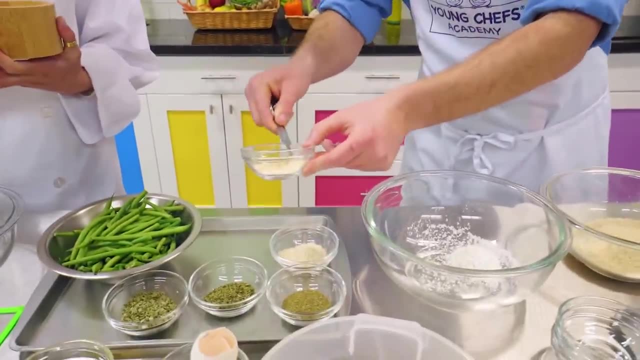 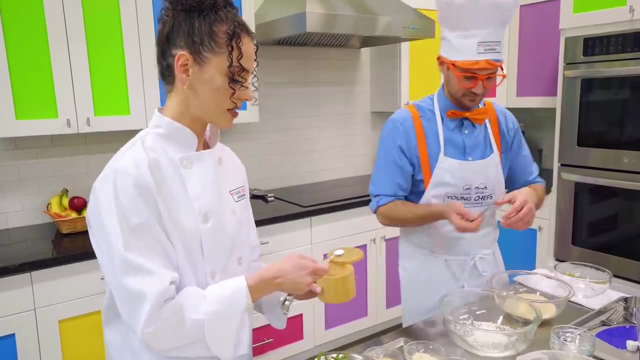 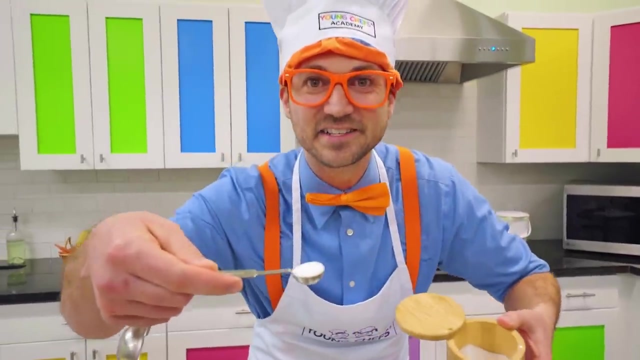 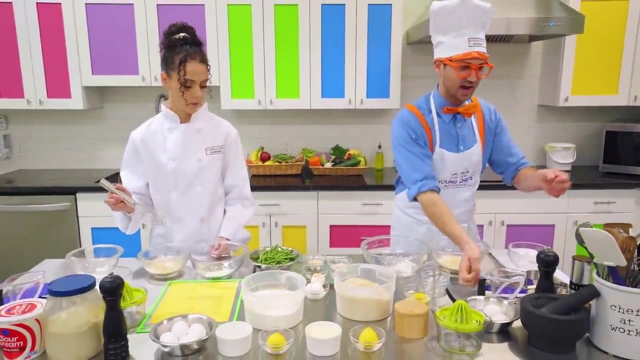 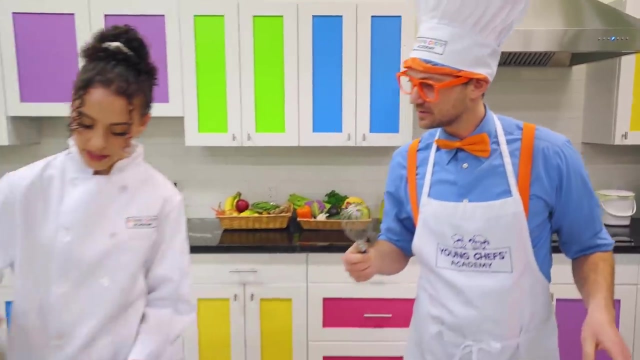 spoon of garlic salt in our panko. okay, here we go, this one. okay, let's put it in the panko, perfect, and then half of a teaspoon of salt. thank you, wow, salt is so yummy. here we go. can you use your whisk and whisk that up? yeah, check it out, this is a whisk. yeah, how do you do it? whisk with your wrist. 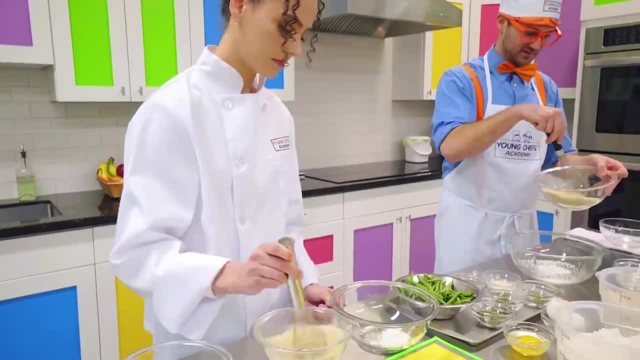 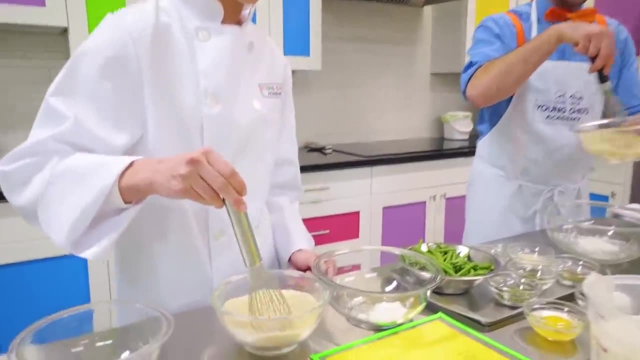 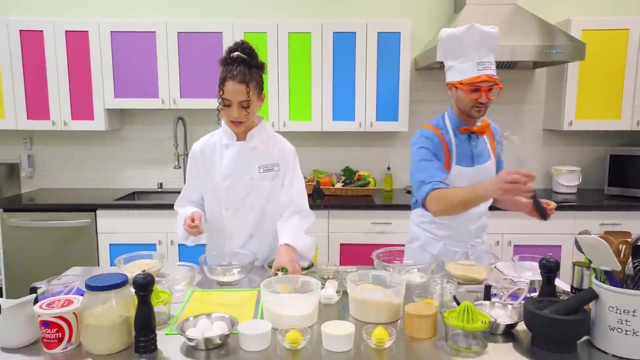 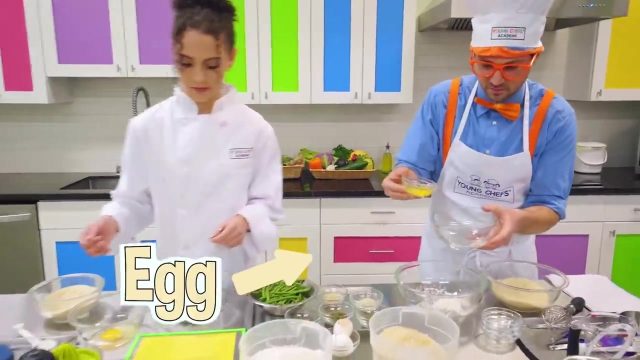 okay, oh, this is a really good way to mix it all up. yeah, you want to use it like that, all right. next, we're going to want to put our egg into this mixing bowl, the clean mixing bowl that we have. okay, here we go, put the egg in this bowl. 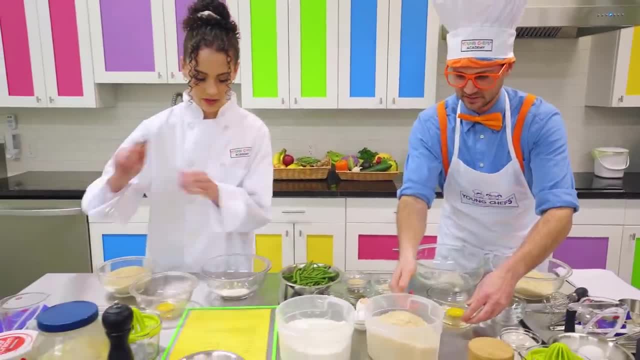 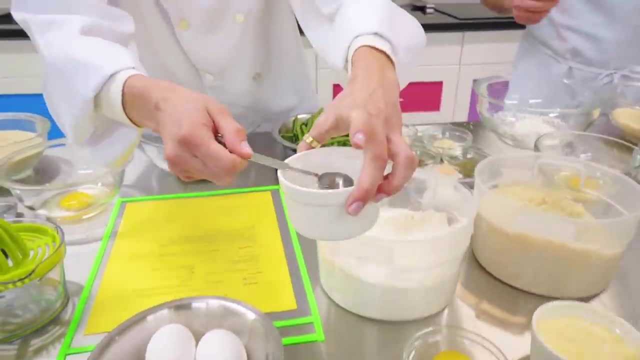 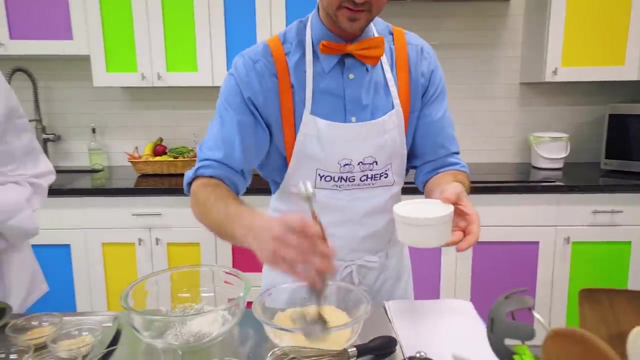 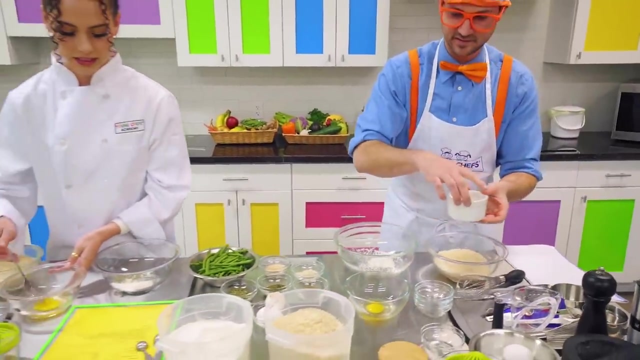 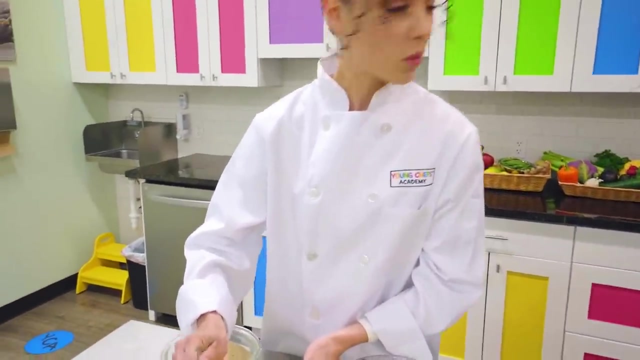 all right, and we're going to want to use a little bit of water like this in with the egg. perfect, thank you. all right, put some water in with the egg. perfect, can you whisk that egg up with the fork? for me, with the fork, forks are easier to whisk eggs than a whisk is. oh, you want to whisk it just like that, okay, so. 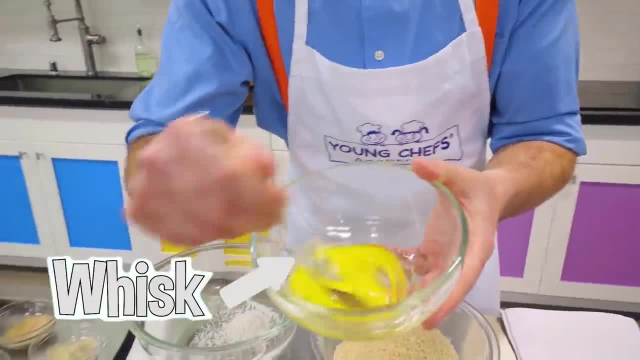 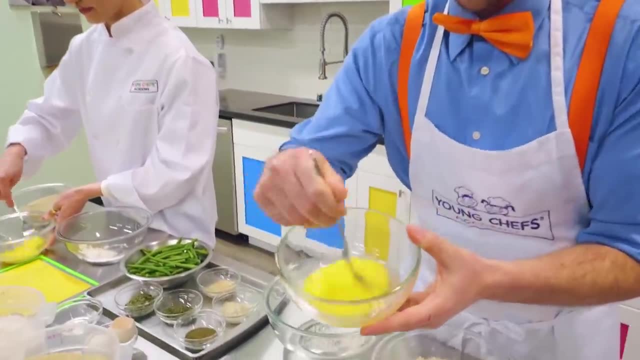 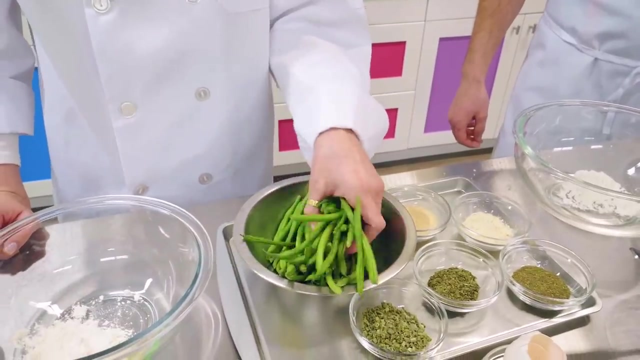 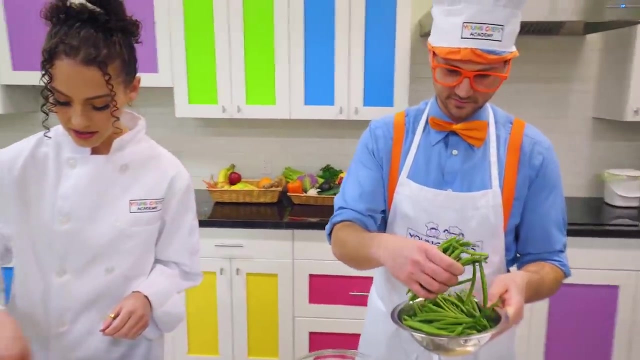 let's take the fork and let's whisk the egg. whoa, did you see how the yolk broke up? and now it's all mixed up. perfect, that's perfect, perfect. we're gonna grab a couple handfuls of green beans right in here, okay, all right, perfect, and toss it in our flour. all right, make sure you get them all nice and 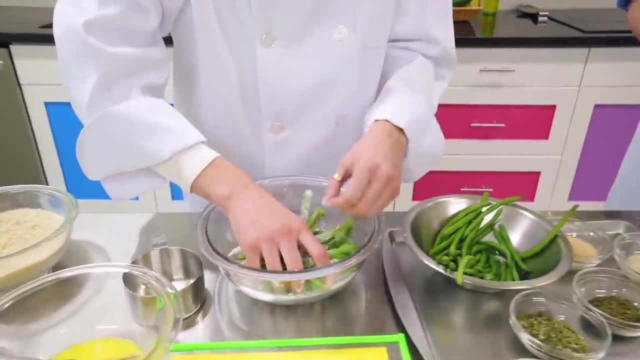 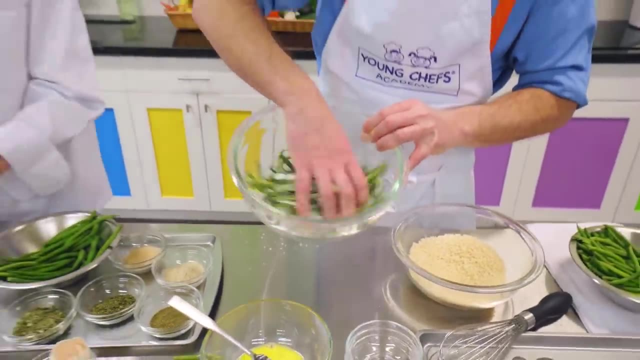 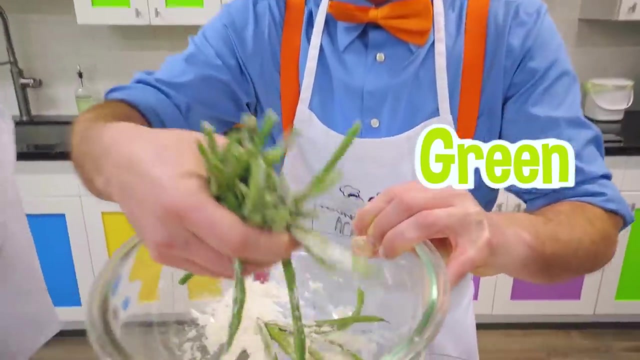 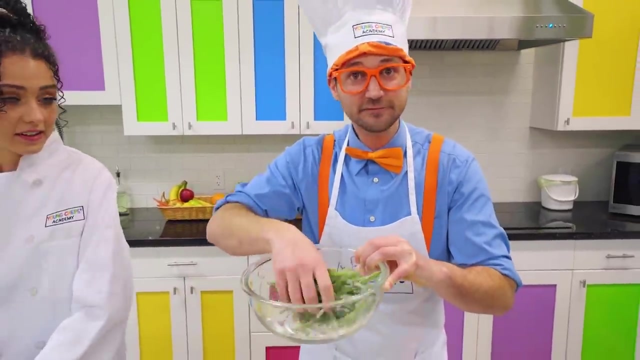 mixed up and coated in flour. okay, toss it. wow, this is gonna help the egg stick to the green bean. okay, interesting, look, it used to be green, but now the green and white. hey, remember how we washed our hands? yeah, good thing we did, because i'm touching food with my hands. you don't want to touch anything after you touch egg or raw meat. 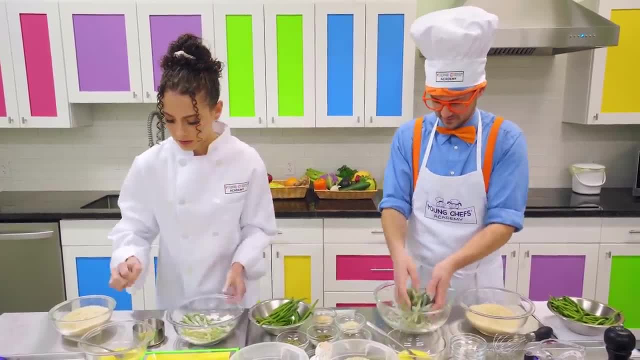 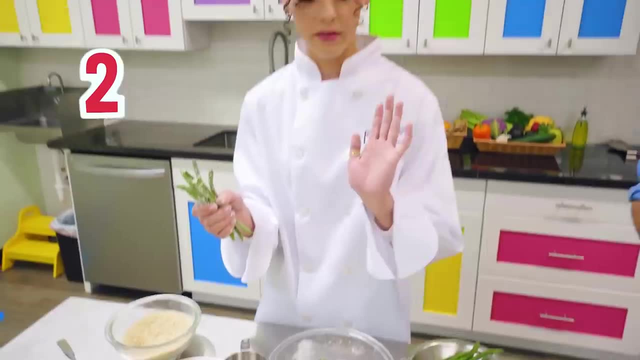 you want to make sure you wash your hands? okay, all right, now we are going to touch the egg, we're gonna put the green beans, we're gonna use two different hands. we're gonna have our dry hand and our wet hand. so we're not going to touch the egg with this hand. 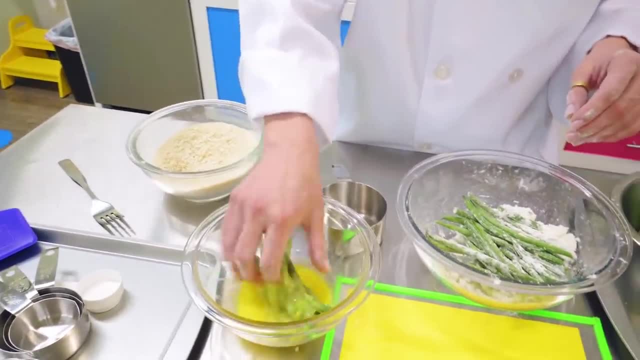 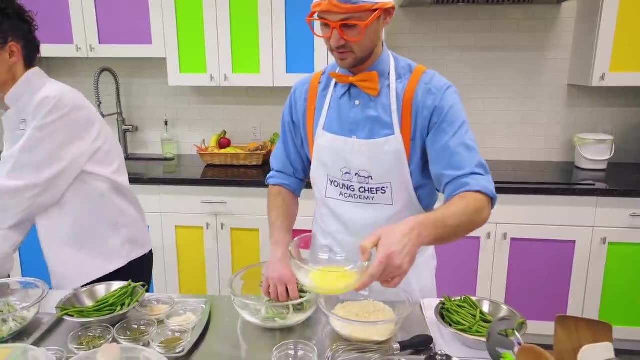 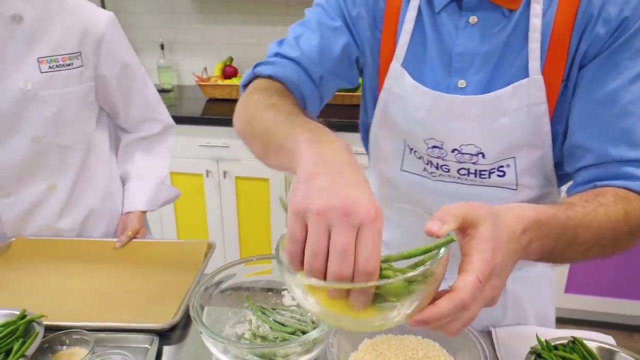 We're going to put our green beans in here and toss it around. Okay, take the fork out Now, toss it. There we go. Whoa, I'm spilling, That's okay. Okay, wow, Look at it. 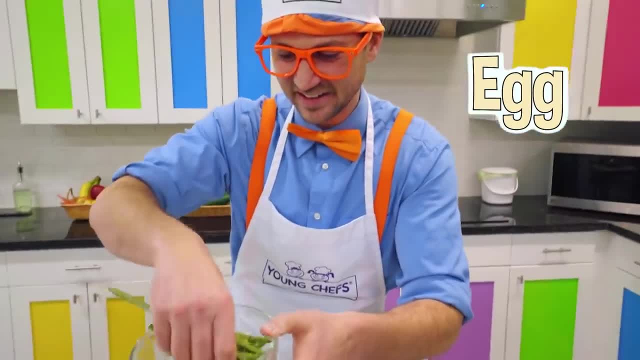 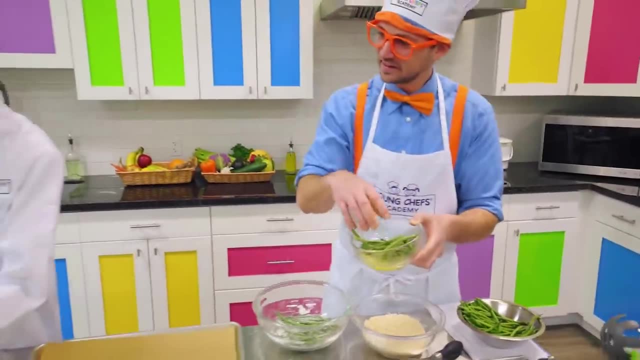 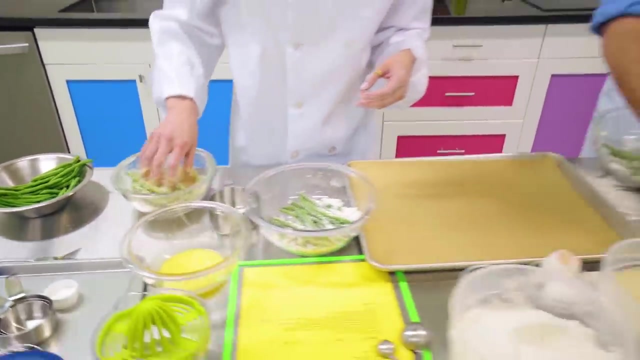 There's so much egg on these green beans. Okay, All right, now you're going to want to put the green beans into the panko and toss them around real quick. Okay, Wow, That looks fun. And once they're nice and evenly coated in panko. 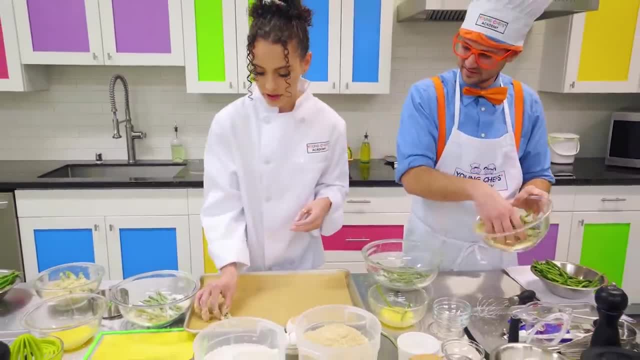 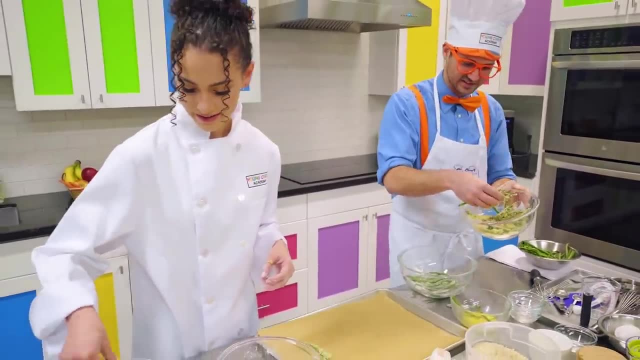 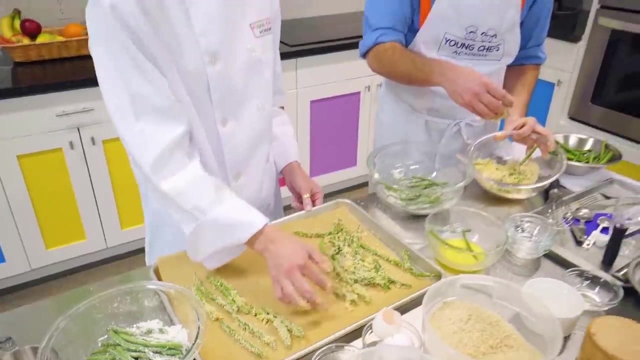 you want to put them onto the tray? Okay, Whoa, These are going to be so yummy. I know I'm excited. Let's put them a little bit nicer so that they're not so messy. Okay, That way they'll cook really evenly when they're spread out on the tray. 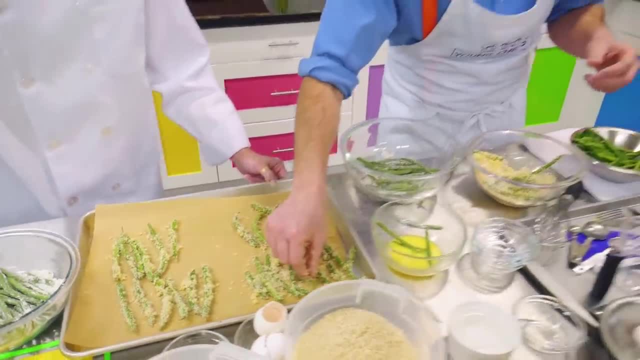 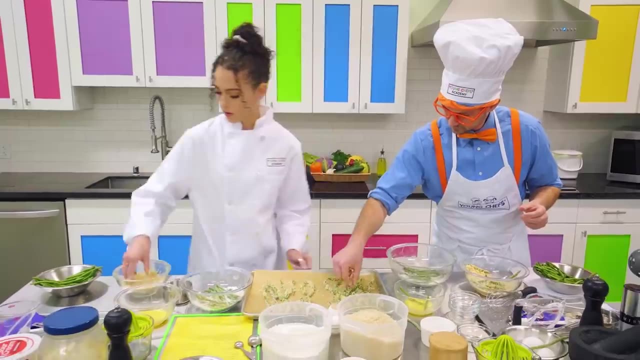 There we go. That makes sense, Oh, I see, because if they're on top of each other, then the heat can't touch the whole green bean. huh, Exactly, You want to make sure that the whole thing is getting cooked. 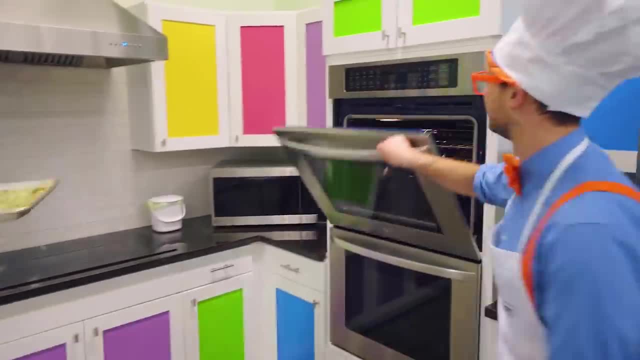 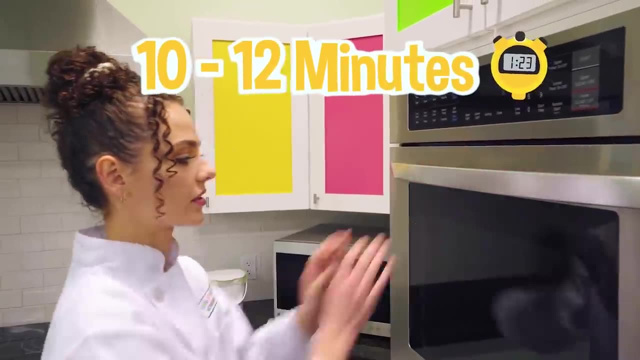 We're ready for the oven. Okay, Here you go. Thank you, Perfect. Those will take about 10 to 12 minutes to cook Whoa. that was really fun making those green beans with you, Wasn't it? Yeah? 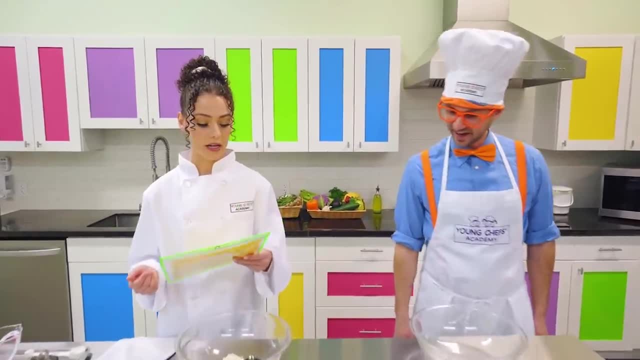 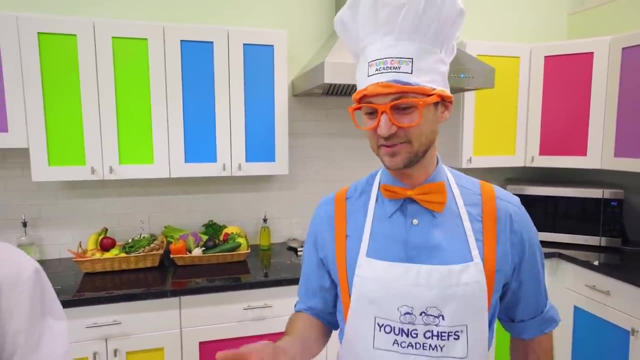 Let's make some ranch to dip them in. What ingredients do we need? We need mayonnaise, sour cream, buttermilk. Oh wait, Did you say buttermilk? Yeah, Oh, I said cream earlier. Okay, so we need buttermilk. 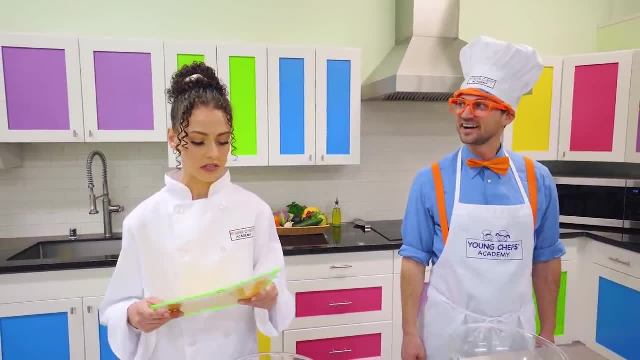 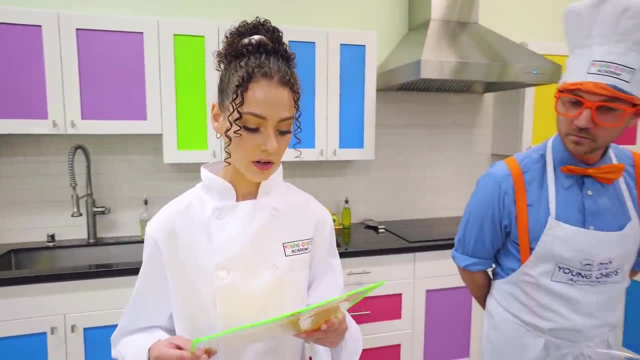 Yeah, They're very similar, but buttermilk smells different and it's a little thicker. Oh, okay, All right. Lemon juice, dill, weed, parsley, chives, onion powder, garlic powder, salt and black pepper. 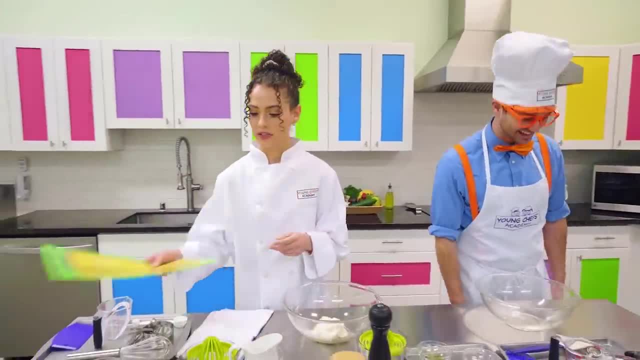 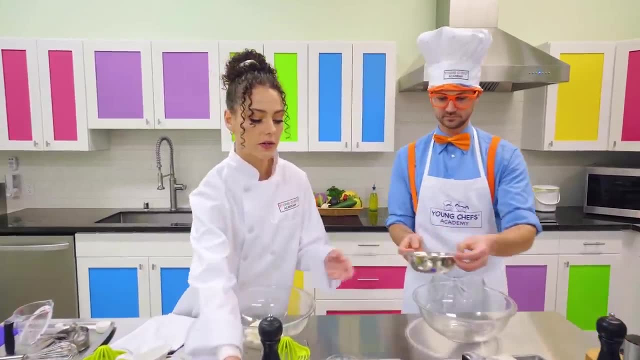 Okay, Perfect, Looks like we have everything I think we do. All right, Next we're going to want to, So I have mine all mixed up. Can you put the mayo and the sour cream into your big bowl? Okay, 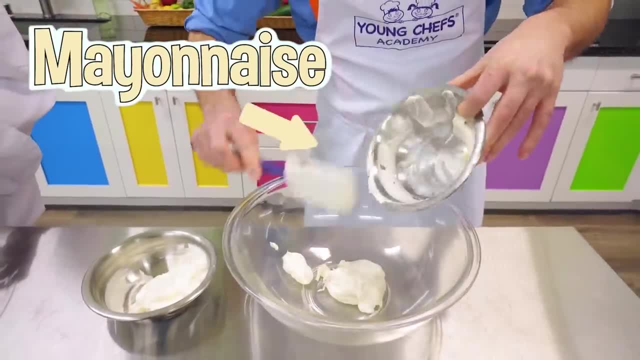 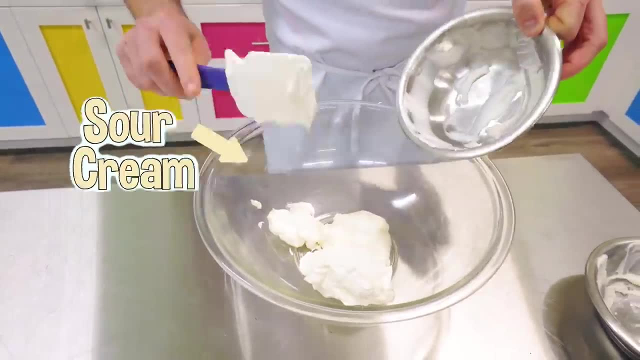 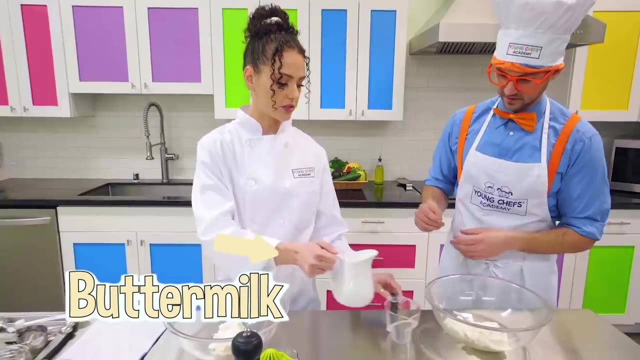 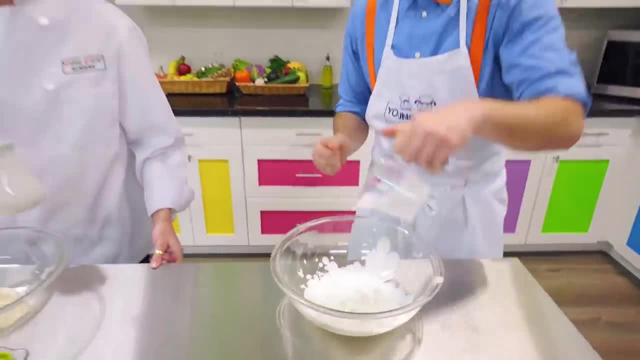 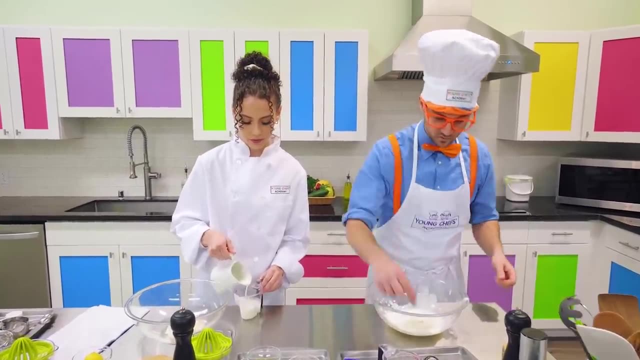 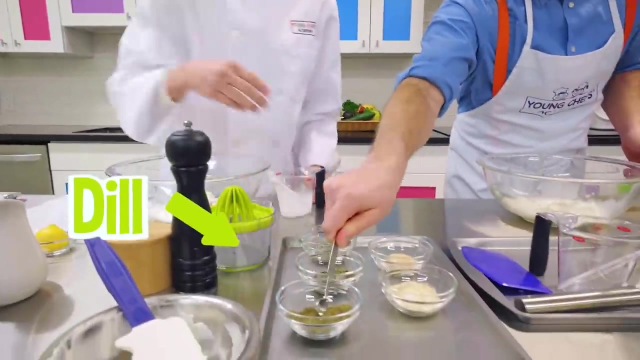 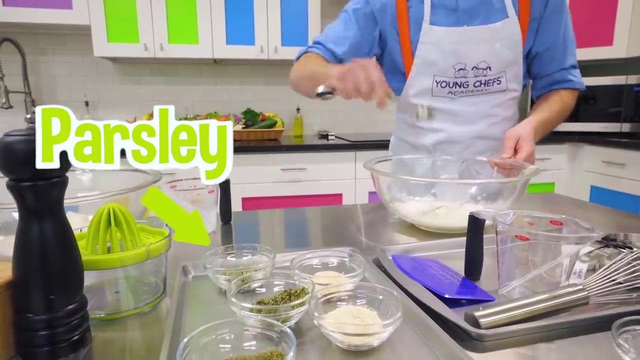 All righty, Here we go. Perfect, All right, Now we're going to want to get our one fourth teaspoon. Okay, Perfect, I'm ready. We're going to use that for, Oh Okay, use that for our dill right here: parsley and our chives Dill, parsley and chives. 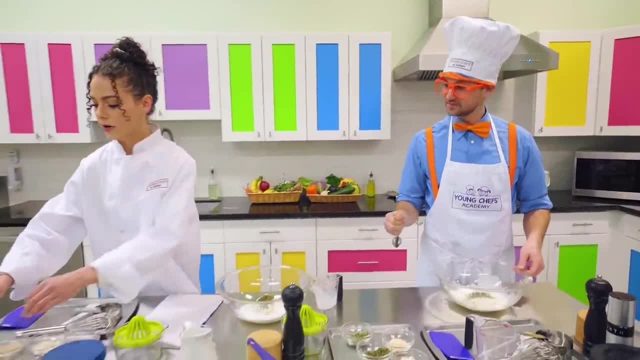 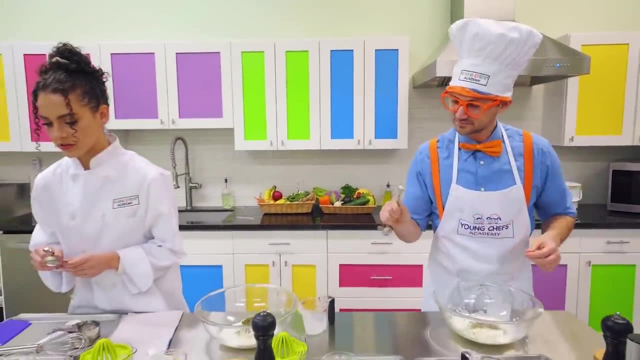 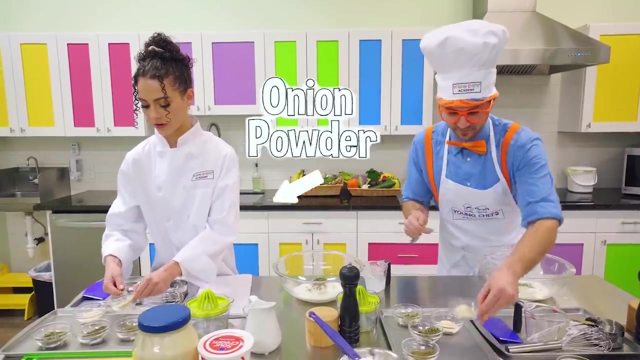 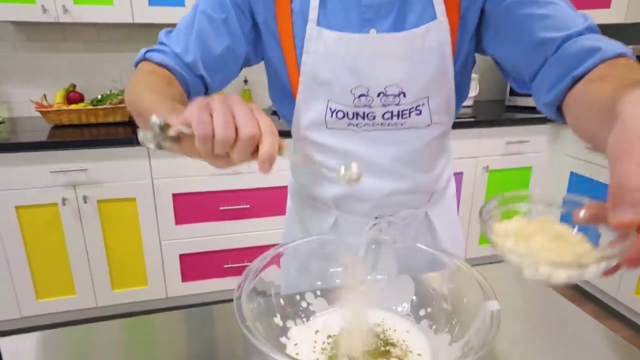 There we go. Good job, puppy. Next, we're going to want our half teaspoon. Okay, a little bigger, All right. All right, and we use that for our garlic powder and our onion powder. Okay, let's give it a little scoop, Okay. and then this one: Perfect. This is going to be so yummy. 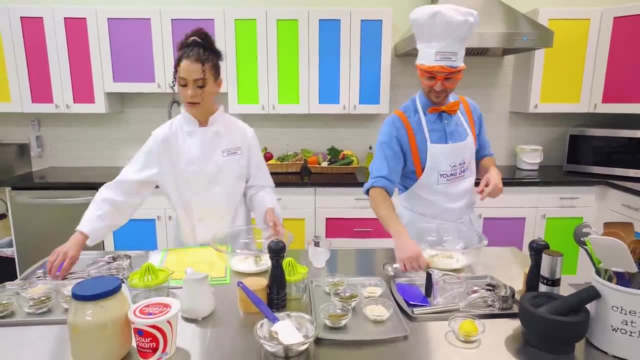 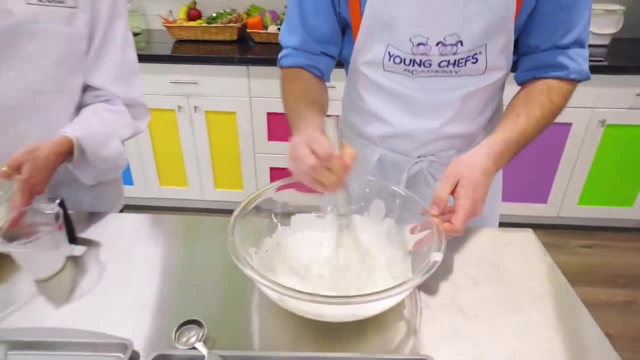 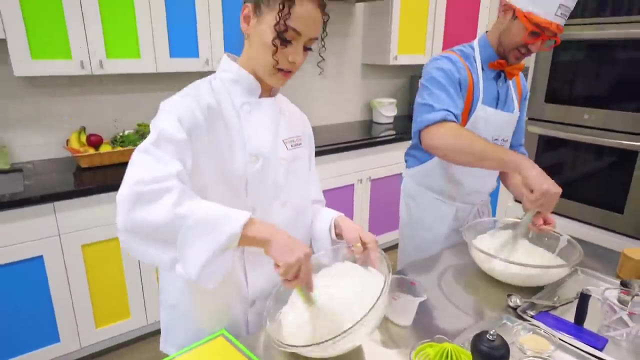 All right, perfect. Let's mix that up with our whisk. Don't forget we whisk with our wrist. All right, Whoa, this smells so good. Once it's all mixed up, we're going to cover it and place it in the fridge to cool. 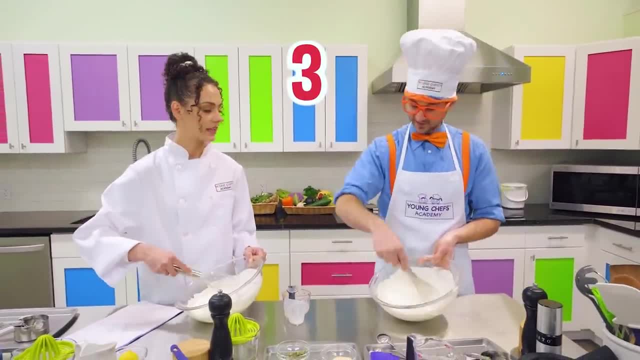 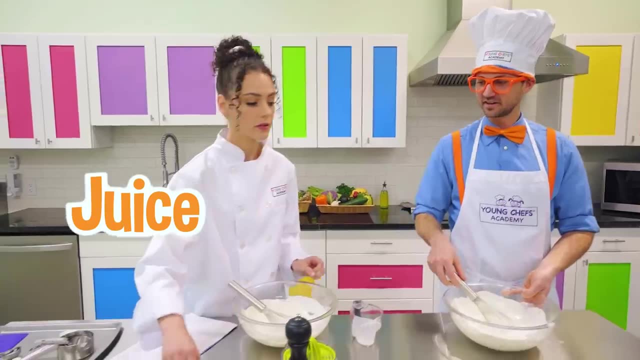 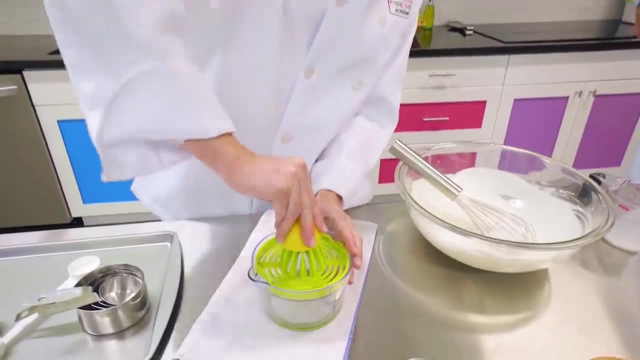 All right, we only have three more ingredients. Okay, what are they? Lemon juice, salt and pepper. Okay, First we want to juice our lemon. Okay, So you have a lemon right up there. Perfect, We have it cut in half and we'll use our juicer here. We want to make sure we squeeze really tight, pushing down and twisting it around to get all of that juice out. 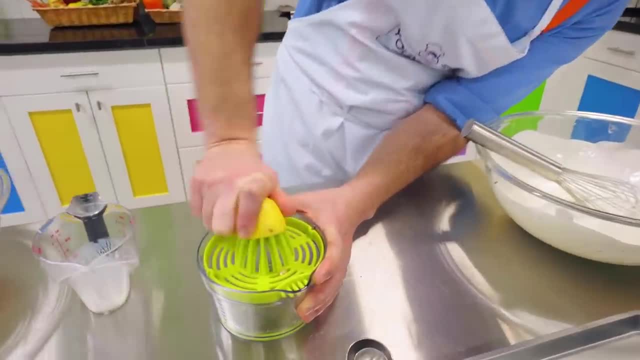 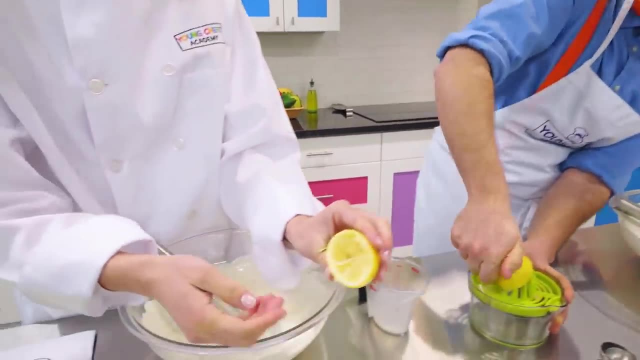 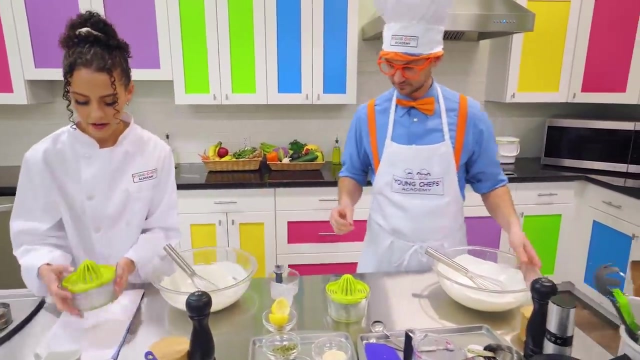 Okay, I guess I'll try it There we go: Good job, Yeah. When you take it off, your lemon should look something like this: Yeah, It's almost empty, Perfect, Good job, Okay. And then we want to pour our lemon juice into our ranch. 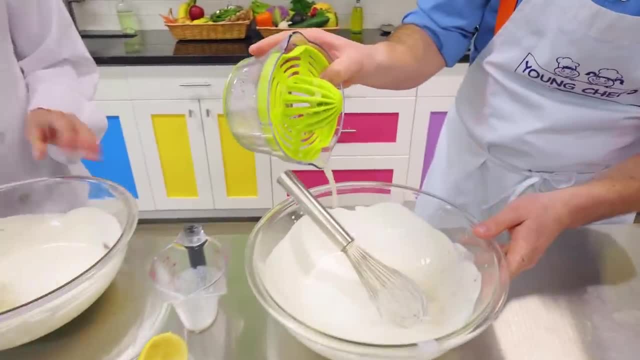 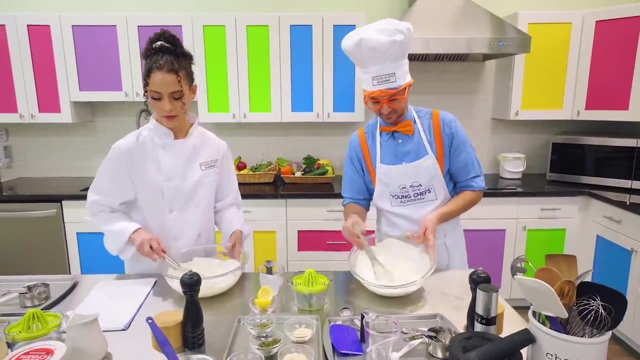 Okay, Here we go. Whee, Awesome, Mix that up. All right, Yum. Now we want to do one-fourth teaspoon of salt Right like this. Okay, Put some salt in there. Okay, All right. 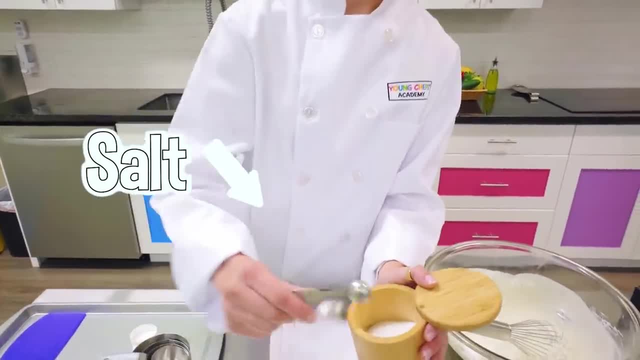 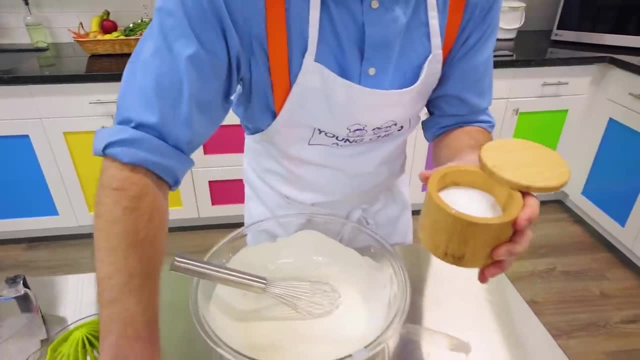 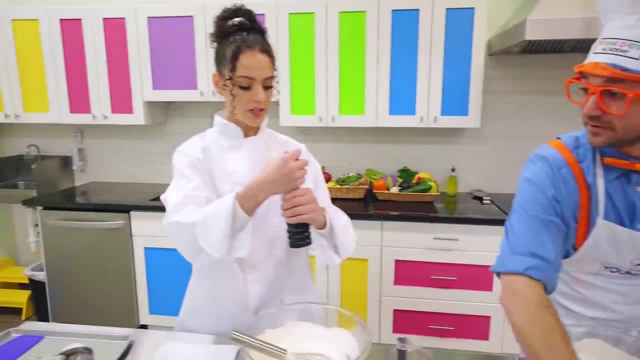 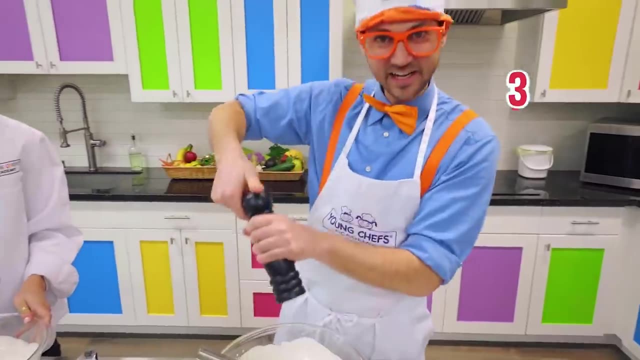 So we'll go about three twists, Okay, One, two, three, Perfect. All right, Let's mix that up. All right, Mix, mix, mix And remember to mix with your wrist. Oh yep, Oh wow. 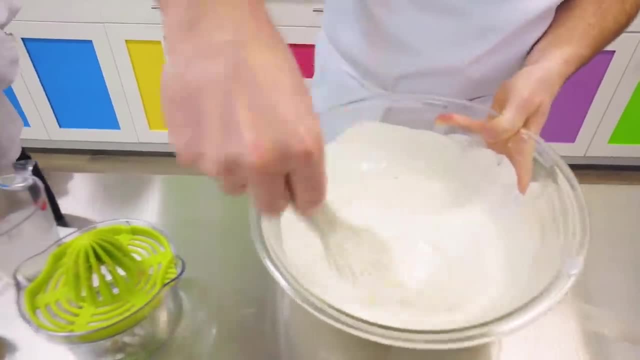 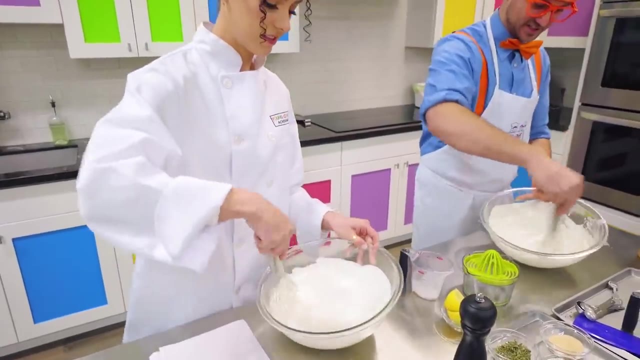 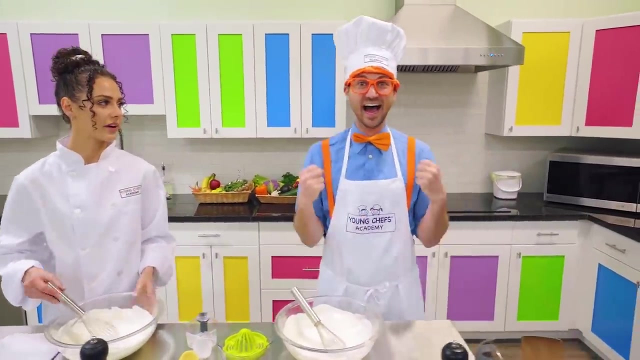 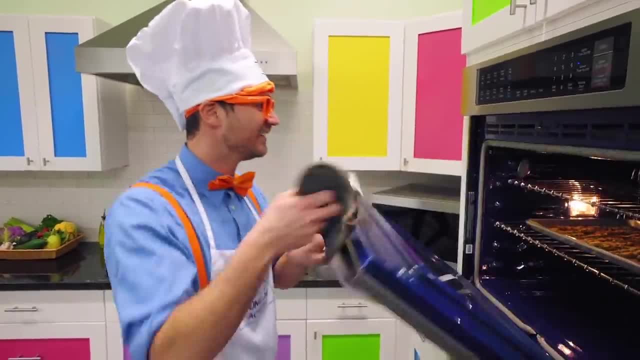 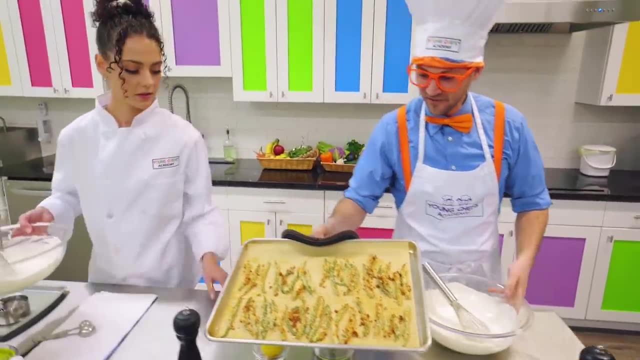 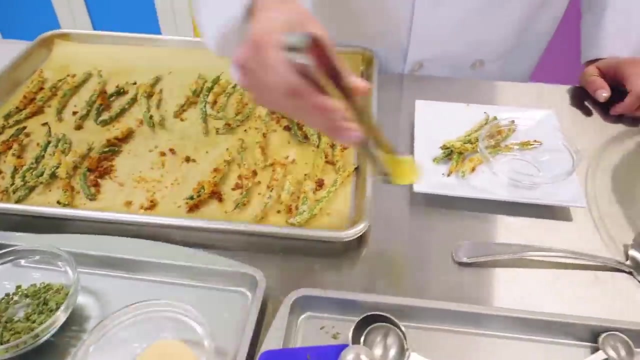 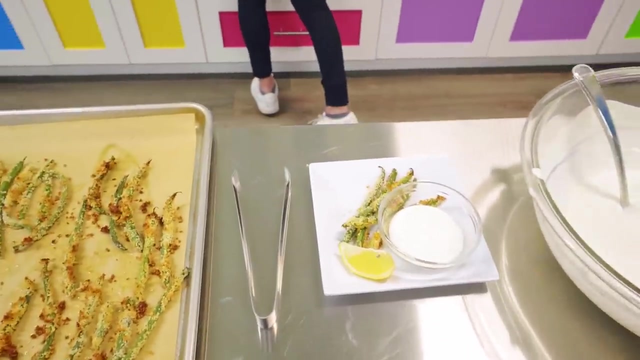 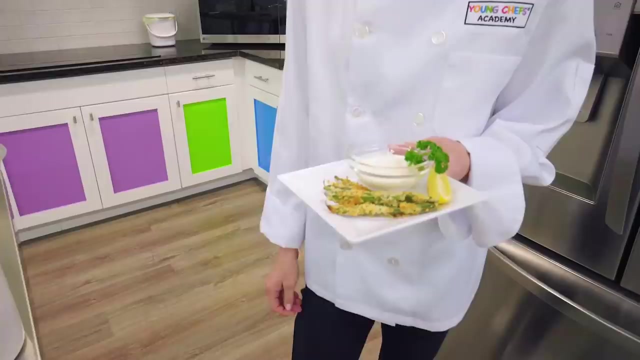 Oh, this is gonna be awesome. Oh, yum, Wow, Those look delicious. Blippi, Whoa, check them out. Oh my gosh, All right, Blippi. it looks like our green beans and zesty ranch are all ready. 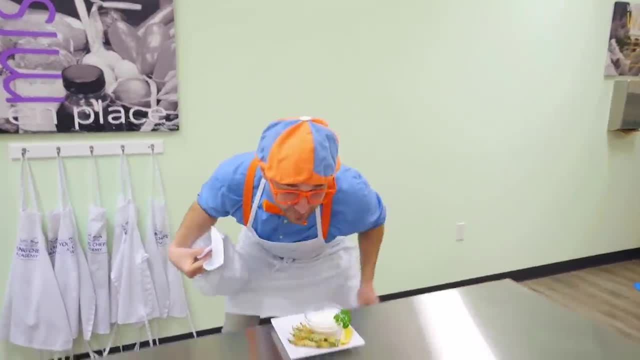 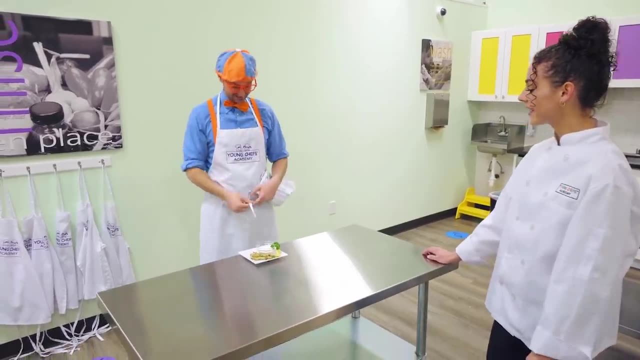 Oh, those look yummy. Check them out. Whoa, I am so excited. Thank you so much for teaching us how to make these. Of course, you did such a good job. Come back next time. Oh well, thank you, See you later. 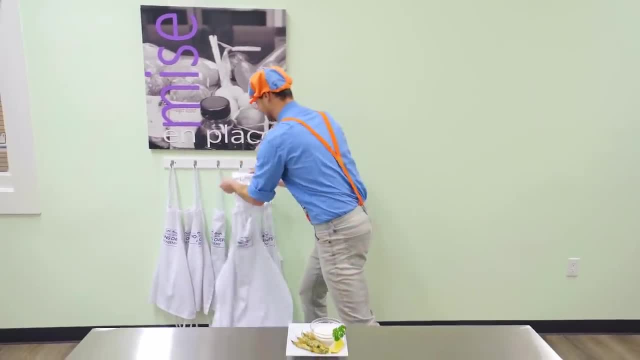 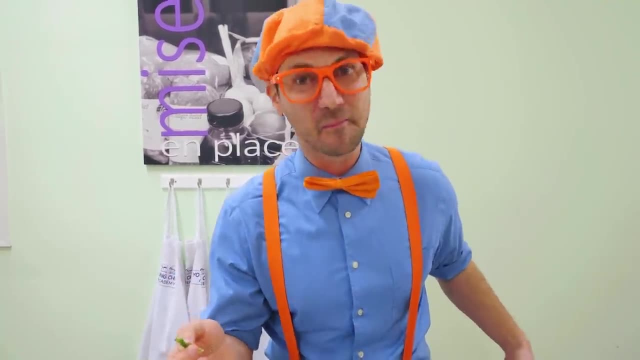 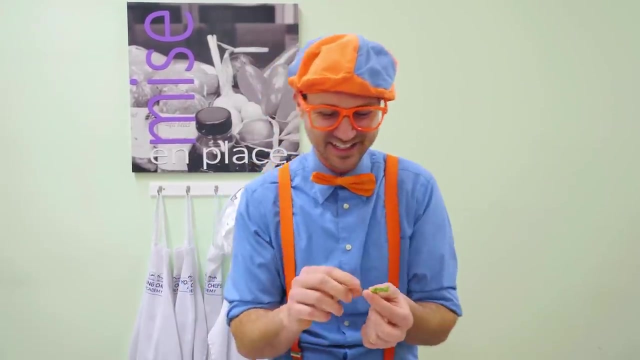 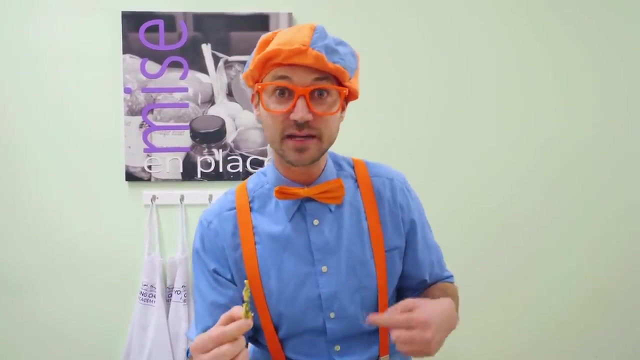 See ya. Wow, I am so excited. Here we go. Yum, that is dippalicious. So silly, Yeah, you'd think, because they're green, they're not good. But hey, trust me, it's really fun to try new types of food. 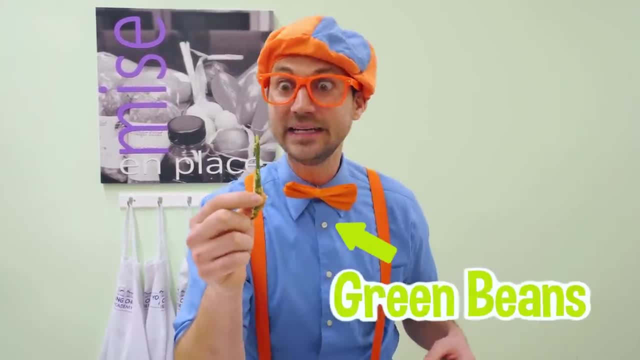 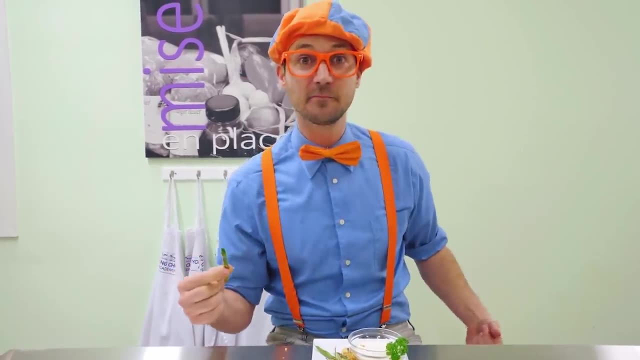 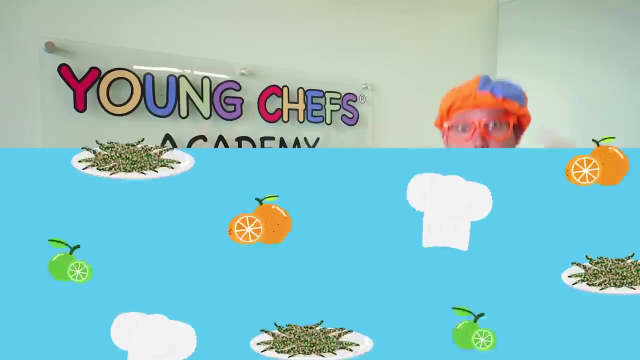 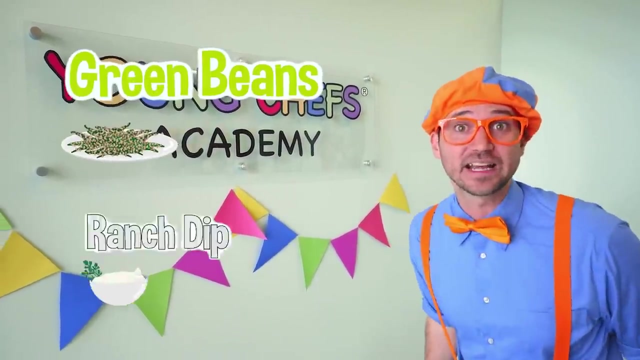 Yeah, like these yummy green beans that we made. Yeah, Mmm Yum. Even healthy foods can be really yummy. Good job cooking, Oh yee-haw, Wasn't that fun making those green beans and that ranch dipping sauce. 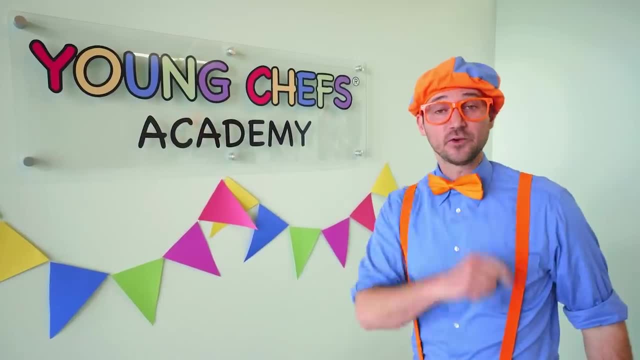 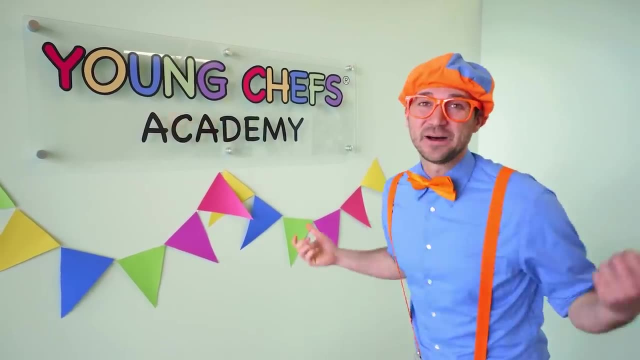 Yum, It was so tasty. Hey, if you want to check out the exact recipe, you can go to Young Chefs Academy website and check out their blog. Woohoo, Well, this is the end of this video, But if you want to watch more of my videos, all you have to do is search for my name.